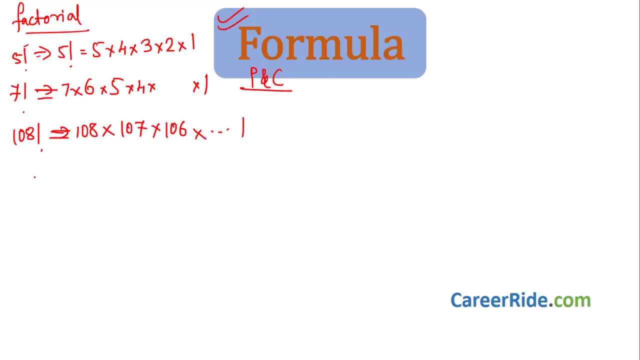 minus 1, 106 up to 1.. So if there is a number n and if we express it as n factorial or if we write n factorial, then its value will be n multiplied by n minus 1, multiplied by n minus 2 up to 1.. This is the concept of factorial. Now let us move to another concept. 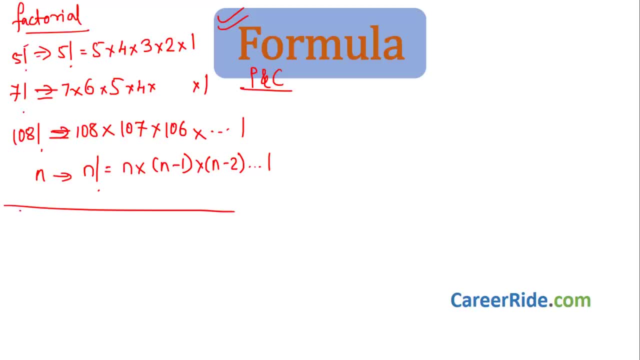 which is related to factorial and which is also related to permutation and combination. If say you have, say, 7 things, if you have 7 things and if you want to let us see, these are the things: 1, 2., 3,, 4,, 5,, 6 and 7.. And if you want to arrange the 7 things in one line, in a single line, 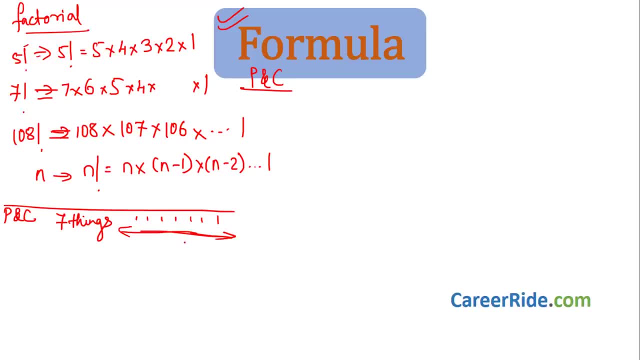 you want to arrange these 7 things. So in how many possible ways can you arrange these 7 things? Very easy. When you want to arrange these things into single line, you can arrange them in 7 factorial ways. So if you have 10 things and if you want to arrange these, 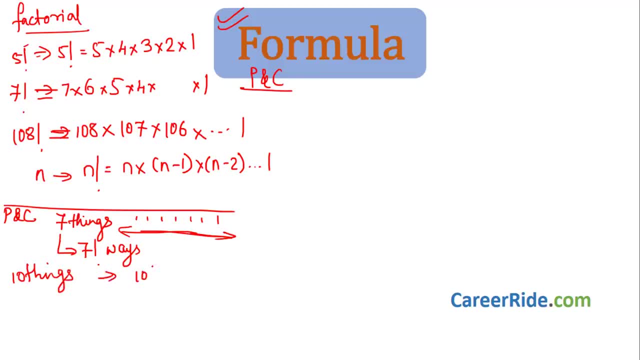 10 things in a single line. you can arrange them in 10 factorial ways. okay, also this is like arranging in a single line. so we have, for seven things we have seven factorial. for ten things, we have ten factorial ways. so for n things you will have n factorial. 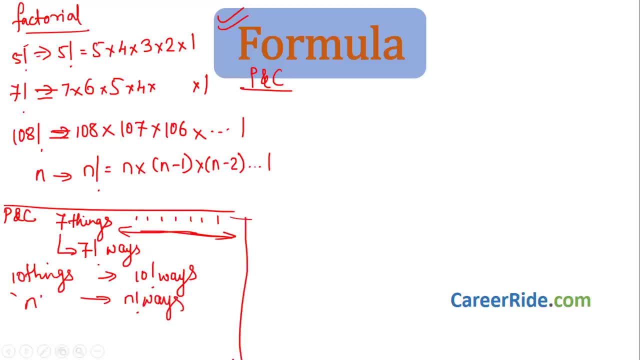 ways. now, instead of a single line we want to arrange it in a circular pattern or in a circle. so that means we have to arrange the seven things- one, two, three, four, five, six and seven- in a circle. we have seven things. if you want to arrange these seven things in a circle, then we can arrange them. 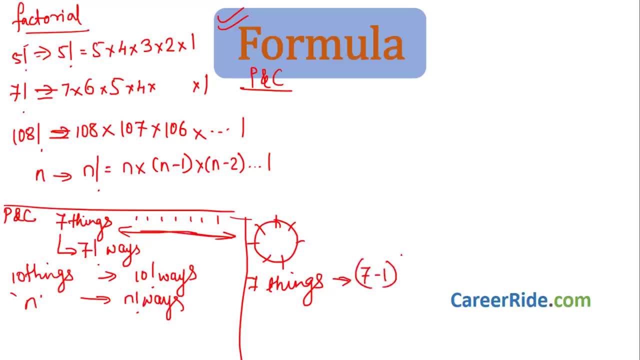 in simply seven minus one factorial ways. that is nothing but six factorial ways. seven minus one is six, six factorial ways. if you have ten things and you want to arrange these ten things in a circle, you will arrange it in ten minus one, nine factorial ways. so we can say: if we have n 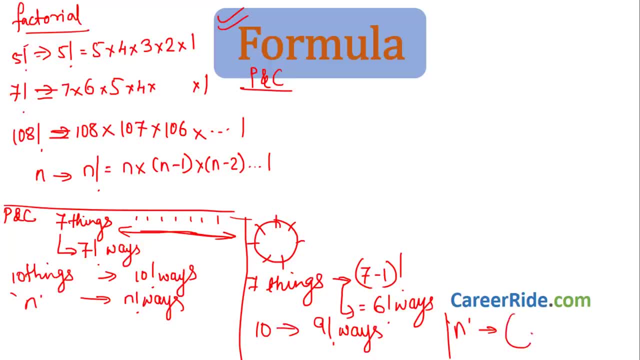 things. we can arrange these n things in a circle in n minus 1 factorial ways. See how easy it was, just remember. factorial means what? if we express any number as factorial, we can write it that number minus 1 multiplied by minus 1 multiplied by number minus 2, and so on. So 5 factorial is 5 into 4. 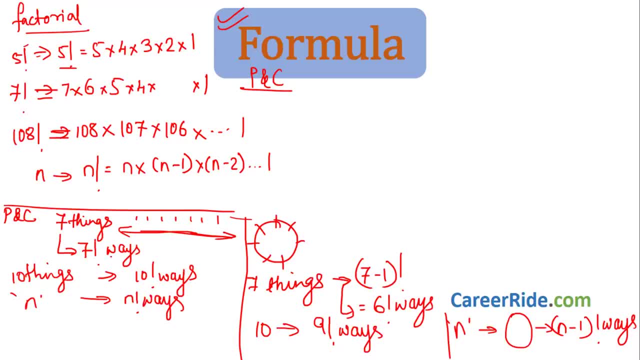 into 3, into 2, into 1, up till 1, we have to go Again. if there are n number of things and we want to arrange it in a straight line, arrange them in a straight line. we can arrange them in n factorial ways. If we have n things and we have to arrange them in a circle, we have to arrange. 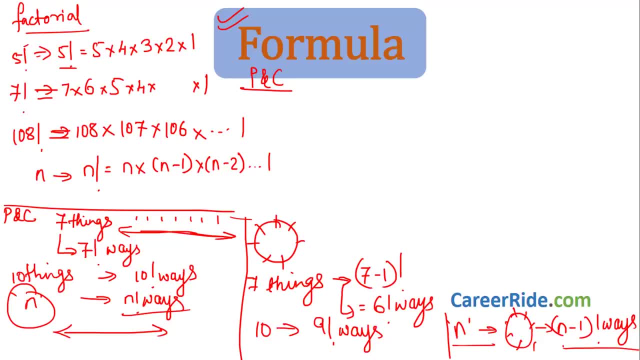 them. we can arrange them in n minus 1 factorial ways. Now, these are some basic things that you needed to know. Now let us move on to the formula related to permutation and combination. We have permutation and we have combination. c comes before p. 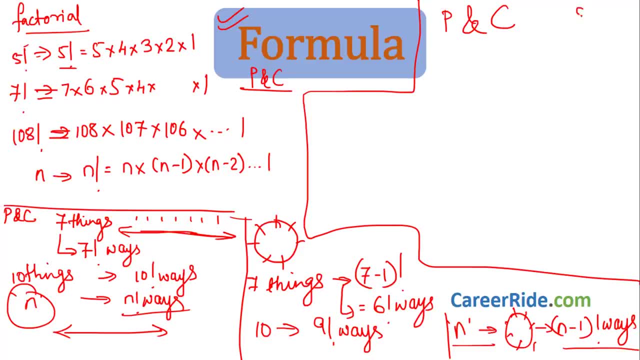 Now there are two concepts over here. first is to select right. first is to select, and what is second? second is to select, right for select and arrange. So there are two concepts that you need to understand. there are two things when we talk about permutation and combination. the first is: 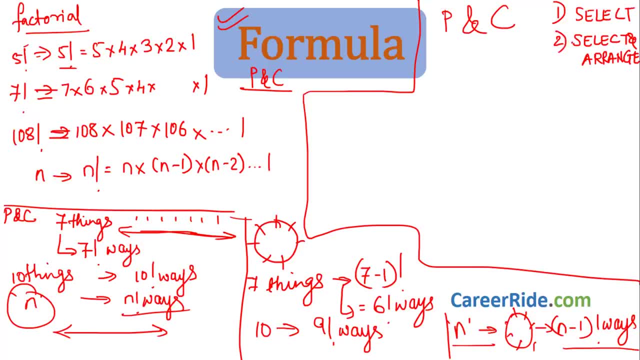 just select. second is select and arrange. okay. Now, select has c into it. So select must be related to combination right, c, c. So combination means to just select. okay, combination means to just select. always remember this. combination means to just select. So 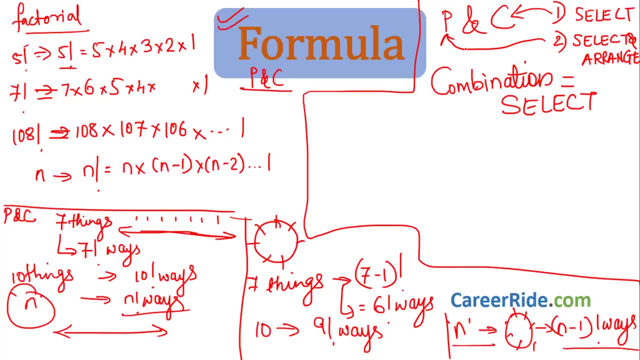 select and arrange means what? select and arrange means permutation. right, but obvious. if there are two concepts, permutation and combination, and we have two things: select and select and arrange. So select is combination, then select and arrange will be permutation. correct combination is select only, select, just select. right. Now combination is expressed as: let us see how to do that, say you. 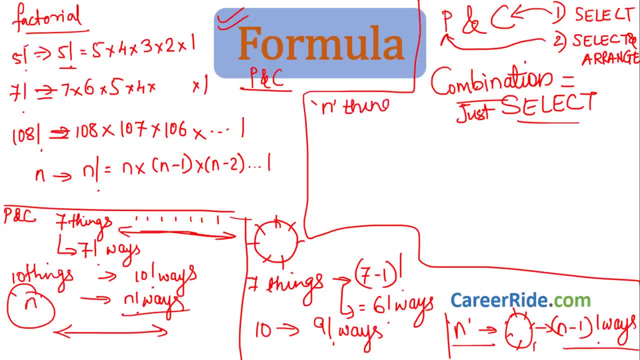 have n things. okay, you have n things in a box. out of that, you want to select r things. you have a box, right, you have a box over here and you have n things in this box. So out of that you want to select are things. so what do we have over? 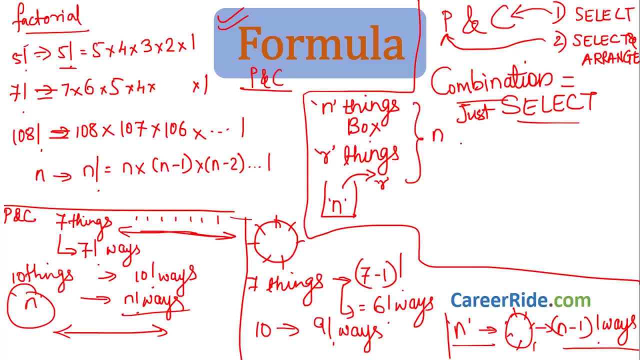 here we have n things, okay. Out of that we have to select. are things. what is select? select means combination. combination starts with c, So n c are means we have n things and we have to select. are things out of those n okay? 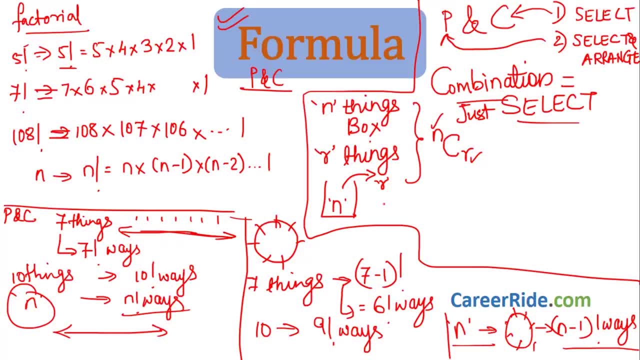 Now are: can be less than n, also equal to n also. for example, you may have five things in this box and you may want to select one thing or n. also many things, all right, Now- are less than and also equal to also. for example, you may have five things in this box And. 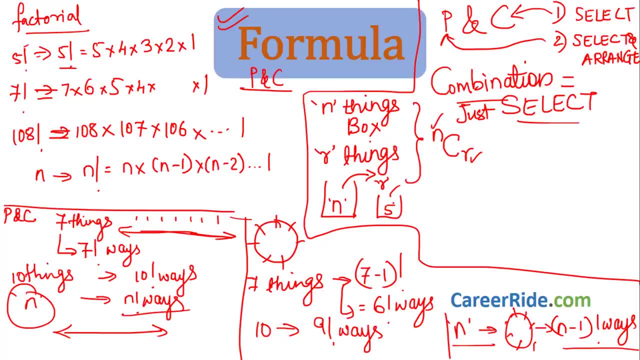 you may want to select one thing also out of that, but what you want to do is go to n Wrestle months may want to select one thing or two thing or anything like that, or you may want to select all the five things. So NCR means is the formula for combination. NCR is formula for combination. 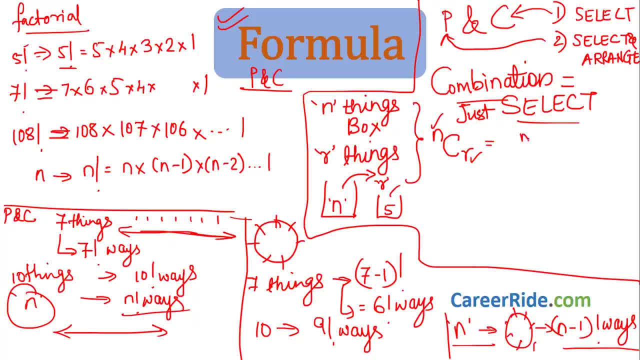 and how. what is the formula? We have N, So write N factorial. We have R, So write R factorial. and there is another term which is nothing but N is greater than R, So N minus R factorial. This is the formula for combination. See, very easy to remember: NCR, Whenever we have N things. 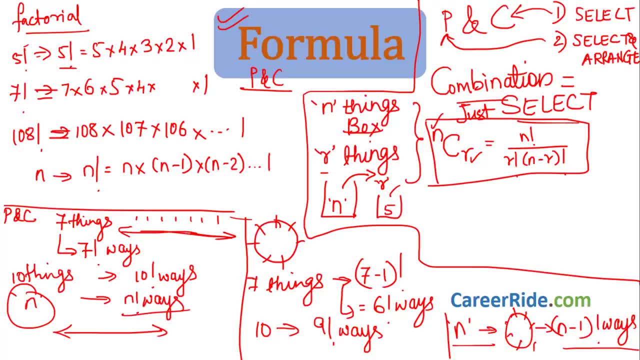 in a box. we want out of that. if we want to select R things, then what will be the formula? It would be: N things in a box, We want to select R things. Select means combination, So we will write C over here. NCR is nothing, but we have N, So N factorial divided by we have R, So 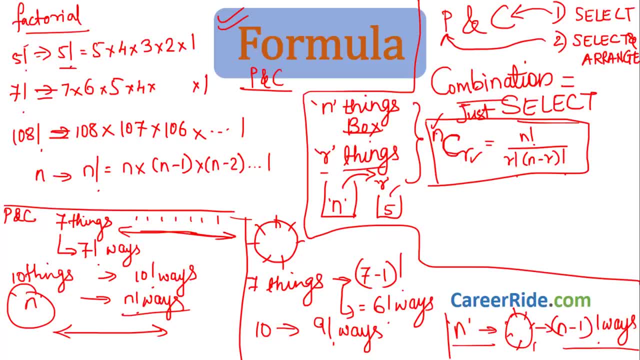 R factorial, and again another term below, that is N minus R, because N is greater, It is C, for X is greater than R. This is the formula for selection or combination. Then what will be the formula for permutation? Permutation starts with what P. We have N. 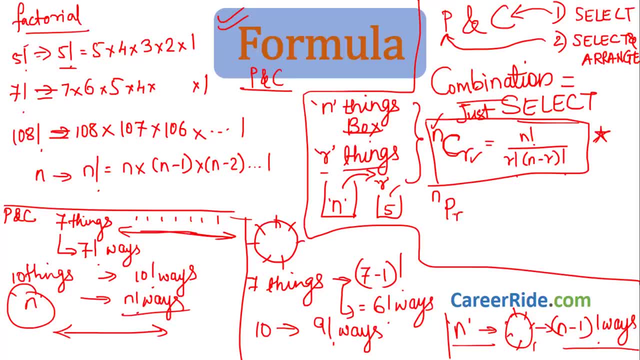 things. We have to first select R things and then arrange them. What is the formula for selection N factorial upon R factorial into N minus R factorial? and we already know that if we have N minus R factorial by N plus R factorial, we are product of theX and our 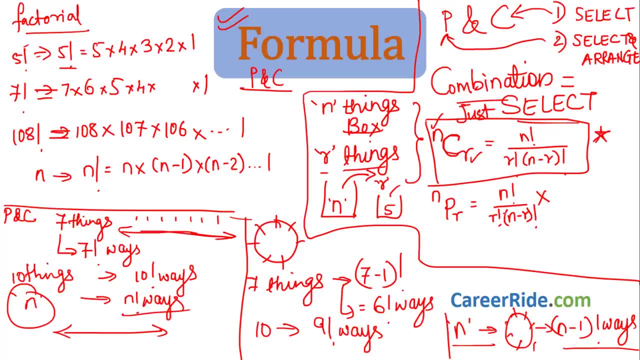 idea is we have X before x and those X before x before x τι, And we already know that if we have X, if we have say r things and we want to arrange r things, if we want to arrange n things, we can do. 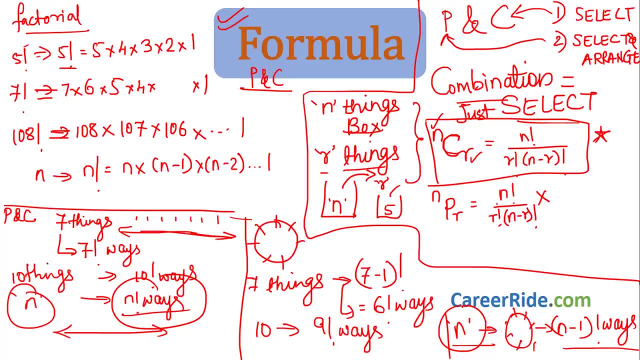 it in n factorial ways. Same way over here. if we are selecting r things and arranging these r things that can be arranged in r factorial ways, So r factorial, r factorial gets cancelled. What do we get? n factorial upon n minus r factorial. So this is the formula for: 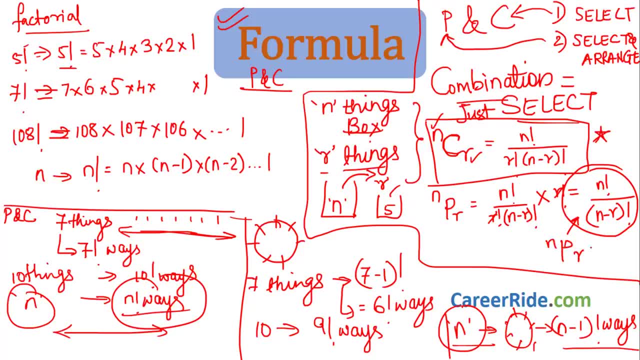 permutation, npr. See, you just need to remember formula for combination, and we know combination is select, permutation is select and arrange. So take select, multiply it by arrange. Arrange is nothing but arranging r number of things, that is r factorial, So r gets cancelled. 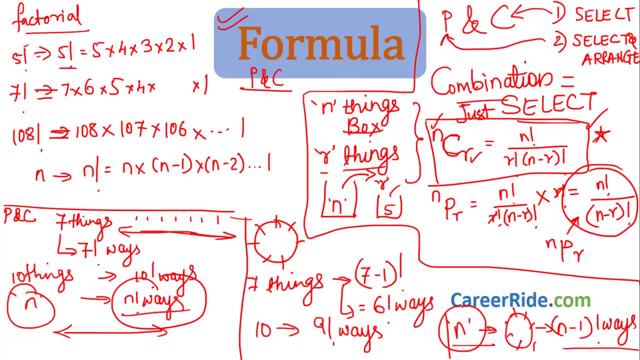 and you get the formula. So there is no need to remember two formulas. You can derive permutation formula right from combination formula. Just remember: combination is select, permutation, Permutation is select and arrange Very easy. Using these formulas we can solve all the 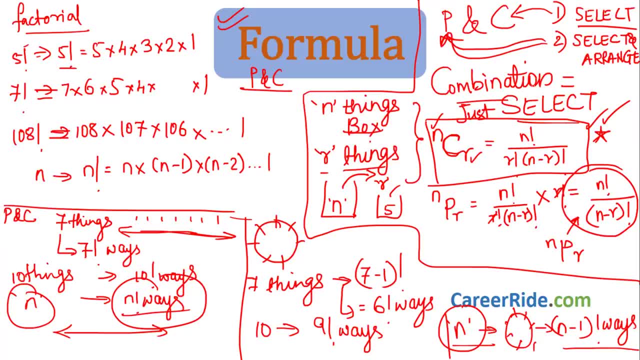 sums related to permutation and combination. Again, before going to the sums related to permutation and combination, I would like to tell you one small thing. Now. what have we learnt? We have seen the formula for permutation combination and we will use it to solve the. 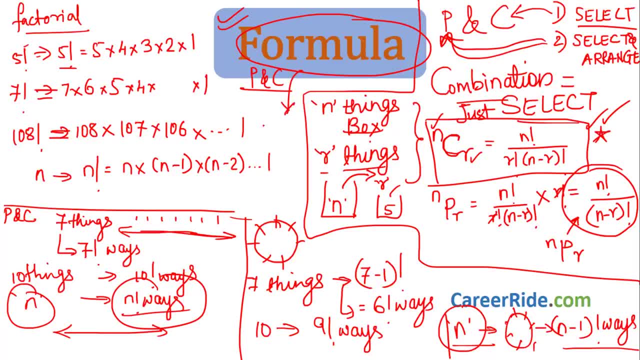 sums. However, some of the sums can be solved by simple logic. also. We are going to see how do we solve sums related to permutation and combination by simple logic also. Not always we will need the permutation and combination formulas. Most of the time we will try to. 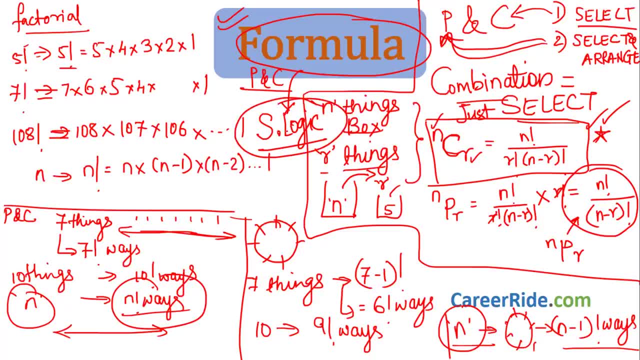 use the formula, but we can also solve most of the sums by simple logic. Why do we need to learn how to solve by simple logic? Because in exam sometimes, if you do not remember the formula, we can try to solve the sum by this simple logic or common sense. So we will. 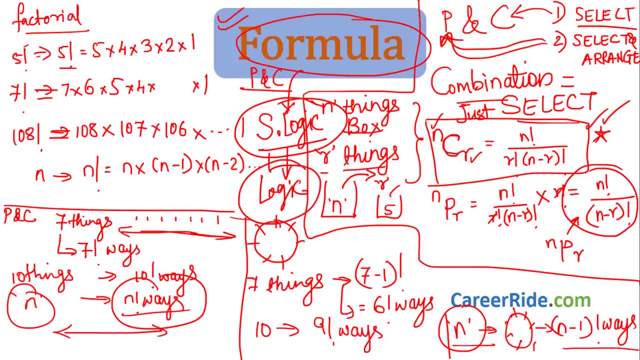 try to see both the ways. We will try to develop both the ways. So these are the two ways of solving the sum. Now, what are you going to do? What are you going to do? Maybe you both the ways. it is much better to have two weapons in our hand while going for. 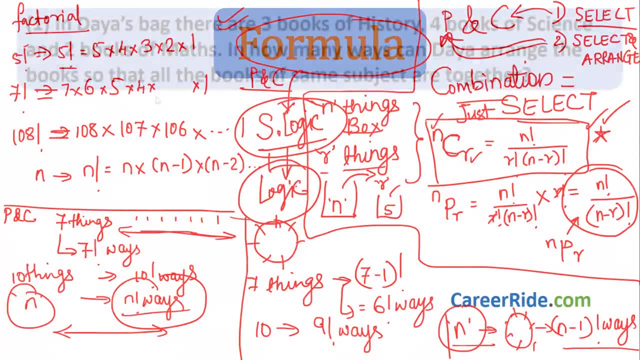 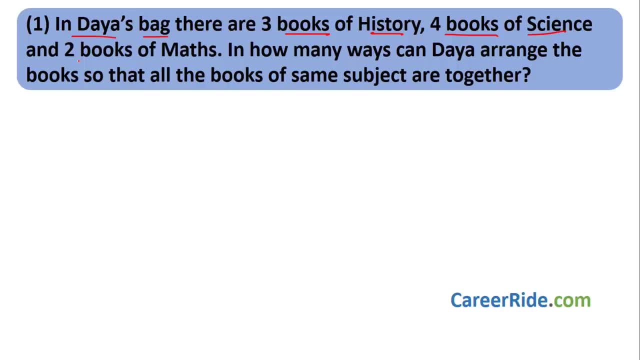 exam. okay, so let's move on to question number one. in Daya's bag there are three books of history, four books of science and two books of maths. in how many ways can they arrange in the books so that all the books of same subject are together? now let us see how to solve this sum over here. do we see the word? 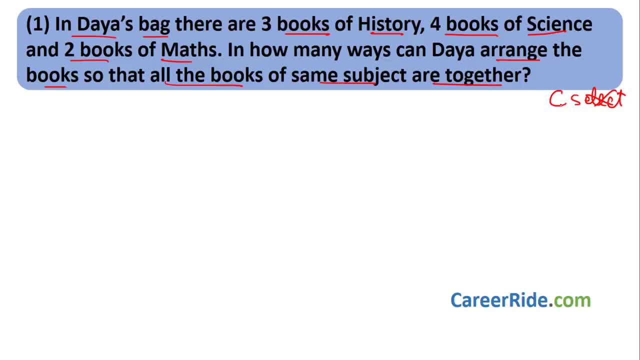 select no, so combination would not be a part of it. but we see the word arranged, so permutation can be a part of this. but this is not select and arrange, it is only arranged. so instead of using permutation formula, let us use the normal factorial. we know that if we have n things, we can arrange them in n. 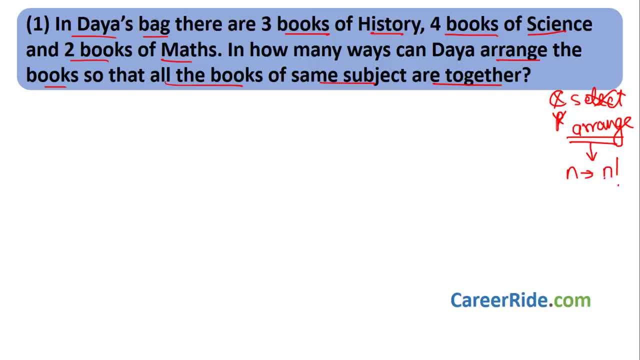 factorial ways, correct. so let us see how to solve this sum using simple logic. now what are they saying? there are three type of books. there are three books of history, there are four books of science and there are two books of maths- correct. now what they want is that Daya should arrange the books so that all the books 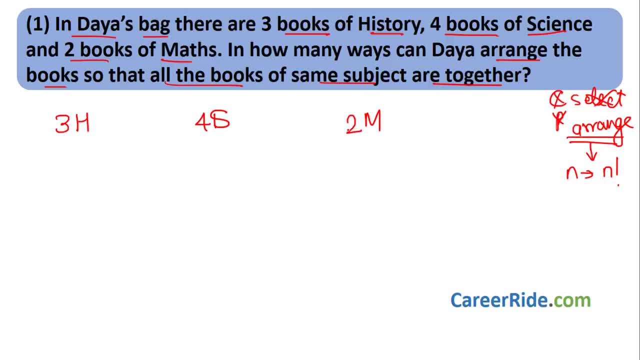 of same subject are together. now how to achieve this, that all the books of same subject remain together. if we add all the books, what do we get? four plus three, seven plus nine, there are total nine books. and if we try to arrange these nine books, we'll arrange them in nine factorial ways. but what will happen is: 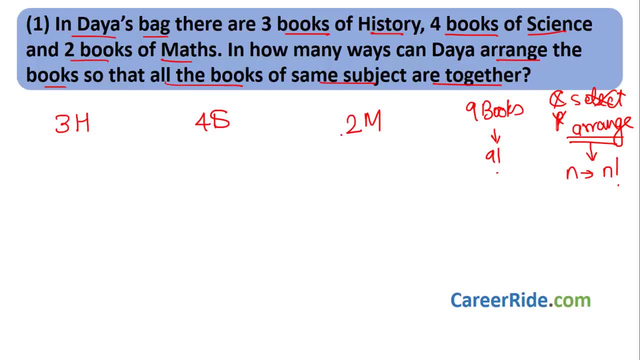 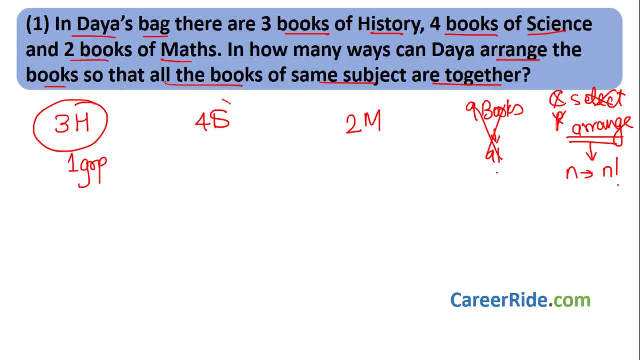 entire group. okay, consider this as a second group, consider this as the third group. now, instead of having nine separate books, we are just having three books or three groups. okay, these three groups can be arranged in how many ways? simple, three factorial ways. so, whenever you are arranging the groups, okay, what will happen? you can arrange them as one, two and three, or you. 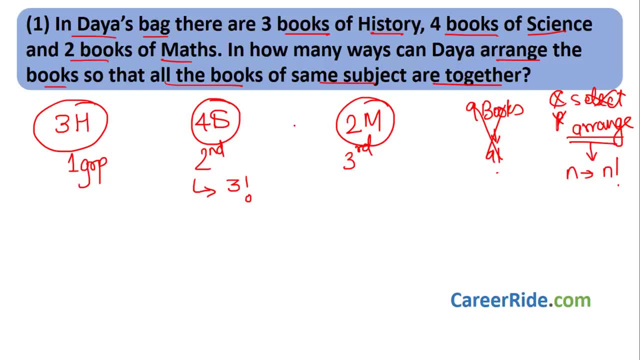 can arrange them as one, three and two, so entire group moves. individual books don't move, so the entire group moves. so we are keeping all the books of same subject together. okay, three groups can be arranged in three factorial ways. now, in each group there are- there is not just one book in each group. 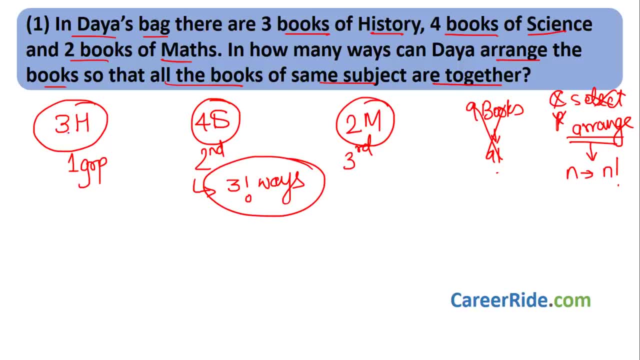 there are more books, multiple books, in one group, that is the first group of history, there are three books, right, three books of history. these three books of history can be arranged within themselves. this is one, this is two, this is three and this is the entire group. okay, in the entire group of. 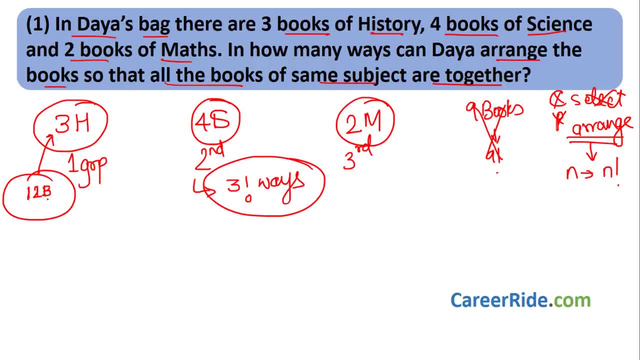 history. we have the first book, we have the second book, we have the third book. it can also be arranged as in the entire group: first book, third book, second book. it can also be arranged as third book, first book, second group. okay, so there are various ways to arrange also within the group. 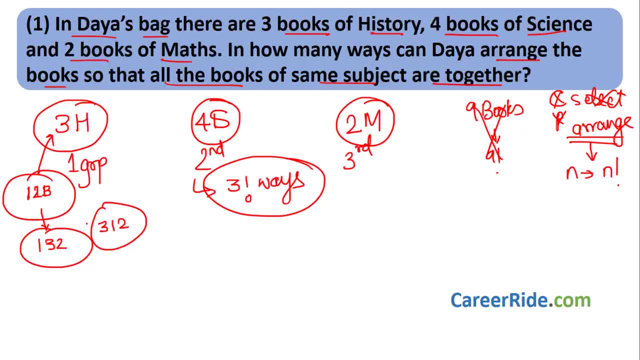 okay, so there are various ways to arrange also within the group. okay, so there are various ways. right, so in the group there are three books, so how many? in how many ways these three books can be arranged within themselves. for the history group there are three books, so these can be. 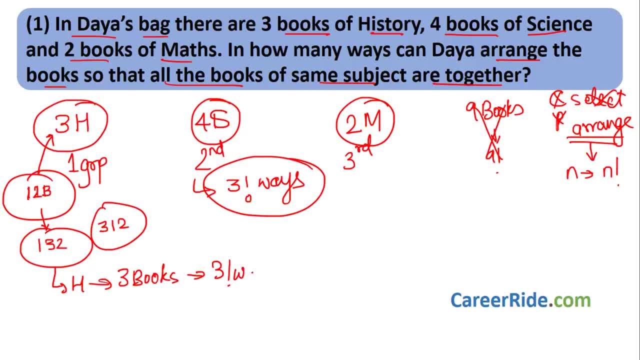 arranged in simply three factorial ways. for the science group, there are four books of science which can be arranged in four factorial ways. for the maths group, there are two big books within maths group which can be arranged within them in how many ways? two factorial ways. so how many are? 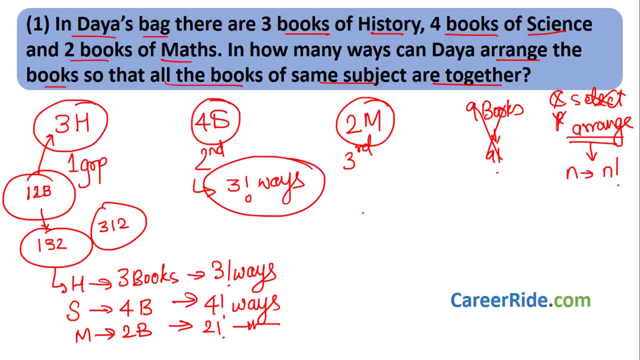 the total ways in which all the books can be arranged. that would be three factorial, okay, multiplied by history book arrangement, science book arrangement, maths book arrangement. three factorial is what? three into two into 1, multiplied by again 3. factorial 3 into 2 into 1, multiplied by 4. factorial 4 into 3 into 2, into. 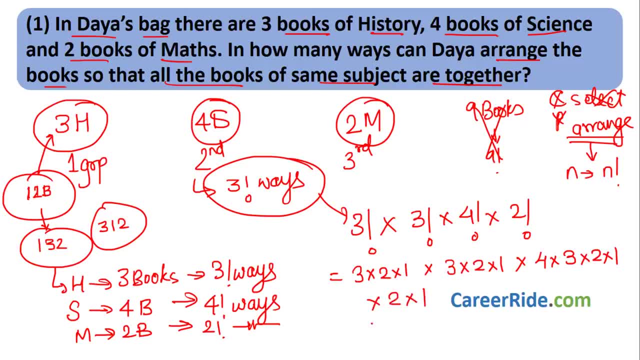 1 multiplied by 2 factorial 2 into 1. What do we get? 3, twos are 6.. 3, twos are 6.. 4, threes are 12.. 12, twos are 24 into 2.. That would give us 1,, 7,, 2, 8 ways. So in 1,, 7,, 2, 8 ways books can be. 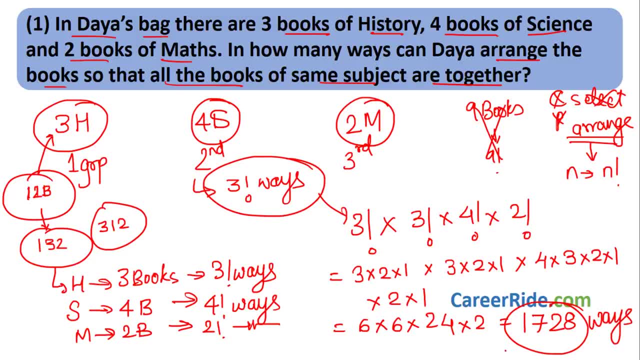 arranged so that all the books of same subject are together. See how easy it was. You just need to remember. n books can be arranged in n factorial ways, And when we make groups, the groups remain together. When we make groups, whatever material is there within the groups, that will always. 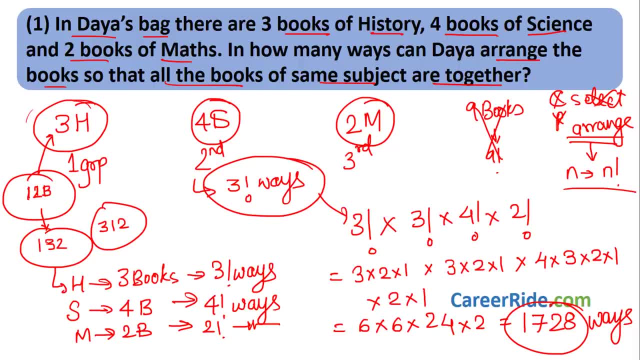 remain together And within a group also, we can make arrangements, We can separate. For example, these three books are 1,, 2, 3.. And these are the other two groups. Now this 1,, 2, 3 can be written. as n books. So these are the other two groups. Now this 1,, 2, 3 can be written as n books, So we can arrange it as 1,, 3, 2. also We can arrange it as first book, third book and second book. 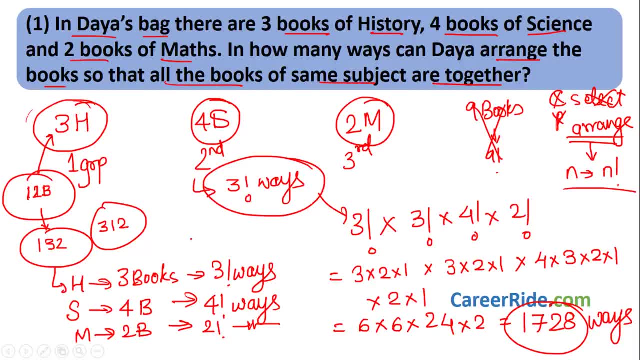 of history Again we will have this same And we can keep on changing. So within group also there is arrangement And between the groups also there is arrangement. So we have to consider both these things Again when we solve more and more sums. it would become very much clearer to 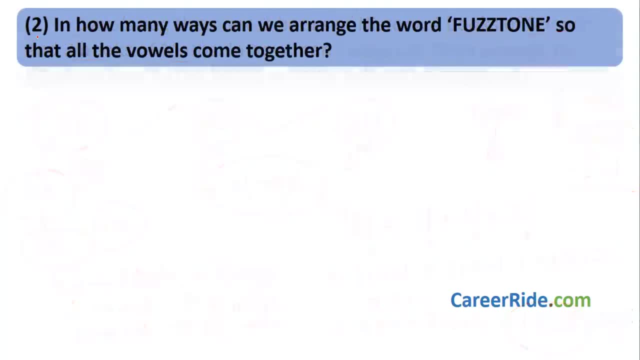 you Now moving to question number 2.. In how many ways can we arrange the word fuzz tone so that all the vowels come together? Again, we have the word arrange over here. Arrange is related to factorial, That is n factorial. There is no select. There is no select, and arrange Only. 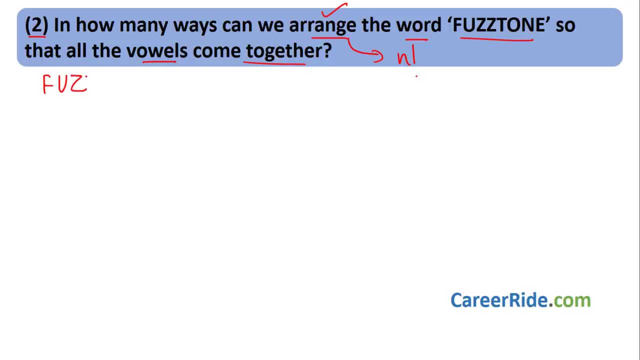 arrange, is there? What is the word? they have given Fuzz tone. Now they want that all the vowels come together. We have to arrange it in such a way that in how many ways we can arrange that all the vowels always come together? What are the vowels U, O and E? These are nothing but the 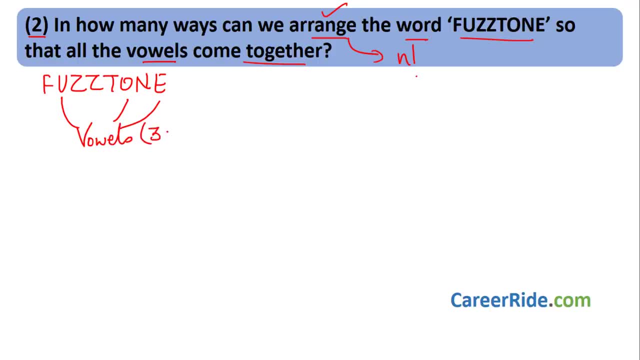 vowels. That means there are 3 vowels. How many total words are there? There are total 8 words. Out of that, 3 are vowels. So how many left? 5 alphabets left? There are actually 8 alphabets, So 5. 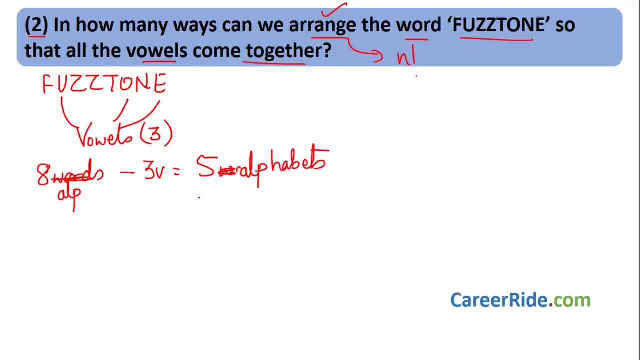 alphabets are left. Now what are the 5 alphabets? F, Z, Z, T, N. Now these 3 vowels have to be together compulsorily, So consider this as one group, Just like we saw. 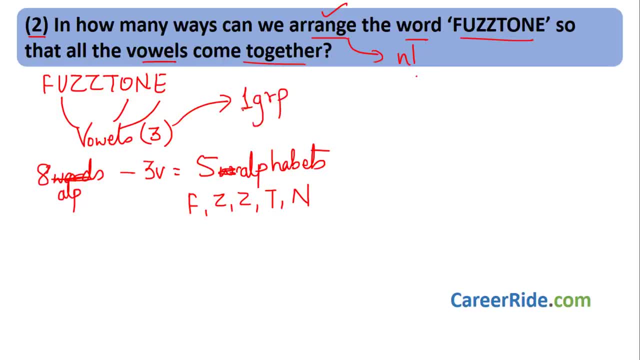 in the last term. we want history books to be together, maths to be together, science to be together. So we consider everything as a single separate group. So these 3 vowels always have to be together, always should come together. So consider the vowels as a single group. Now 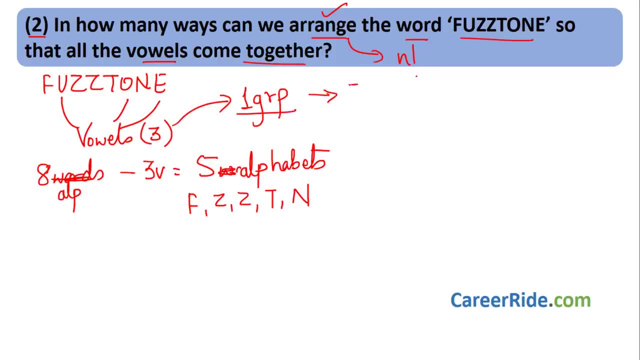 these vowels can be arranged within themselves in how many ways? 3 factorial ways. Why We have seen that history books? there are 3 history books and within themselves, within the 3 history books, the 3 history books can be arranged in 3 factorial ways. Same way, these 3 vowels within. 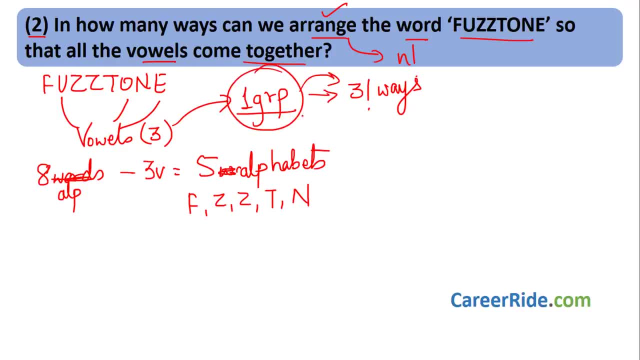 the group can be arranged in 3 factorial ways. Now, after we consider these 3 vowels as one group, we are left with 8 alphabets minus 3 vowels, that is 5 alphabets. So these 5 alphabets plus. 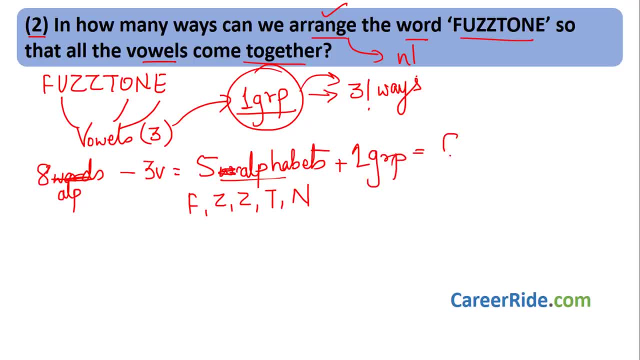 this one group will make total as 6.. So we will have 6 things, These 5 things plus this one thing. So we will have 6 things. These 6 things can be arranged in how many ways? 6 factorial ways, we have already learnt. If there are n things, we can arrange them. 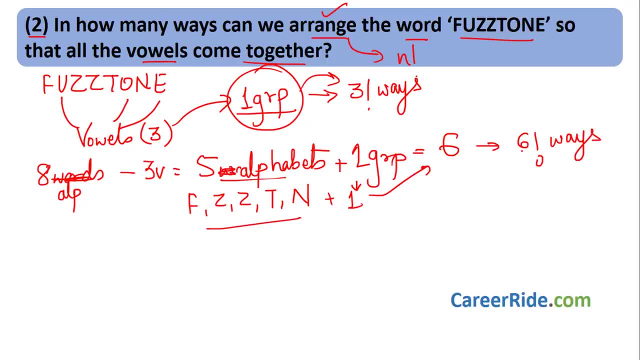 in n factorial ways. So these 6 things can be arranged in 6 factorial ways. So what you can say directly is that these 6, so the final answer in how many ways we can arrange is 6 factorial into 3 factorial. but no, that is not the answer. Why? 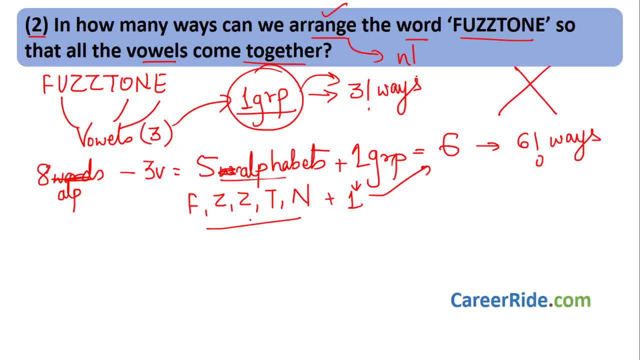 Let us see Now over here. if you observe carefully, what do we see over here? We have f, we have z, we have z, we have t and we have n. z gets repeated twice. So this is duplicate, this is duplication. There are 2, there is an alphabet which is getting repeated. 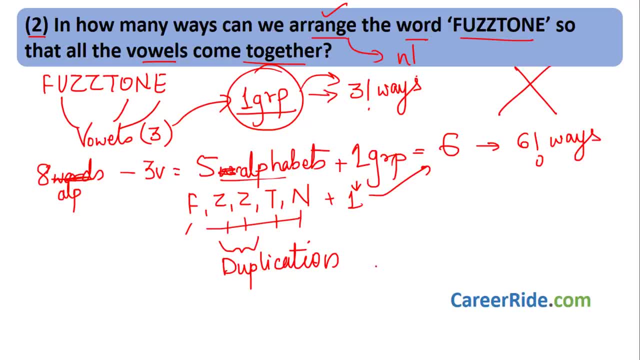 twice How to handle such things. It is very easy. Take a look on the right hand side you will understand it. If, say, we have n alphabets or n digits or n things, if we have n things, out of that one thing gets repeated, say, 4 times. 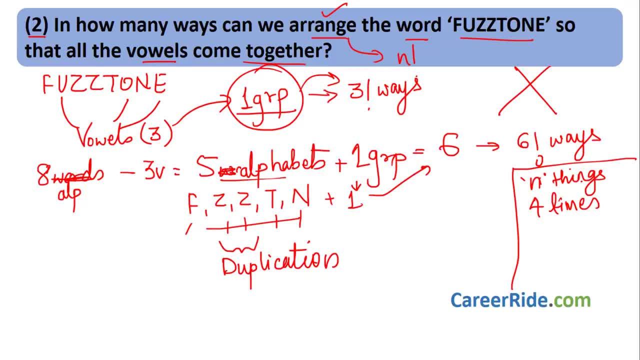 or we can say: if there are n alphabets and out of that one alphabet gets repeated 4 times, then how, in how much, how many ways we can arrange these n things? We already know that n things can be arranged in n factorial ways, But one alphabet or one thing is getting repeated. 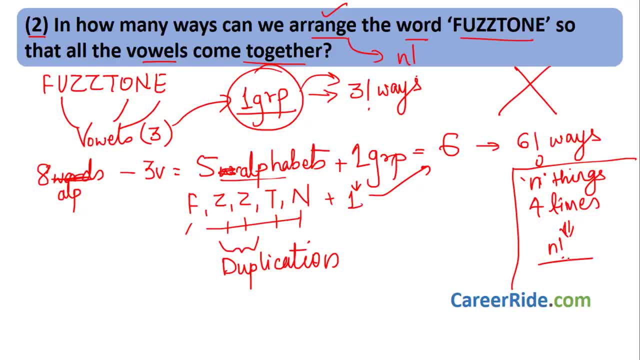 4 times. So how to arrange these? How many repetitions? Very easy. How many times does it get repeated? 4. Simply write 4- factorial. So over here we have 6 things. Out of that, one alphabet, that is, z, gets repeated. 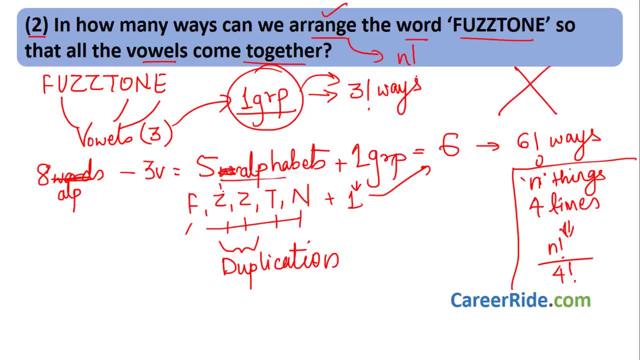 twice. That means z appears. how many times z appears once and twice 2 times. So total number of ways in which we can arrange these 6 things are 6 factorial upon z appears 2 times. So if z would have appeared 3 times, we would have written 6 factorial upon 3 factorial. 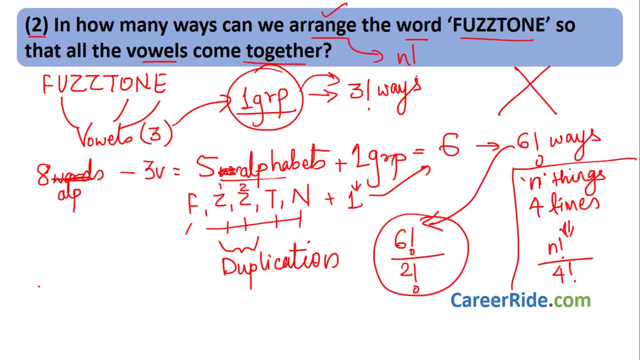 So now we can have the final answer as 3 factorial into 6, factorial upon 2 factorial, That would be 3 into 2 into 1, multiplied by 6 into 5, into 4, into 3, into 2, into 1 divided. 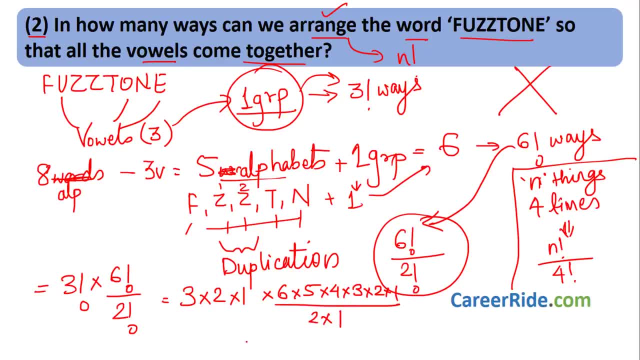 by 2 into 1.. Now take a look carefully over here. What have we written? We have written 3 factorial into 6, factorial upon 2 factorial. What is 2 factorial, 2 into 1.. Here also. 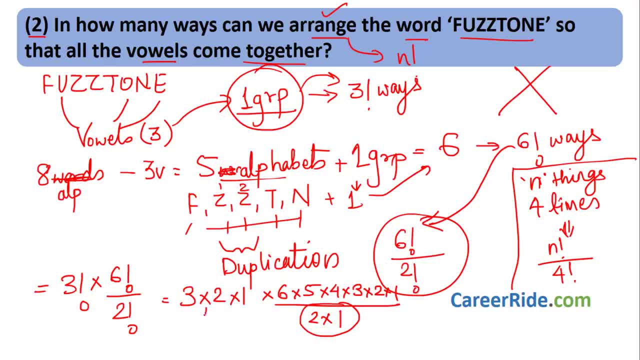 what we have: 3 into 2 into 1.. So we can write this as very easily: 3 into 2- factorial- Though it is not useful over here, Anyways, this gets cancelled over here, But always remember this trick, because whenever the values are greater, like 6 factorial, 7 factorial, 8 factorial. 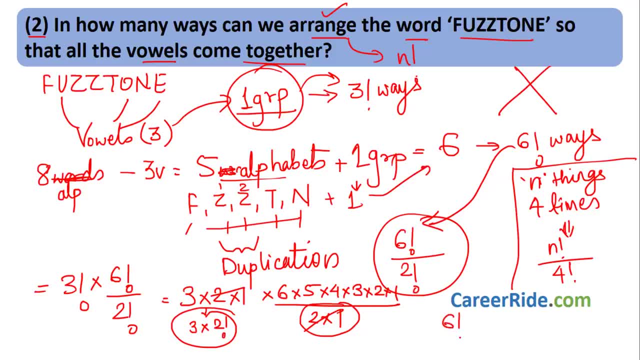 while division. you can use this trick: You can write 6 factorial as nothing, but 6 into 5 into 4 factorial or 6 into 5 factorial, like that. So that would help you to reduce the calculations. So right now this gets cancelled over here and the answer to this comes out. 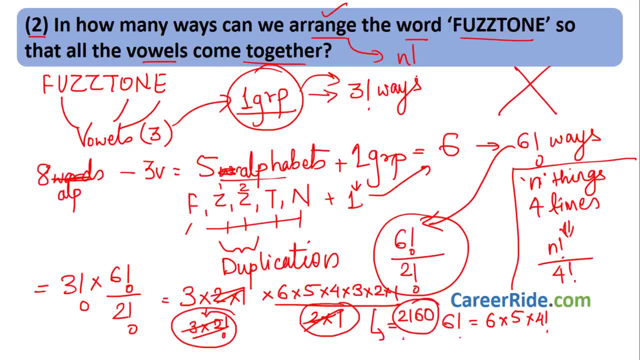 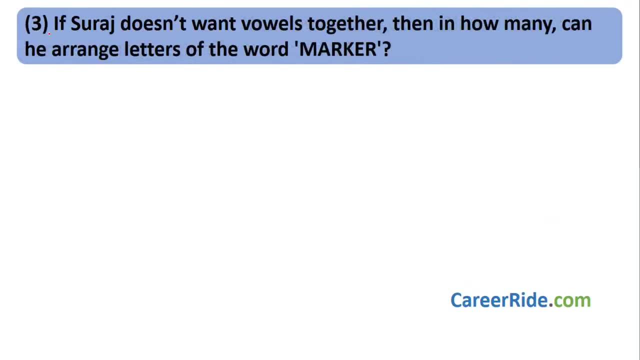 to be 2160 ways. The answer is 2160 ways. So in 2160 ways we can arrange the word of a stone so that all vowels come together. Moving to next question, Question number 3.. If Suraj doesn't want vowels together, then in how many ways can? 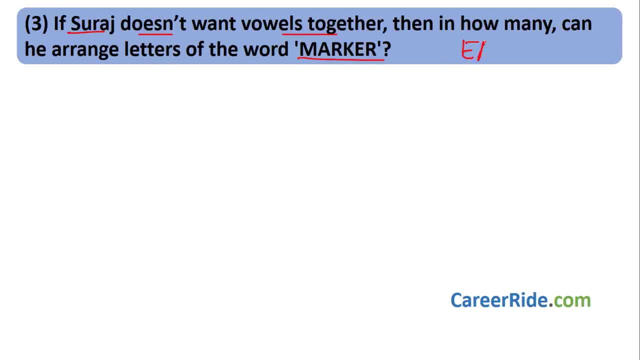 he arrange the letters of the word Marker. Again, this is very easy. If you have seen the probability video, then you will be able to solve this in a jiffy, very, very quickly. But even if you have not seen the probability video, no problem, We will learn again over. 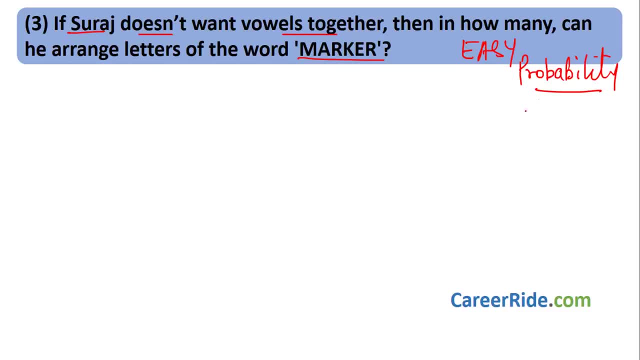 here how to solve these kind of sums. It is very easy. It is related to our question number 2.. Let us see What have we learnt in question number 2? That whenever we want the vowels together, what we should do Now over here? what they have? They have the word marker. 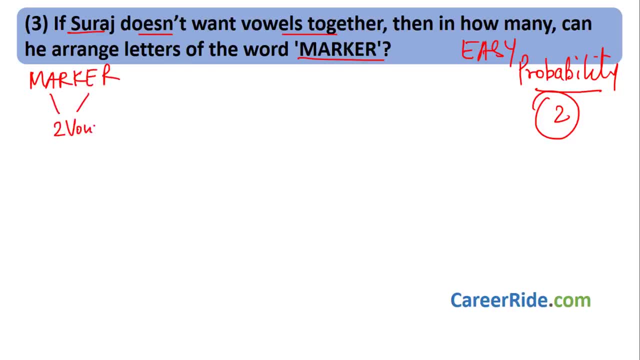 Which are the vowels over here? A and E. So there are two vowels. How many letters are left? Total is 6 letters. Out of that, 2 are vowels, So 4 letters are left. What are the letters? M, R, K and R? Now, what do they want? They do not want the vowels to be together. 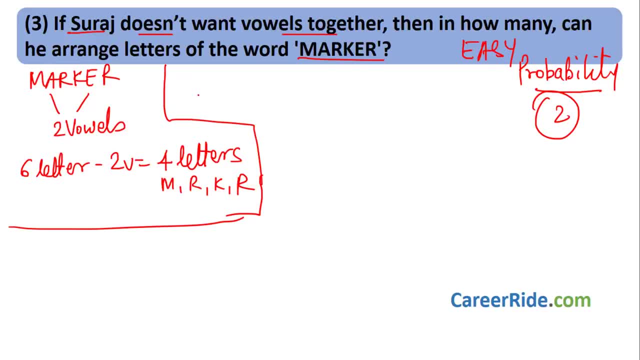 So how to find out the vowels should not be together Very easy. Total number of ways in which we can arrange the words is nothing but the ways in which we can arrange so that the vowels are always together. Vowels are always together, plus the ways in which the 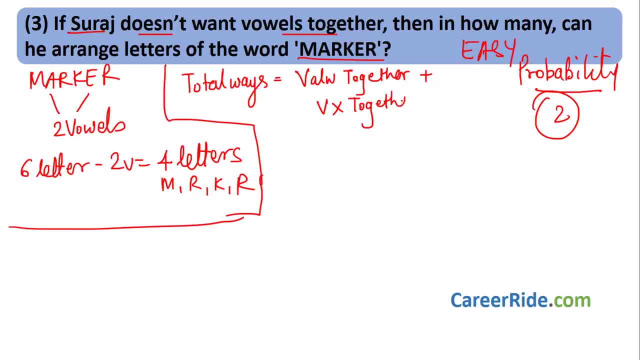 vowels are never together. It is very simple: Total number of ways in which we can arrange the all the letters of this word marker is simply the number of ways in which we can arrange so that the vowels are always together, plus number of ways in which we can arrange so that the always are vowels are never together. 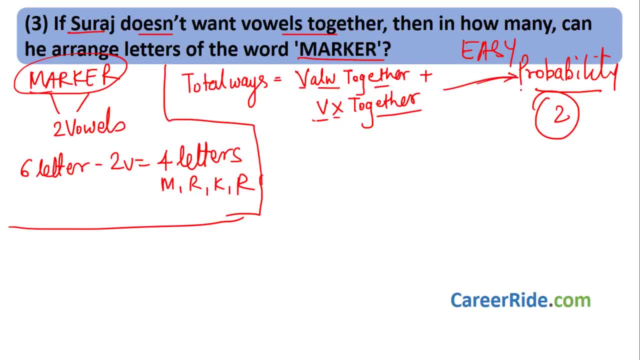 This is what we had seen in the probability video also. Please remember it is very easy that there is nothing much or complicated over here to understand or to remember. It is very easy just remember total ways in which we can arrange a word or this is nothing. 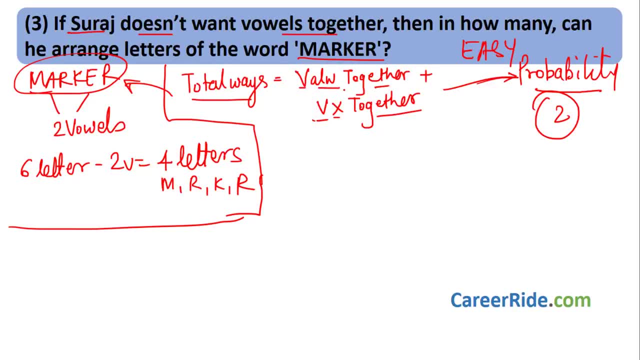 but our total number of ways in which the vowels always together and total number of ways in which vowels are never together. So of total number of ways in which vowels or never together will be nothing but total ways. Total ways minus the number of ways in which the vowels are always together. 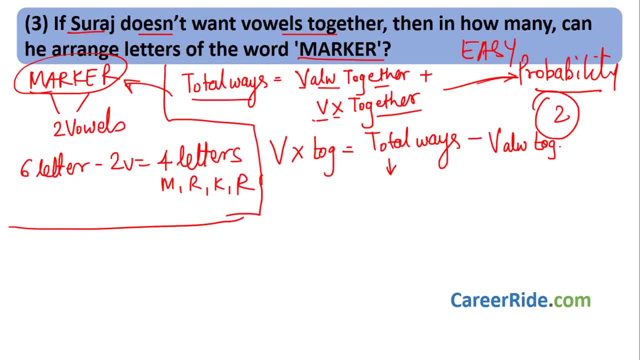 The total way. Total ways is: how much, How many letter? How many letters are there in the word marker? 1,, 2,, 3,, 4,, 5, 6.. So total ways are 6, factorial No, it is not 6. 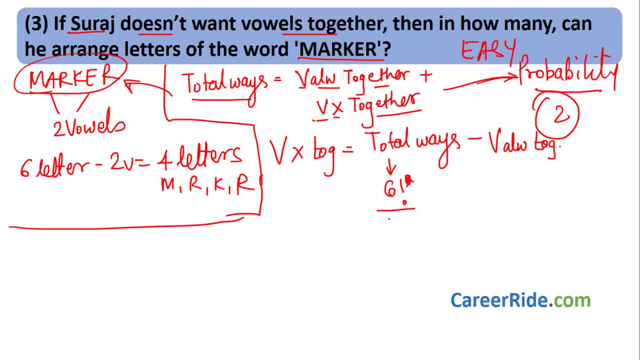 factorial, Then what it is. It is 6 factorial divided by. here you see the word or the letter R gets repeated 2 times, So 6 factorial. upon cancelling the repetition, 2 factorial, This is the total number of ways in which we can arrange the letters of the words marker. That is nothing. 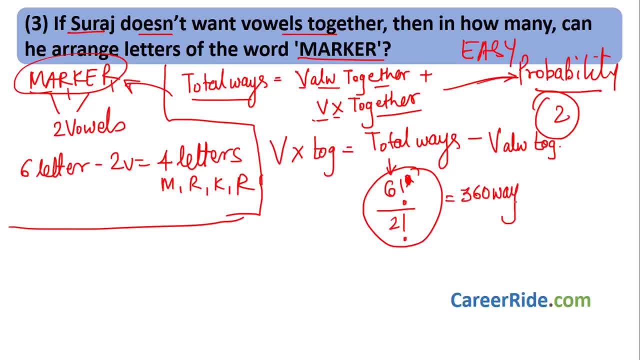 but that comes out to 360 ways. Now let us find out the total number of ways in which the vowels are always together. This is like the sum number 2 which we have seen. So vowels are always together. How to find vowels are always together? Make the vowels as one group. So 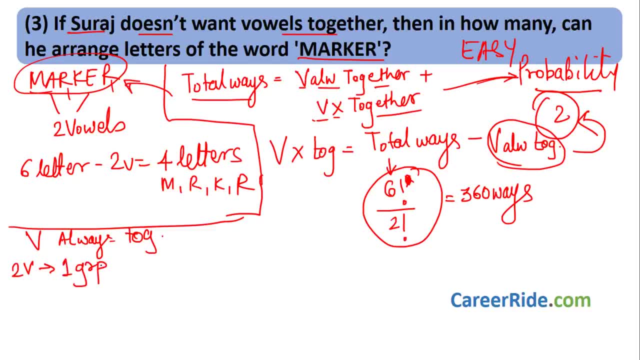 the two vowels become one group And the two vowels of the group can be arranged in two factorial ways. Now, when we make it as one one group, what are we left with? Six letters minus two vowels are four letters. So we 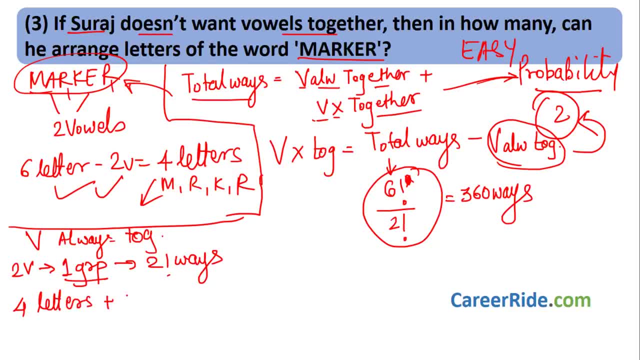 have four letters plus one group, That would be five things. These five things can be arranged in five factorial ways. No, not five factorial Why? Because four letters are M, R, K and R. R gets repeated twice, That is two times. So answer is: these five things can be arranged. 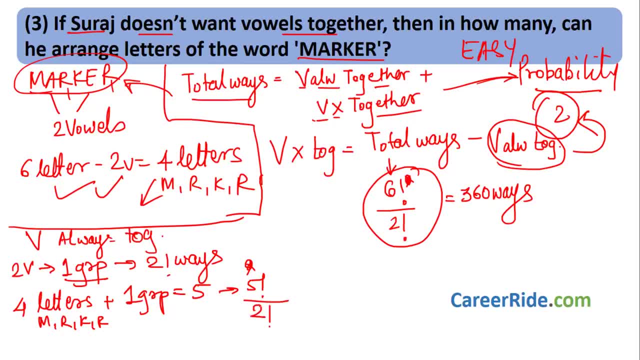 in five factorial ways: Five factorial divided by two factorial because we are cancelling the repetition Now. this is the way to arrange: four letters and one group plus in the group. we can arrange it in two factorial ways. we have already seen. So the total number of ways is five factorial. 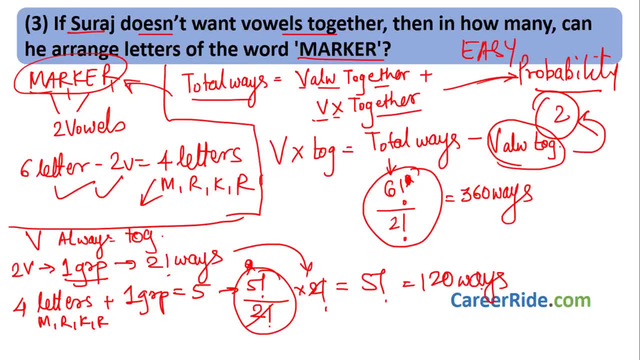 Five factorial is nothing but 120 ways. So the ways in which vowel can always be together is 120.. Total ways is 360. So the answer would be nothing but 360 minus 120. that would be 240 ways. So in 240 ways we can arrange the letters of. 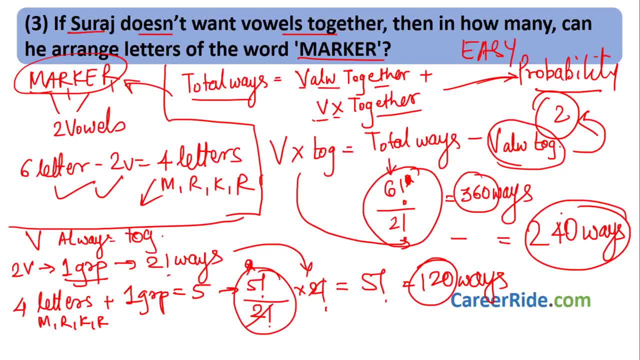 the word markers so that the vowels are never together. See how easy it was. there is nothing to it. very, very easy sum. So you just needed to remember that total ways is nothing but vowels always together plus vowels never together. If you know this, you will be able to solve the sum. Many of the sums rely on the these. 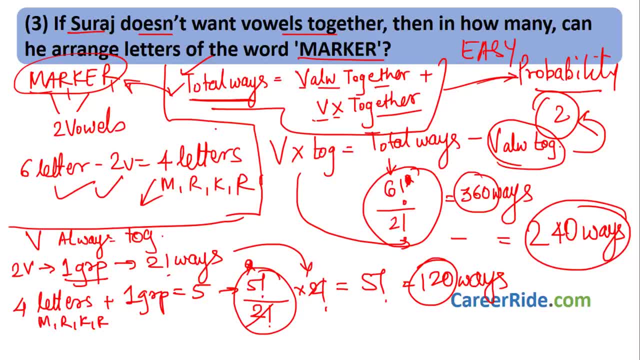 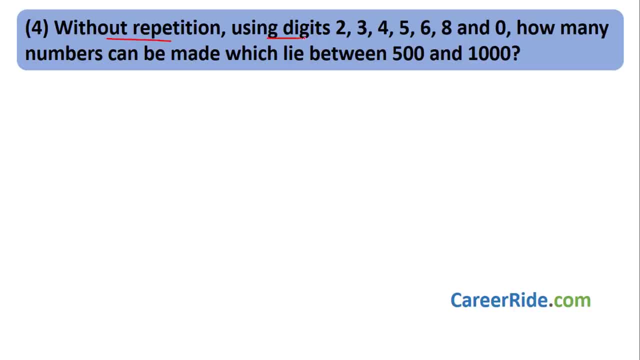 kind of small commands like one one, two, three, four, five, six, seven, eight, nine. common sense and common logic tricks to solve the sum. okay, now moving to next question, question number four: without repetition, using digits two, three, four, five, six, eight and zero, how? 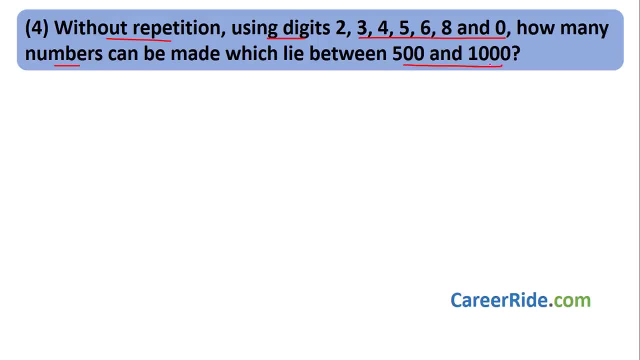 many numbers can be made, which lie between 500 and 1000. again, this is a easy sum and in this sum we are going to see two methods, okay, two ways to solve this sum. one is by the formula right, one is by the formula and other is by logic or the common sense. okay, 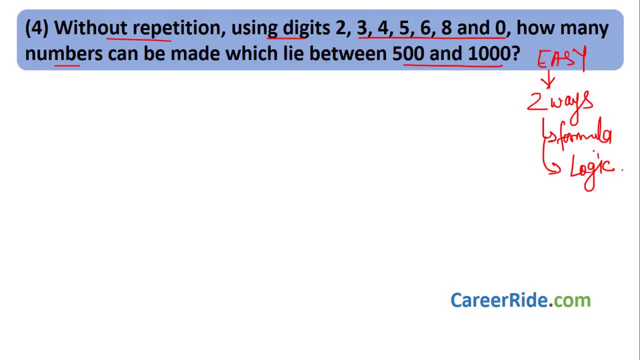 now first, let us solve it by formula, right? or let us solve by logic first. okay, let's take logic first. now, what is given over here, without repetition? so repetition should not be there. and we have to make numbers which lie between 500 and 1000. okay, so number has. 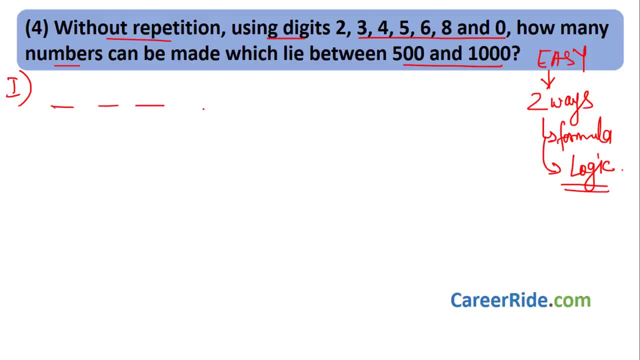 to be three digit: one, two and three, because we want a number which which is between the 500, that is, more than 500 and less than 1000. okay, now, how many, whatever possible, what possible choices are given: two, three, four, five, six, eight and zero. now, out of that, if we see, if 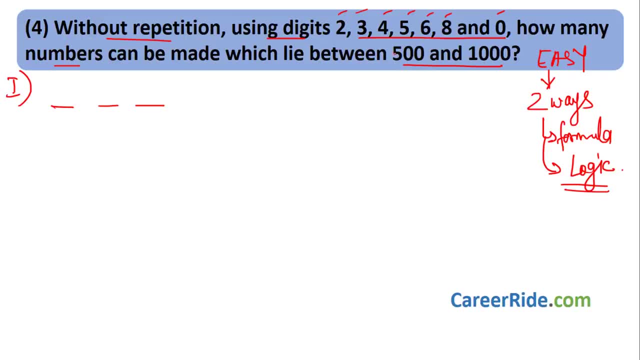 you take the first digit of the number as two, will it lie between 500 and 1000? no, three. if we take it as three: no. if you take it as four: no. if you take it as five: yes, possible, because 500 and one to 599 lies between 500 to 1000. 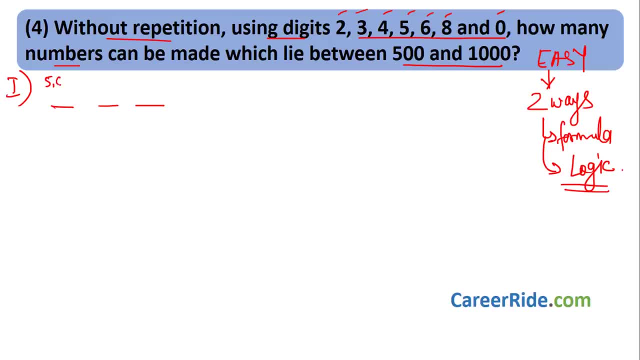 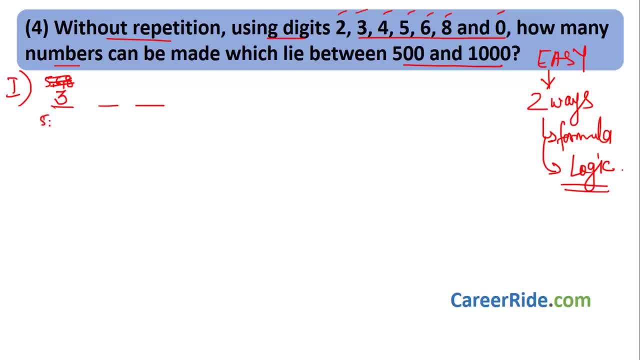 are three choices possible. okay, what are the choices? five, six and eight. now here, three choices are possible, since they have given that there should not be repetition. okay, that means that total numbers- how many are these total numbers- two, three, four, five, six, eight and zero total are: 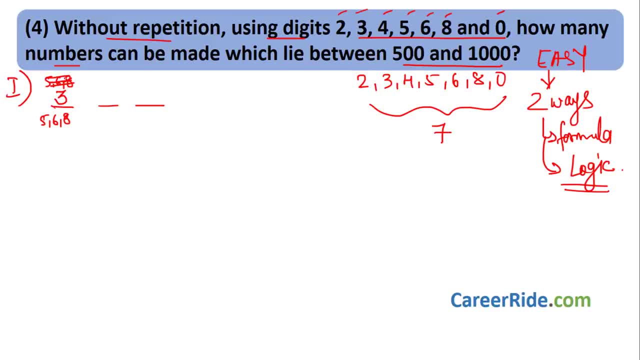 seven. okay, seven numbers are there. out of that, one number gets utilized over here. whichever number it is there out of five, six, eight, doesn't matter, but one number gets utilized. so how many are remaining? seven minus one. remaining are six. okay, now, here anything can come, because now we have already. 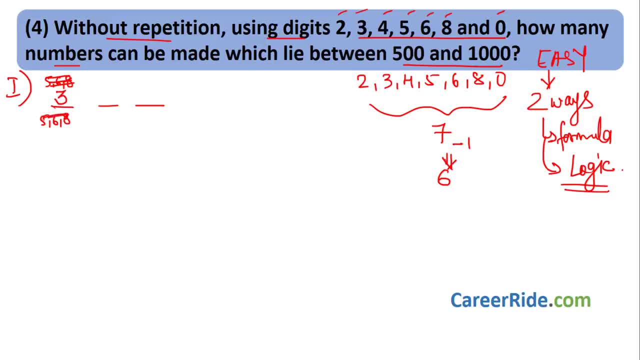 know that it should be greater than 500. we have already known that it should be greater than 500. we have already known that it should be greater than 500. we have already chosen numbers which are related to, which will make the number greater than 500, so all the possible numbers can come over here. okay, so how many out of seven? since there is? 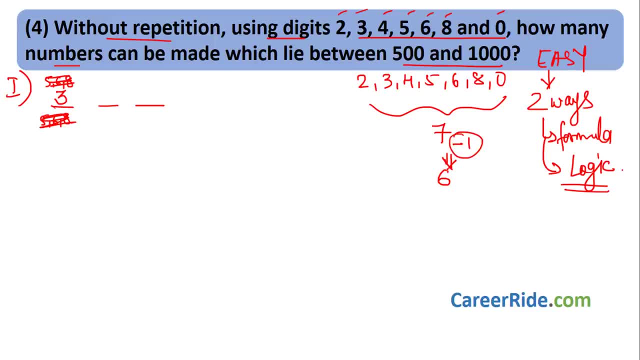 no repetition. we have already used one number. okay, so how many digits are remaining? six digits are remaining right. so here six possible choices are there. out of these six, anyone can come over here again. one has been utilized, correct. how many possible choices remain? now five? so there are. 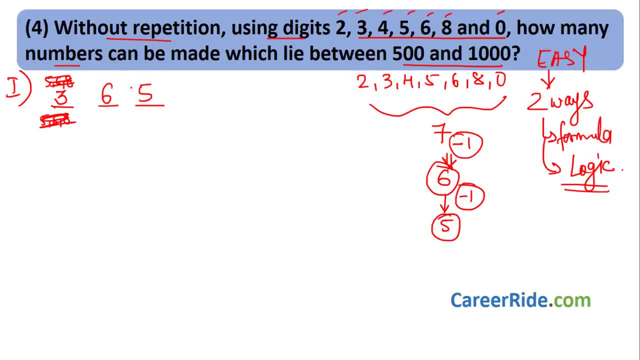 five possible choices over here. so condition was five hundred to one thousand. so we did not take seven over here, we took directly only three, because only three numbers- five, six and eight- will make sure that our final answer, or all the numbers which we form, will lie between five hundred and. 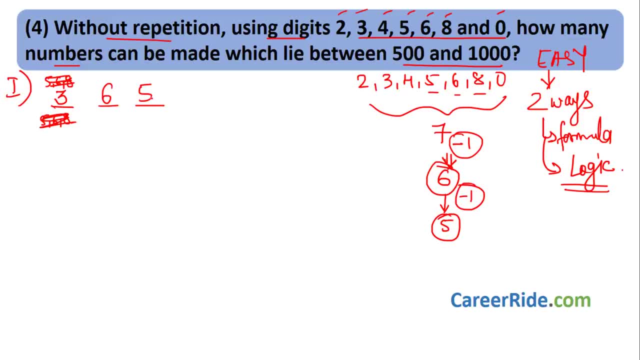 one thousand. so the possible choices are: we have put in here three choices can come here. six digits can come. any of the possible six digits here. any of the possible five digits can come, okay. So what is the final answer? How many possible numbers are possible? 3 x 6 x 5.. 3 x 6 is. 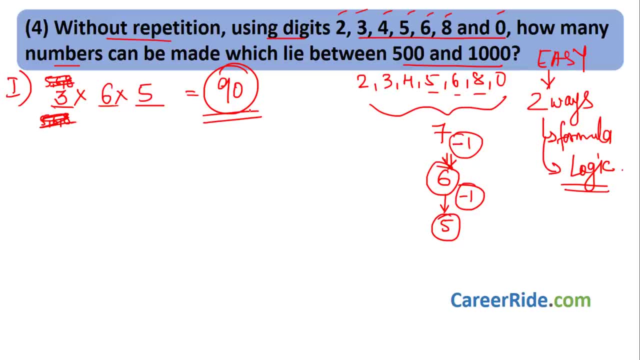 18.. 18 x 5 is 90. This is the answer. This is the answer because there is no repetition. If they say repetition is allowed, what will be the answer? Let us see Repetition is allowed First. we want the number between 500 and 1000.. So there are three possible choices. 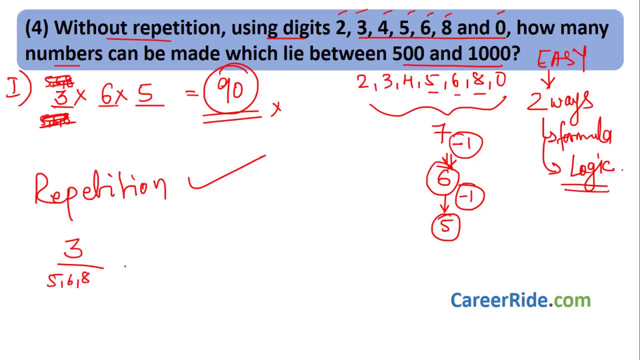 again over here: 5,, 6 or 8.. Second number, third number: Now, even if we use one number over here, still repetition is allowed. So again we have the entire set, That is, seven possible choices over here Again, even if we use one number, two numbers over here. 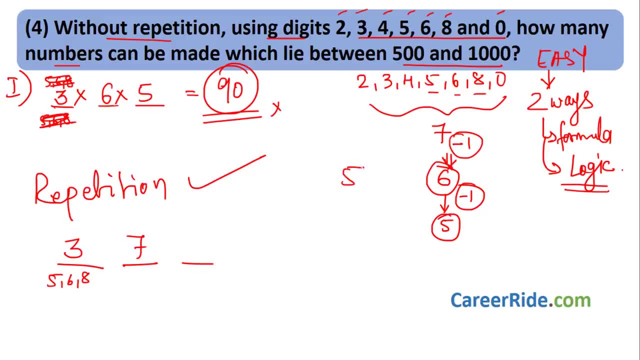 we can. repetition is allowed. That means if we take 5 at start, then 555 is allowed. Initially, over here 555 was not allowed. Why? Because repetition was not allowed. But over here 555 is allowed in second number. So again we have the entire set. So again. 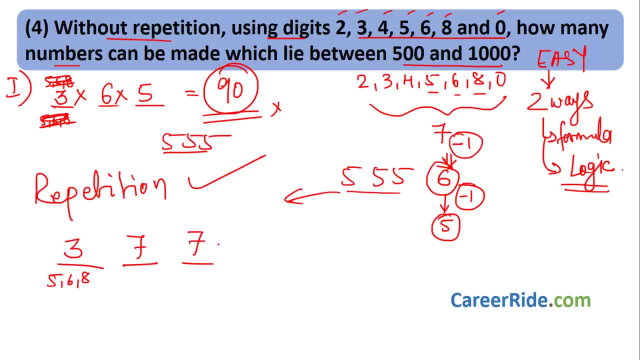 at the last we will have seven possible choices. We can take any number, So the answer will be: 7 x 7 is 49.. 49 x 3 or 21 x 7. That would be 7147.. But we do not want repetition over. 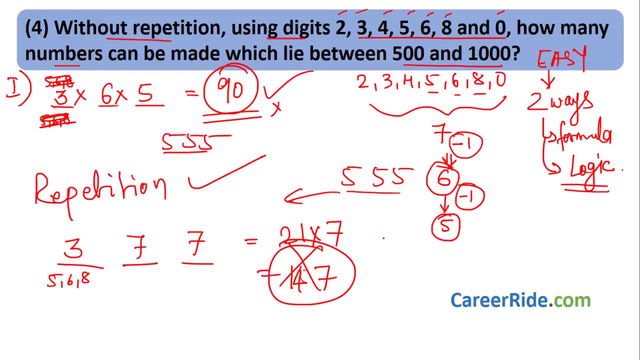 here. So our answer is 90.. So have you understood what exactly it means by repetition and how, by logic, we can solve such kind of sums. Now let us move on to the second method. Second method is formula based method. 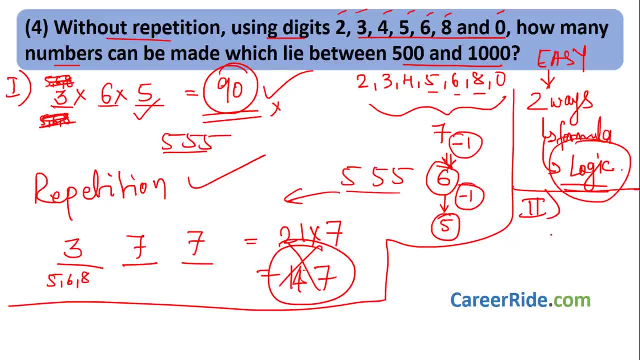 So let us move on to the second method. The second method is formula based method, So we have two options. Okay Now, second method is similar Three digit number. we have to form Now the first digit, It can be 5.. It can be 6. Or it can be 8.. So there are three. 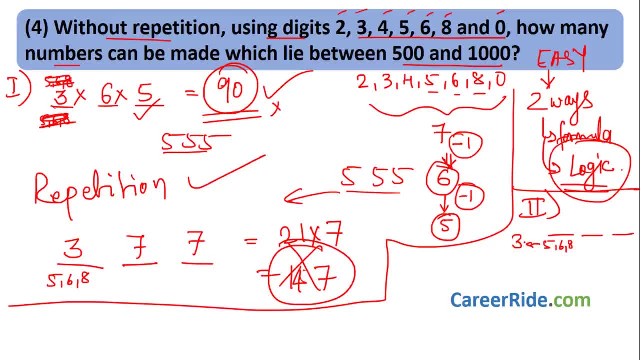 possible choices. Out of these three choices, we have to select one digit to put over here. So three choices are there. We have to select one digit. Select means combination, So we have c. Now please remember whenever they are saying that using these digits form a. 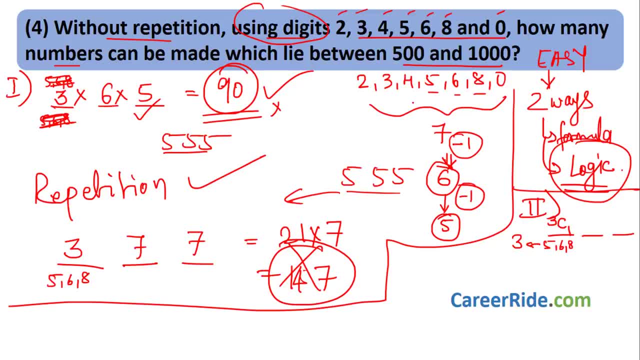 okay, whenever they are seeing that, use these digits or select these digits directly, you should mention combination. okay, here again there are three possible choices: 5, 6, 8. out of that we have to select one digit and put over here. okay, so select is combination. so we have 3 c 1 multiplied. 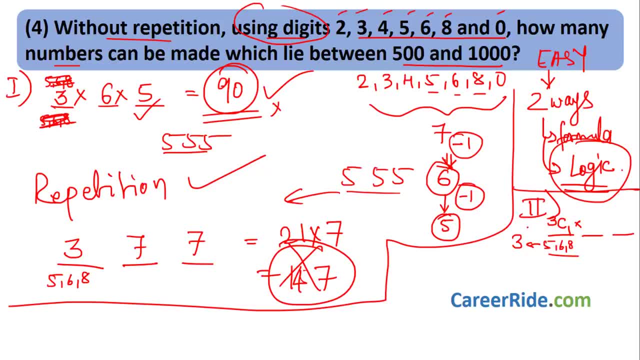 by. here again, one digit has already been used, so there are six possible choices. so out of six, we have to choose one. out of six, we have to select one. so 6 c, 1 right. and out of six, again one digit is used in this place. so over here, only five digits remain. out of five, we have to choose. 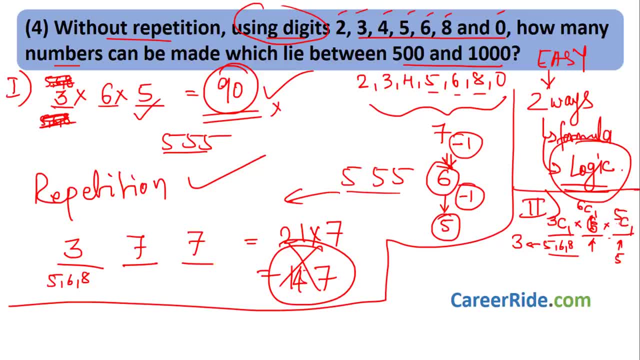 one. choose means select, select means combination. so answer is 3 c 1 multiplied by 6 c 1, multiplied by 5 c 1. what is it? what is 3 c 1? it would be 3 factorial upon 1 factorial. 3 c 1: it would be 3 factorial upon 1 factorial. 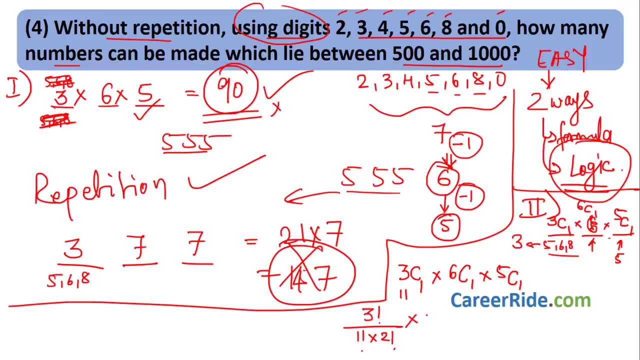 3 c 1 multiplied by 3 minus 1 is 2 factorial x 6 factorial 1 factorial. 6 minus 1 is 5, 5 factorial multiplied by 5 factorial 1 factorial multiplied by 4 factorial. now 3 factorial can be written as: 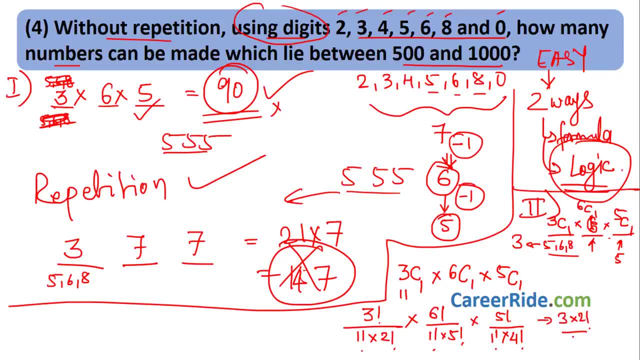 we will write it over here: 3 into 2 factorial divided by 2 factorial. that gets cancelled. same way, 6 factorial is 6 vector into 5 factorial. that gets cancelled. so we get 6 over here. 5 factorial is 5 into 4 factorial. 4 factorial. 4 factorial gets cancelled, We get 5 over. 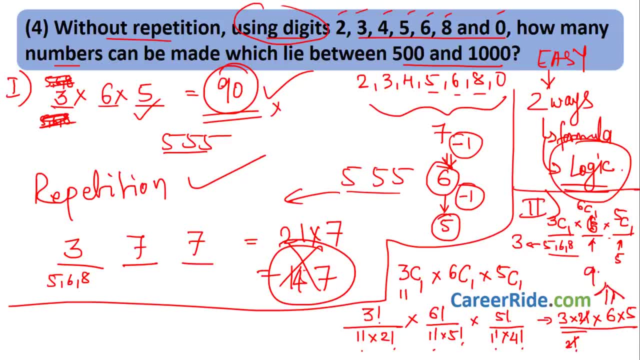 here We get it as 90.. 3 into 6 into 5 is 90, just like the previous answer. So you can go any way. You can go by the formula also, You can go by simple logic also It. 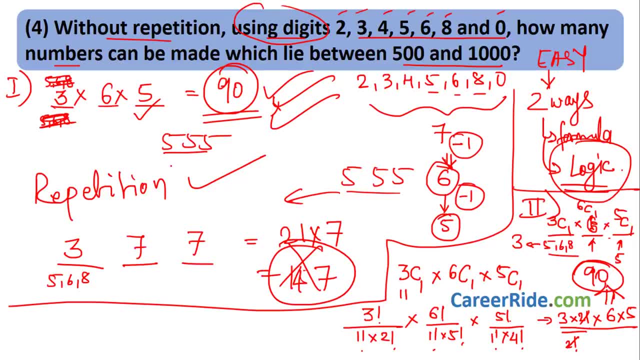 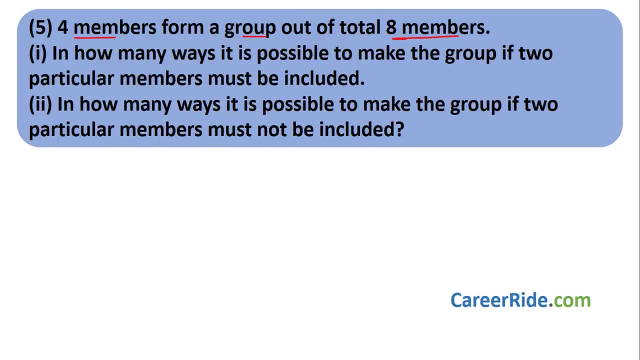 is best to develop both the areas, because some sums you can solve very quickly using logic, Some sums you can solve very quickly using formula. Moving to next question, Question number 5.. 4 members form a group out of total 8 members. Point 1. In how many ways it is? 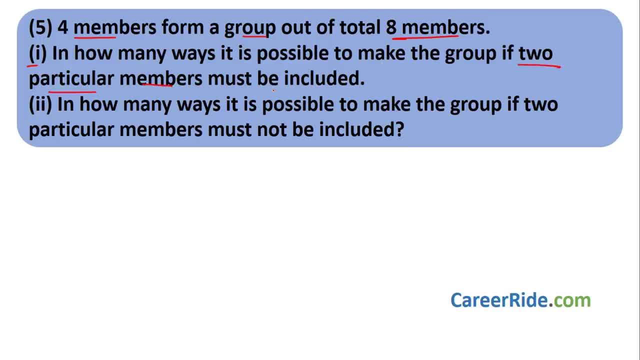 possible to make a group if 2 particular members must be included? Point number 2.. In how many ways it is possible to make the group if 2 particular members must not be included? Now here there are 2 sub questions Now. earlier we saw how to solve the sum using logic also. 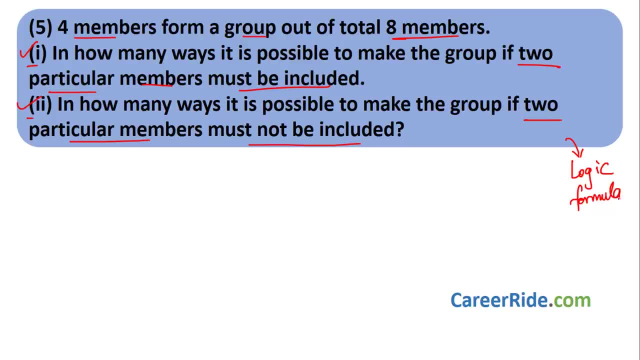 and formula also. You might have thought that using logic it is faster. You might have thought that using logic it is faster. You might have thought that using logic it is faster, There is no need to use formula. But over here I will show you how formula is also very, very useful and it is very important to learn it. Let 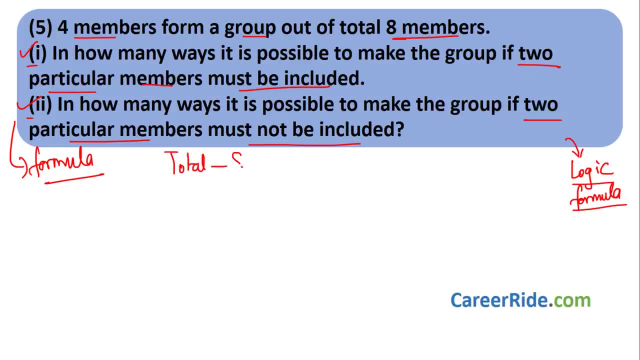 us see What are they saying. There are total 8 members. There are total 8 members Say let us let the members be A, B, C, D, E, F, G and H. These are the 8 members Now in. 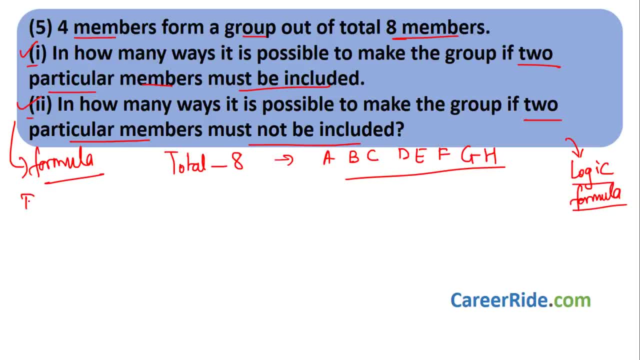 how many ways it is possible. the sub question 1.. Sub question 1.. In how many ways it is possible to make a group of 2 people if 2 particular members must be included? They already say that the group must be of 4 members. At the start they say 4 members must be in. 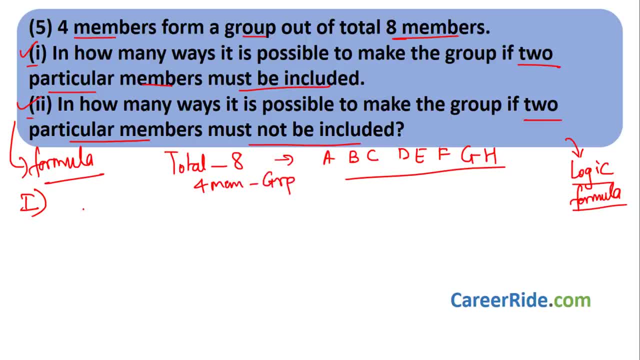 the group. But the condition in the first case is that 2 particular members must be included always. Let us assume that member C and member F. both these members have to be included compulsorily. They must be included. So 2 places have been occupied by these. How many places are remaining? 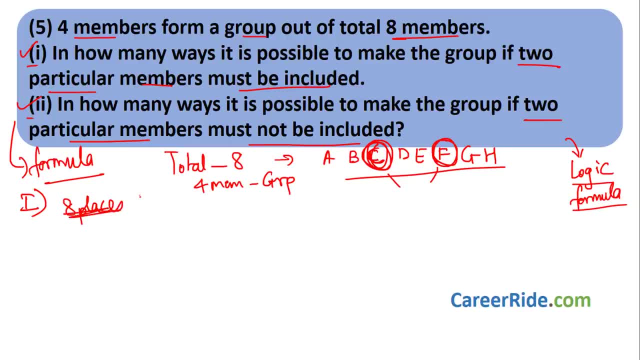 Now 8 places. There are 4 places in a group, So 4 members can form a group. That means there are 4 places in a group. Out of that, 2 places are already occupied by C and F. So out of 4 places 2 places are occupied, So only 2 places remain. That means you can. 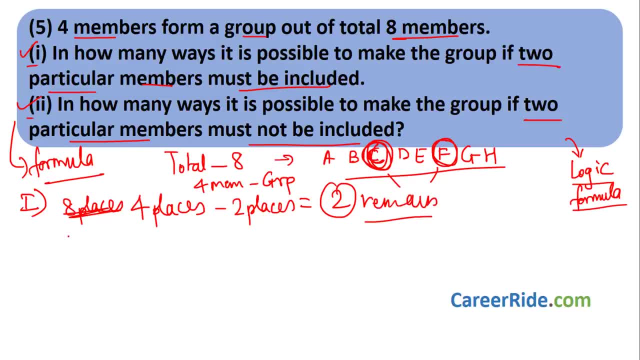 select only 2 members. now Total members are 8 total members, But out of that we have already selected 2 members. Those have to be included compulsorily. So how many members are remaining? One, 2,, 3,? 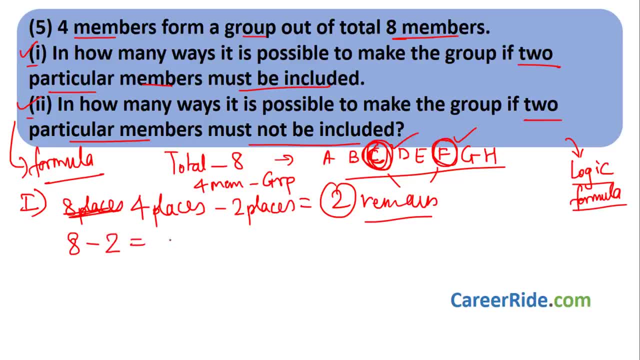 4, 5 & 6.. So two members are already selected, So 6 members remain. We have to fill these two remaining places using only these 6 members. Here we have to make the group. That means we have to choose people to form the group. That means we have to select people to form. 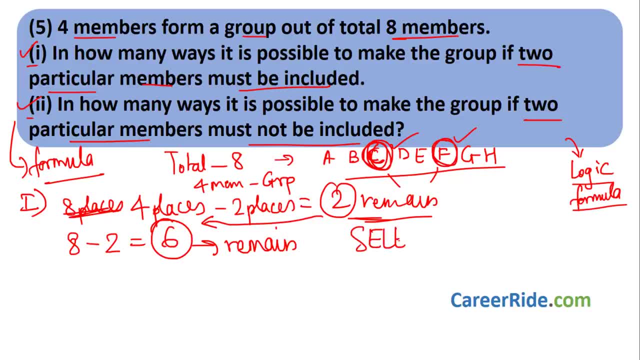 the group. That means we have to select people to form the group. So we have to select people and select means. combination Combination: that means we have 6 people remaining out of that, using this 6 people, we have to fill the remaining 2 seats. We have to choose 2 people out of 6.. 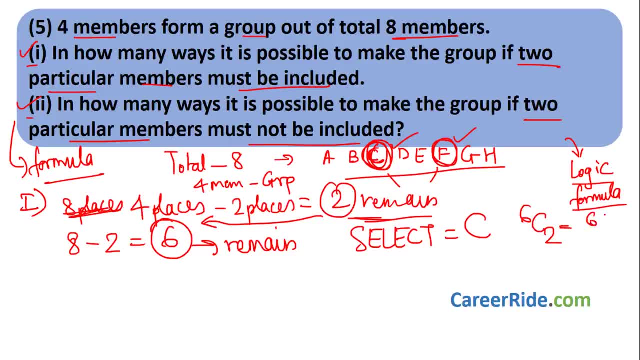 We have to select 2 people out of 6.. So it would be 6 factorial upon 2 factorial into 4 factorial. that would be equal to 6 into 5 into 4 factorial, divided by 2 factorial into 4 factorial. This 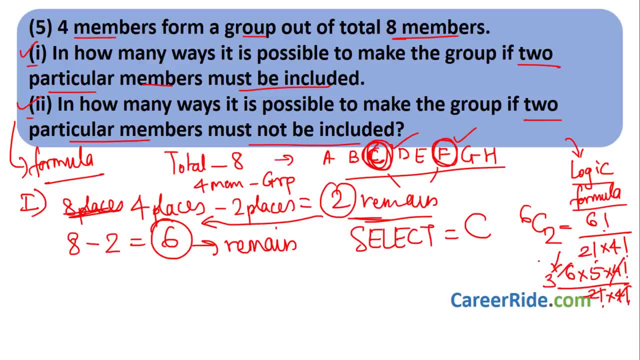 gets cancelled. 2, factorial is nothing but 2.. 2, 3 is a answer would be 15.. There are 15 ways: in case of 1, in case of point number 1 or question number 1.. Now let us take the question. 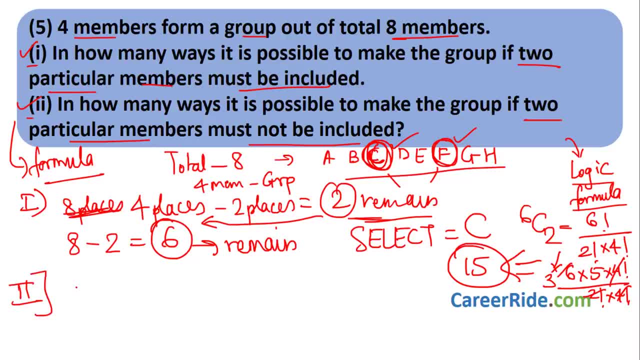 number 2 or case 2.. Here they are saying that 2 particular members must not be included. Let us assume that now over here, C and F must not be included at all in the group. How many members are remaining? Total: there are 8 members. out of that, 2 must not be included, So 6 members remain. 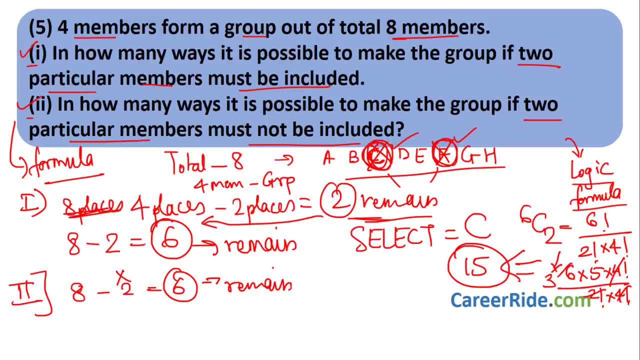 again, 6 are remaining. So whatever group we have to form, we have to form out of these 6 members. they are given that the group has to be formed, But C and F, 2 members, that is, C and F must not. 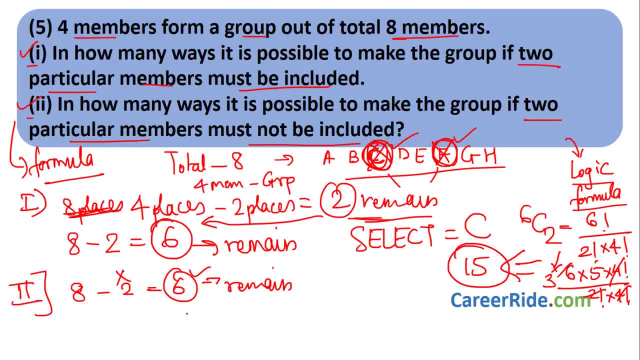 be included at all. 2 particular members must not be included at all. So we have to fill the 4 vacancies which are there in the group using these 6 people. So there are 6 people, We have to fill 4 vacancies. that is, we have to fill that. we have to choose. 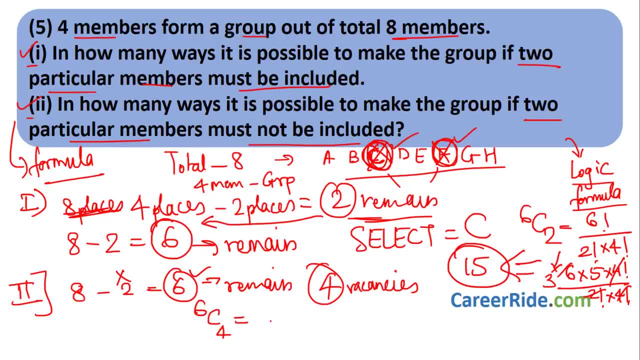 4 people, that is select 4 people. Select means combination. So number of ways is 6 factorial divided by 4 factorial multiplied by 2 factorial, that will again come out to 15 ways. So both the answer for both of them is: 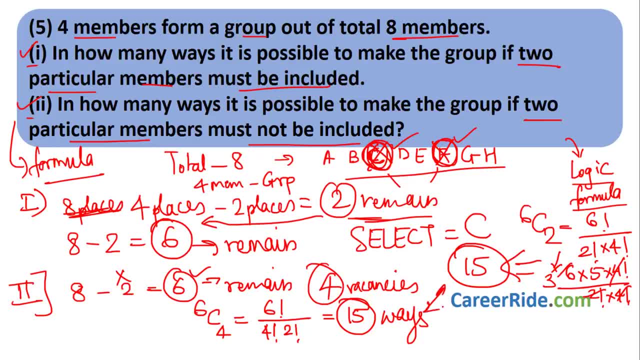 15 ways. So see how easy it was using the formula. This is since I am explaining. it might have taken time, But using the formula, you can simply write 6C2.. Need 2 places. Only 2 people should be considered out of 6.. So 6C2, you will get this answer. 6C4: you will. 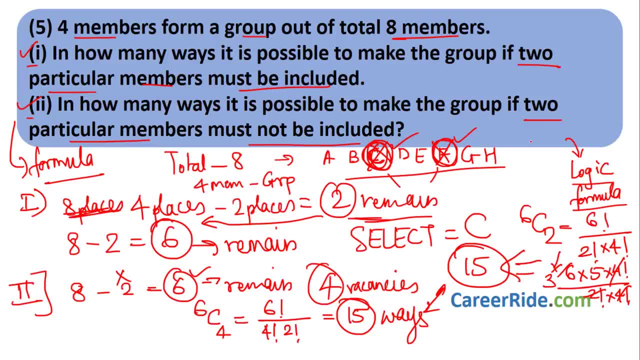 get the answer as 15 ways That is done, You will be able to solve combination problems. If you practice, you will be able to solve combination problems in 45 seconds to 1 minute, Very easily. Just remember when to use logic, when to use formula, and with practice you will be able. 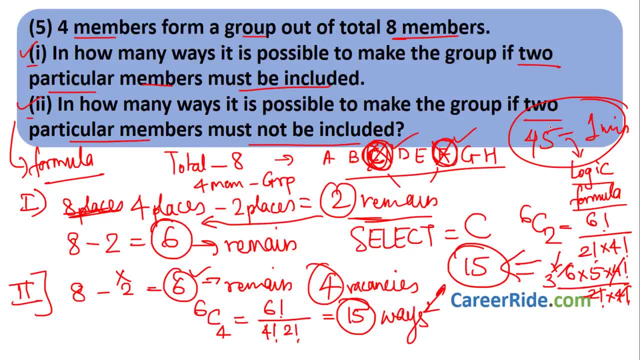 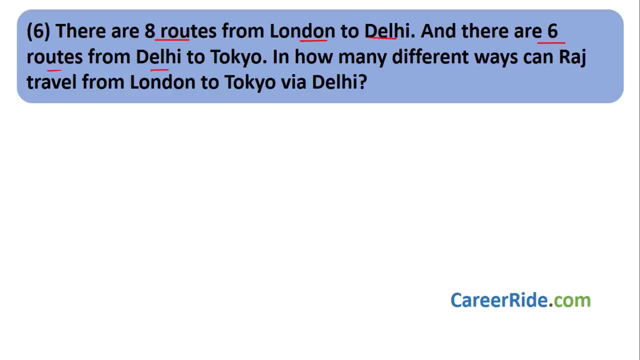 to get a grasp of this, It is very, very easy Moving to question number 6.. There are 8 routes from London to Delhi and there are 6 routes from Delhi to Tokyo. In how many different ways can Raj travel from London to Tokyo via Delhi? Now, over here again, we can solve this. 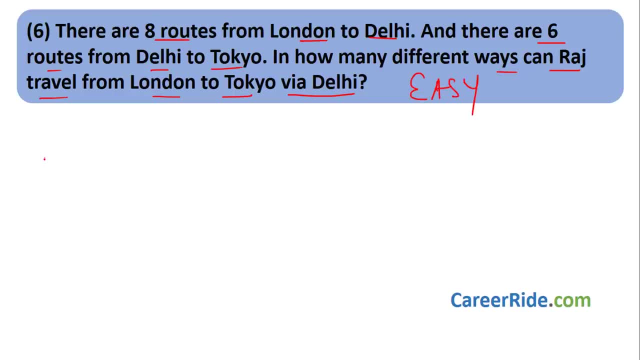 by common logic, It is extremely easy sum. Let us see how. Let us see here- Raj can travel from London to IR shots. to slick doesn't mean six places from London to FL shots. Right now, Raj must go through a stratagem where he can vamos. 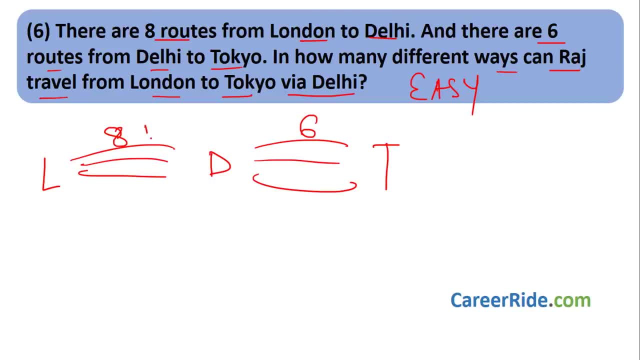 in prompt and final. is school out liquid or 아주 simple project. At the point which we have to do, that is, when we add a contact number, then we can get a value to L. Right now, Raj must be using the formula smarter Whereyeah. if you add LAnC to the class matrix, then 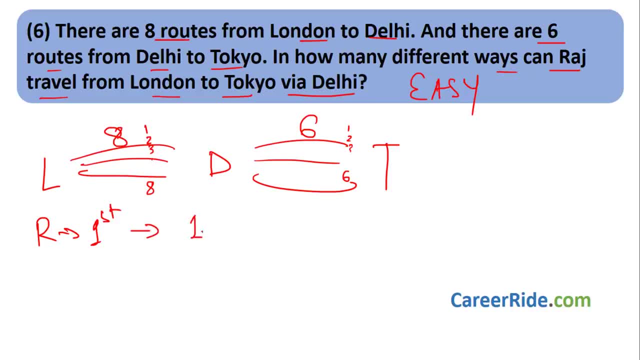 this will equal toulink in progress. What about London torn of Interior? aha, London battle takes way number 1 from London to Delhi When he reaches Delhi for way number 1, how many options are there for going Delhi to Tokyo? There are 6 options, because there are 6 ways. 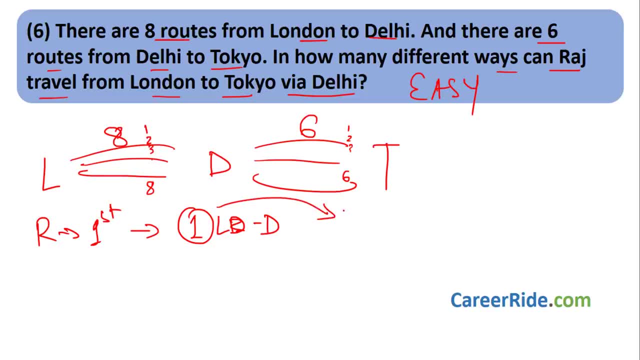 So for road number 1 or way number 1, he has 6 choices to go from Delhi to Tokyo. Same way, if Raj takes the second way and reaches Delhi, again from Delhi to Tokyo, how many choices he will have? Again, 6 choices he will have. He can go by any way. So for every 8, 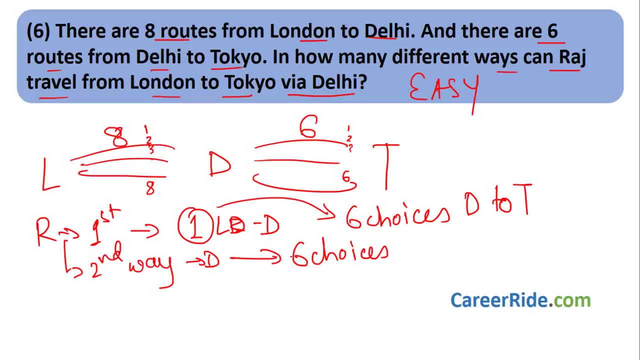 way, all the ways in this, from London to Delhi, Raj will have 6 choices. That means for 8 ways of London to Delhi. for each way Raj will have 6 choices. That is totally 48 choices would be there with Raj, and this is nothing but the number 1.. 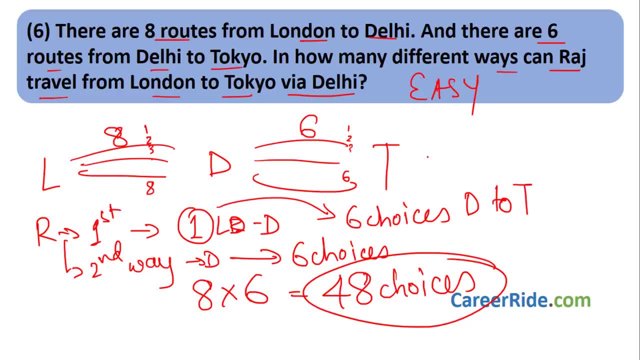 Number of different ways in which Raj can travel from London to Delhi and London to Tokyo via Delhi. You can count it. Let us see how. For first way, 6 choices. Second way, 6 choices I will write over here. For first way, from London to Delhi, there are: 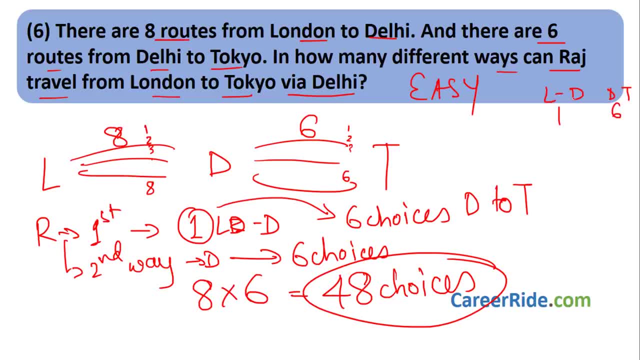 6 choices: from Delhi to Tokyo, Delhi to Tokyo, and this is London to Delhi. For second way, 6 choices. Third way: 6 choices. Fourth way: 6.. 5,, 6,, 7,, 6.. For the 8th way, also, 6 choices. 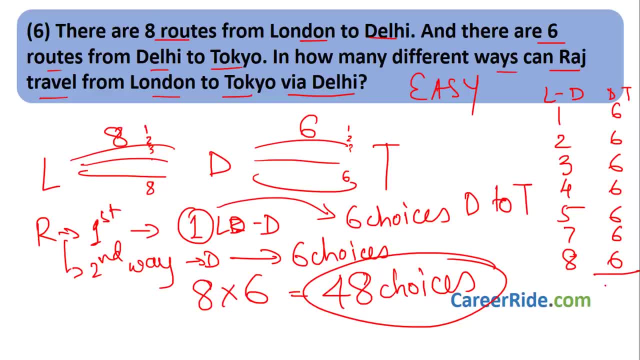 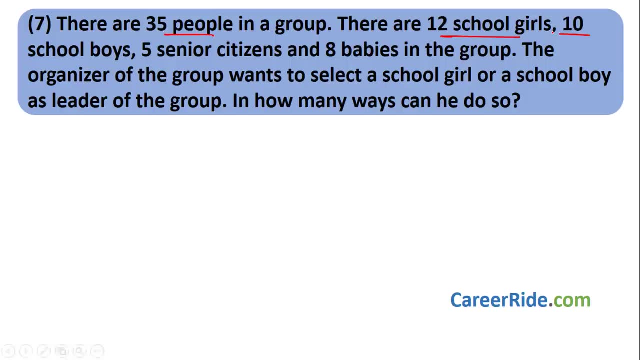 How many different ways are possible? 1,, 2, 6.. 6 x 8,, 48.. That is what we did: 8 x 6.. See how easy it was. Moving to next question, Question number 7.. There are 35 people in a group. There are 12 school girls, 10 school. 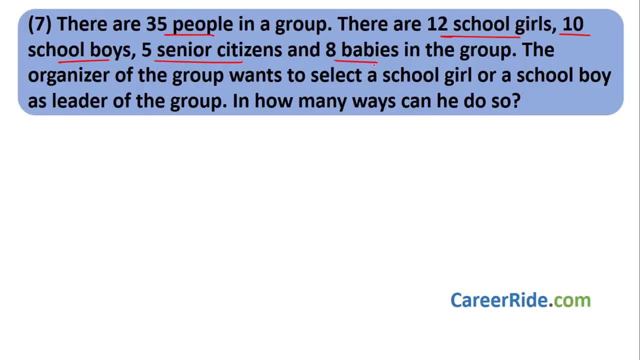 boys, 5 senior citizens and 8 babies in the group. The organizer of the group wants to select a school girl or school boy as leader of the group. In how many ways can he do so? Again, it is very easy. Again, we can solve it by 2 ways. We will see both the ways of logic and formula. Very easy. 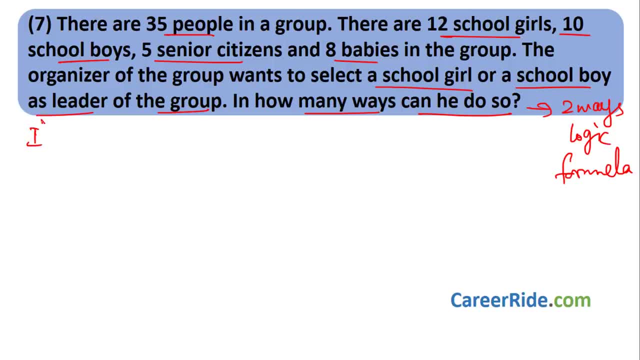 Both are easy Now. first we will see formula this time. Now formula Now. he wants to select a school girl or school boy as leader. How many leaders does the person want? Person wants 1 leader. Person wants to select 1 leader. So this is nothing but value of r, because 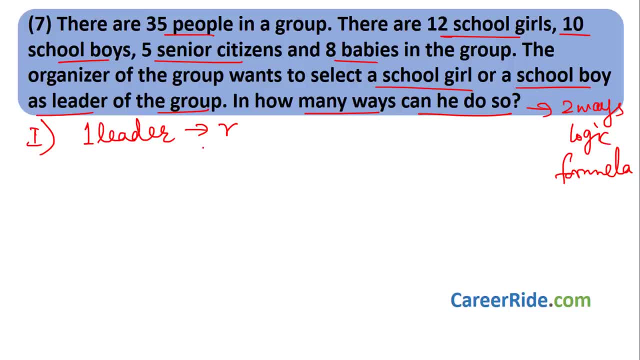 we select r things out of n one. the organizer wants to select one leader, that is r is one out of who? out of a group of 35 people, but your n will not be 35 why? because the organizer does not want any one leader. the organizer wants a leader only from only who is a school girl or who is a school boy. okay, so. 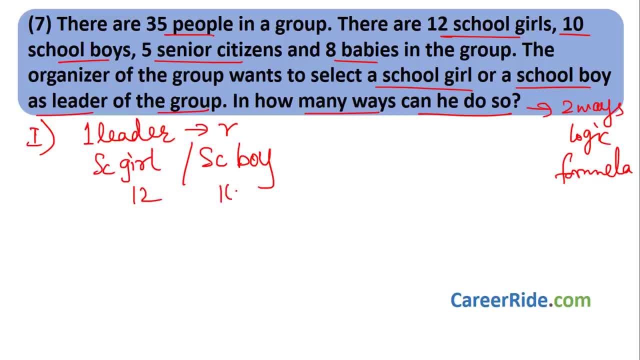 total number of people. school girl is 12, school boy are 10. so out of these 22 only. okay, school girl or school boy? only out of these 22. the organizer want to select one leader, so n is nothing but 22. we have to select r things out of n, so we have to select one leader out of these 22. 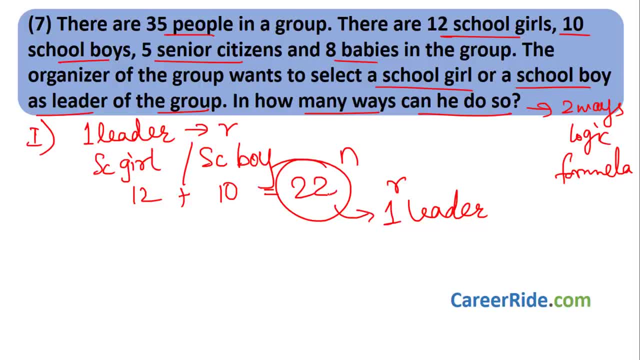 only, we don't want 35 people, because 35 people includes five senior citizens and eight babies. but the leader should be from school, should be a school girl or a school boy. so we want to select one leader from 22 people, right, so what? since we have to select what we'll do. selection means c. we have to select r. 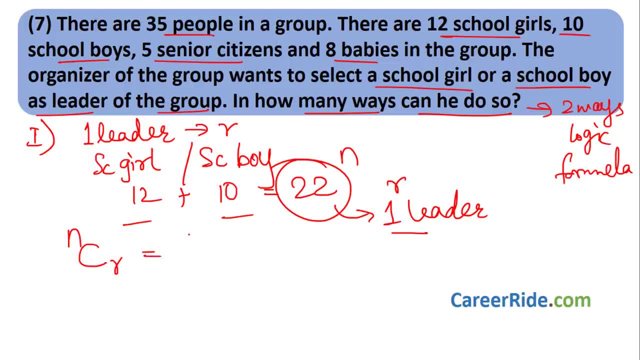 people from n things r things from n things. that is 22 c 1, 22 factorial upon 1 factorial into 22 minus 1 is 21 factorial. that would be 22. right now, let us see by logic- okay, this is by logic. how many school girls and school boys are there? 12 school girls, 10 school boy or 10? 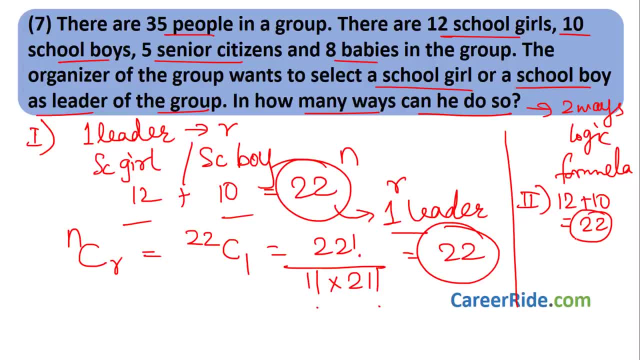 school boys. so 22 people are there. out of these 22 people, we want just one leader. if you want one leader, how many choices do the organizer have? they have 22 choices. they can choose anyone from these 22. okay, we will not consider senior citizens and babies because the organizer want a school girl. 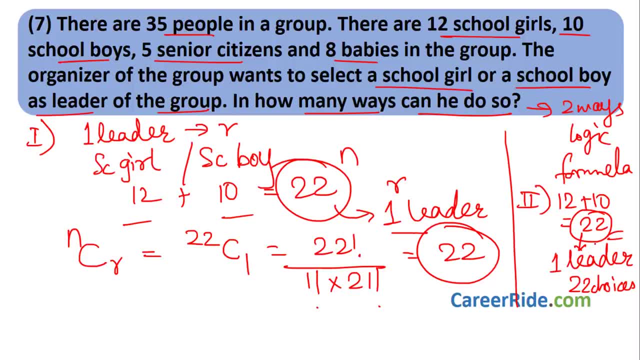 or a schoolboy as leader. so we will consider only 22 people. so out of 22 people, we want one leader. so the people? how many choices are there for this position, this vacant position of leader? there are 22 choices with the organizer. so answer is 22. see, with logic. also, we got the same answer. now, if they. 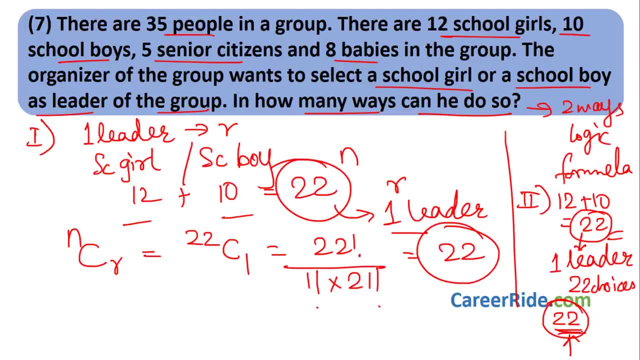 would have said that the organizer of the group want to select one person as leader of the group. then we can simply say: we want one leader. okay, this vacant position of one leader has to be selected. how many possible candidates are there? 35 choices are there because there are 35 people. 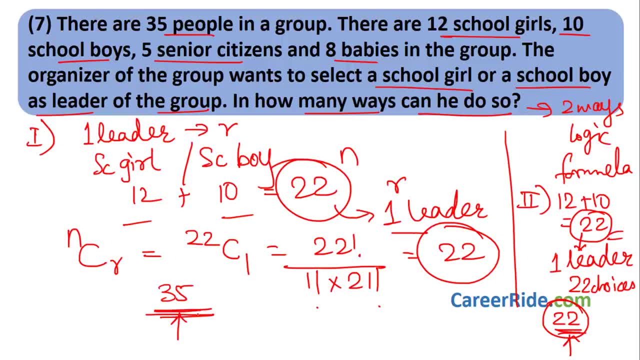 and there is no criteria that school girl should become a leader or school boy should become a leader or a baby should become a leader. they just want one person as leader of the group. so 35 choices are there, but over here we will not consider 35. that was just an extension to explain. 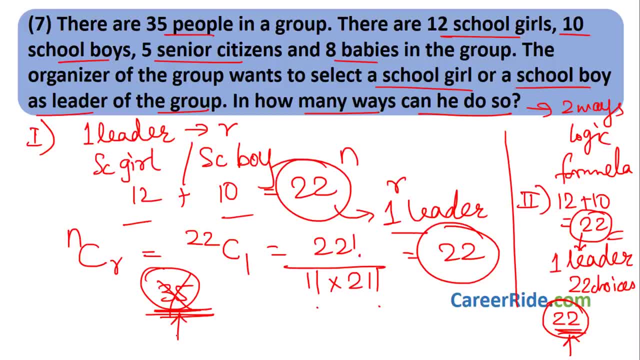 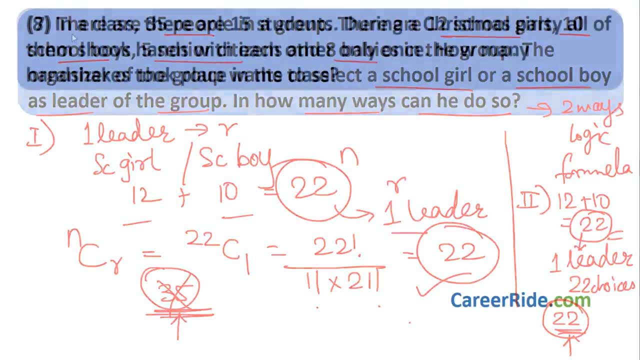 what you are doing over here. we just want that the leader should be school, school girl or school boy. so the answer is 22 ways. moving on to next question, question 8: in a class there are 15 students during a christmas party. all of them shook. 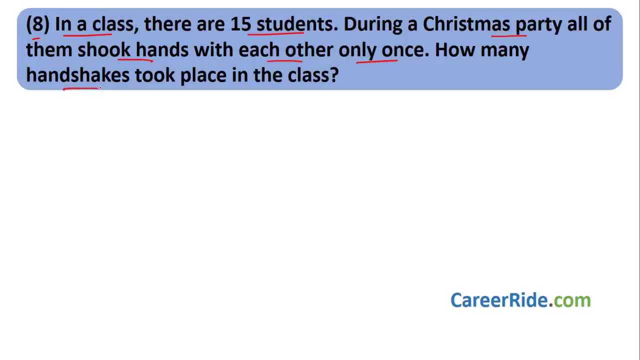 hands with each other only once. how many handshakes took place in the class now? this is one of the most famous examples which are asked in every exam. please remember how to solve this kind of sum. it is extremely, extremely, extremely, extremely easy. okay, this is a permutation combination sum. actually, specifically, it is a combination sum. 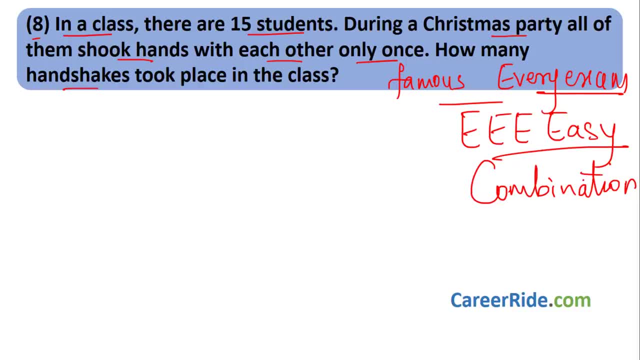 okay, very easy sum and a very easy formula or a very easy trick to solve this sum. i'll also explain in what format this sum can be asked. now over here they are saying that there are 15 students, so total number of students are 15 in. okay, they, each student shook hand with the other person only once only. 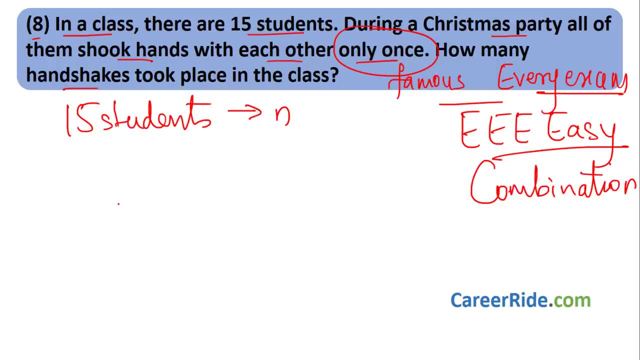 once. this is important. okay, how many handshakes took place in the class? very easy, there are 15 students, okay for an handshake. how many students do we need? we need two students for a handshake, okay. so if you out of 15, select means combination, select two students out of 15. this is the answer. what do we get? 15 x 14. 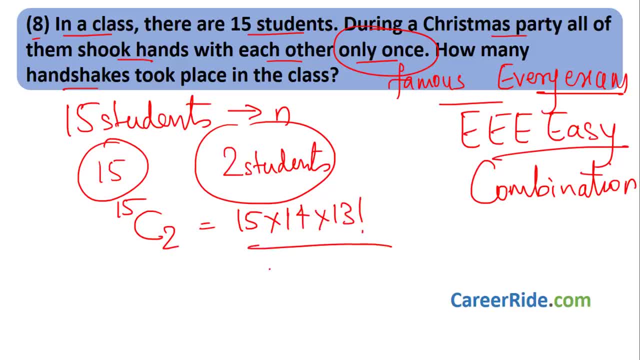 to 14 into 13. factorial upon 2 factorial into 15 minus 2. 13 factorial, that would be 15 into 14 divided by 2: 105.. 105 handshakes take place in the class. Very easy Answer is what? 15.. What is 15?? 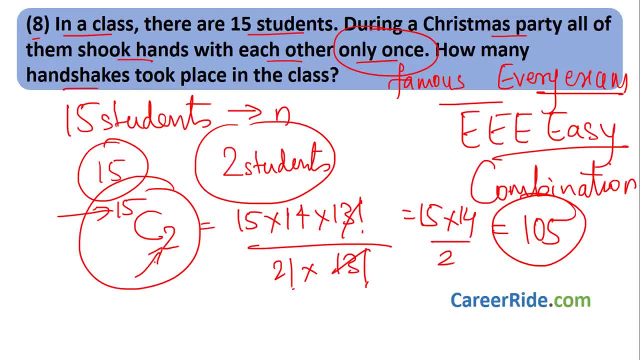 Total number of students. What is 2?? 2 will always be there, Why, For an handshake, 2 people are needed, So 2 will always be there. Only thing changes is this: If they give you, if there are 30 students in a class and they shake hands with each other only once, what will be the answer? 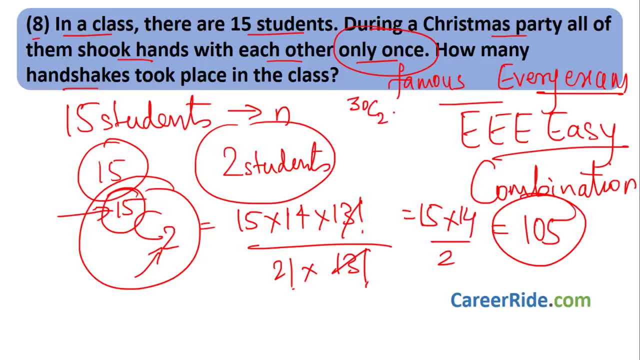 It would be 30 students are there, So 30 C2, and find the answer like this Very easy. Nothing to it, Just remember. answer is 15 C2 or N C2, where N is number of students. Now, in what way can this? 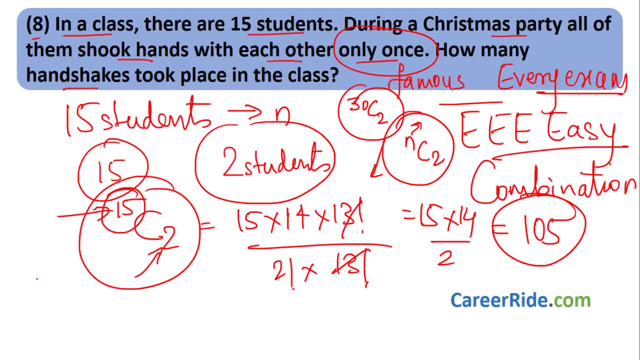 question be asked. They can say that there is a cricket league or a football league and there are say there is a cricket league or a football league and there are say there is a cricket league or a say 9 teams in the football league or the cricket league and each team plays match with other team. 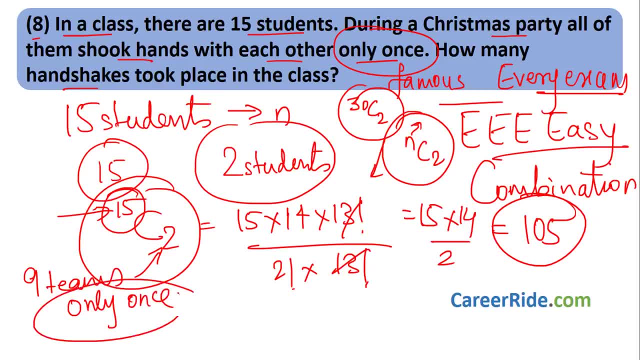 only once. Only once. This is very important. Only once. Then, how many matches are played in the league? Simply, How many teams are there? 9. 9, C2.. This is similar to handshakes For playing a. 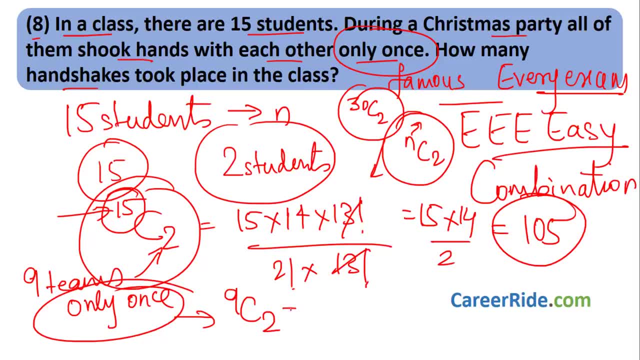 match, 2 teams are needed, So selecting 2 teams out of 9.. 9 C2.. What you will get: 9 into 8.. This is 9 factorial upon. 9 minus 2 is 2 factorial. 9 minus 2 is 7 factorial. That would be. 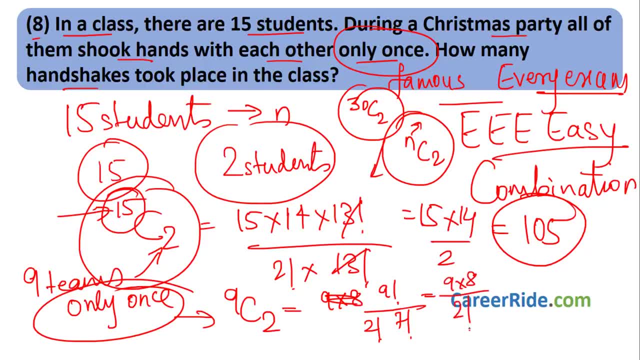 9 into 8, into 7 factorial- That gets cancelled. 2 factorial is 2.. 2, 4, 9, 4 is 36.. 36 matches get played, Very easy. Now again, I will go a little bit further. If they say that in a class there are: 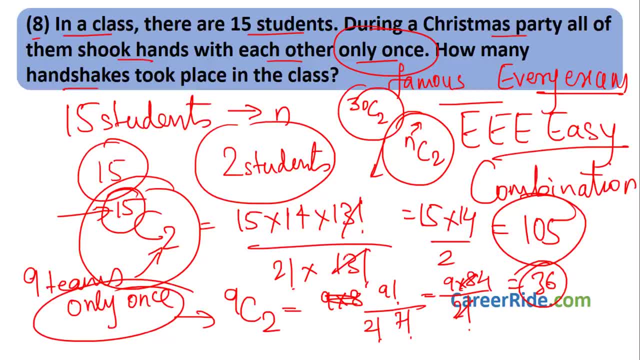 15 students and during a Christmas party, all of them shook hands with each other. Only that much is given. Only once is not given How many handshakes took place, Then what you can say over here is that 105 handshakes take place when each of them shake hands with each other. So this is. 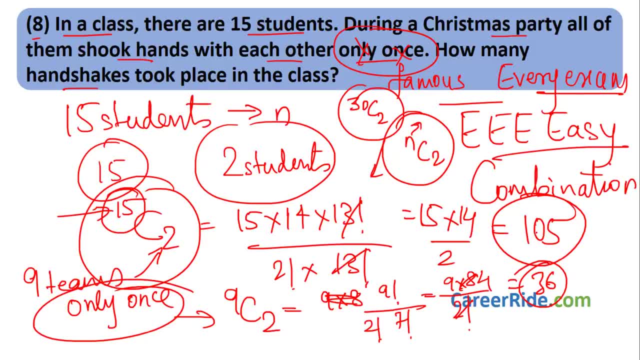 again a simple situation: That all of them is shaking head with the other person only once. But if only once's criteria is not there, then there is a chance that each person can shake the hand twice Because, say, if there is A and there is B, A can shake hand with B, and then, when B's turn, 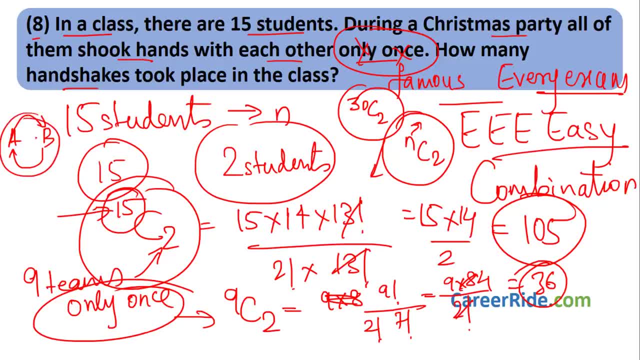 come, B can also shake hand with A, So for both the people 2 handshakes happen. So over here what we can have. We will have 105 when it is only once. Simply multiply by 2. You will get 210.. But 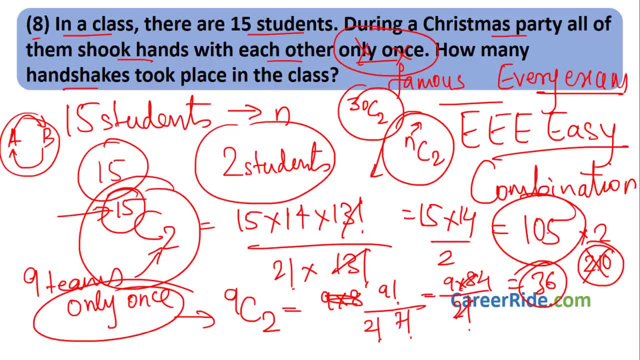 is not asked only. they asked how, how many of them shook hands with each other? only once, okay, only once is there most of the time? go with only once. and the answer is 15 c 2. remember, it is 15 c 2, n c 2, very, very easy. moving to next question, a bank has six digit account number with no 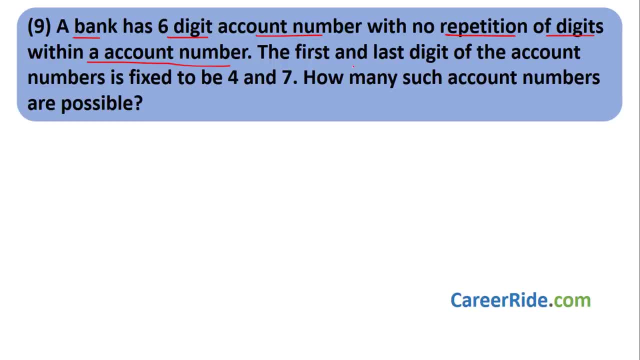 repetition of digits within a account number. the first and last digit of the account numbers is fixed to be four and seven. how many such account numbers are possible? very, very easy some. let us take a look. account numbers are six digits, okay, four, five and six. out of that they 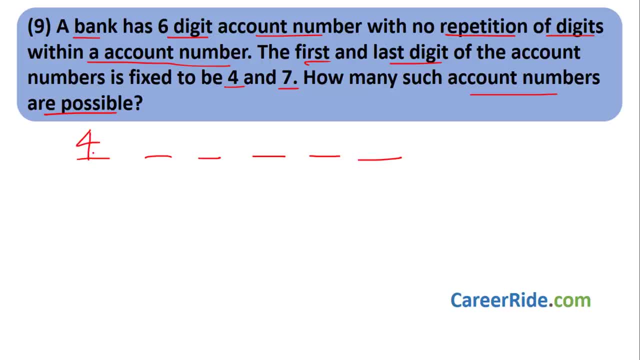 have given. first and last digit of the account number is to be four and seven compulsorily, so these are completely useless for us. why? because first and last digit is fixed, so we have no choice. so just consider only the middle four digits. what have they said is that there is no repetition of 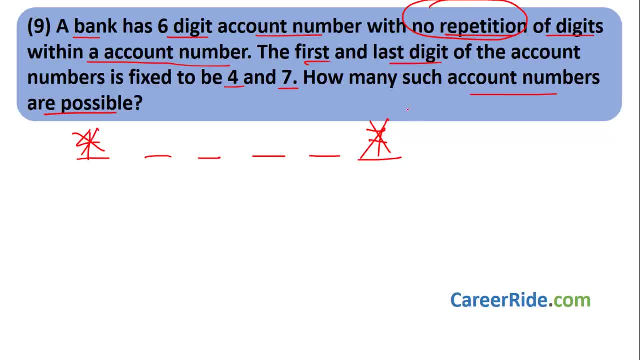 digits, right, how many digits are there in mathematics if we see single digit numbers, how many are there? there are, since it is a six digit number. single digit numbers are ten. how zero? one, two, three, four, five, six, seven, eight and nine. okay, out of that, four and seven already been used and since there is no repetition, we 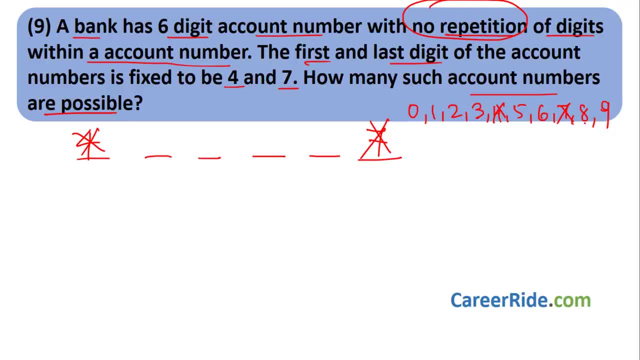 cannot have four and seven over here. how many are left out of these ten when we remove these two? how many are left? eight are left. so here we have eight choices. correct the second digit. have the second digit of the account number. we have eight choices over here. 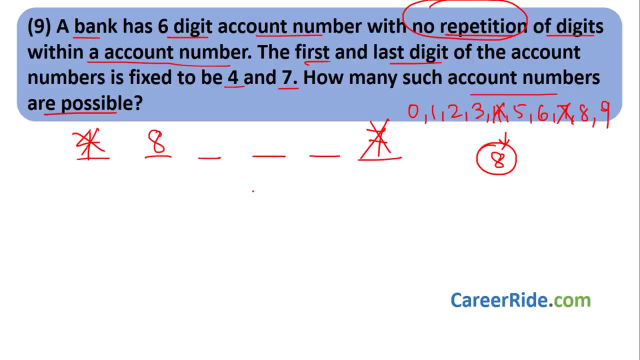 zero, one, two, three, five, six, eight, nine. out of that, again one digit gets over over here at the second digit. okay, so how many choices are left over here? eight minus one, seven choices are left. okay, again one digit gets over at this place. so how many choices are left? only six digits are left. 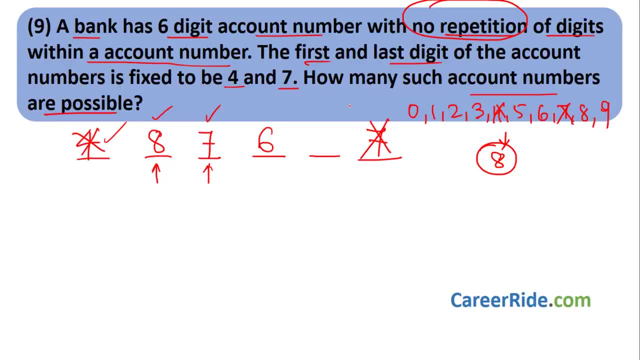 because why six? because out of ten here, one digit is taken here. one digit is taken here. one digit is is taken here. one digit is taken again this place. okay, five digits are already taken. how many are left now? how many choices are there? out of five, we have to choose a digit. so what is? what are the? 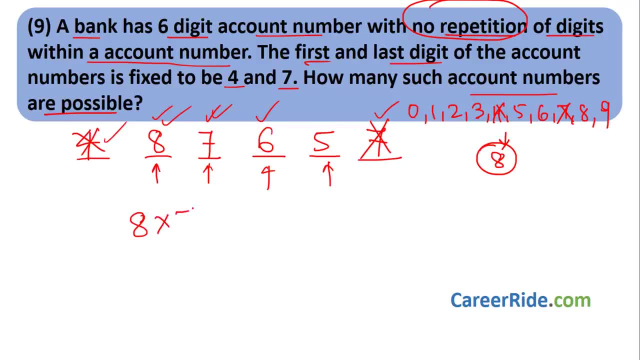 total possibilities or possible account numbers: 8 into 7 into 6 into 5 would be equal to 8. 7s are 56, 6, 5s are 30. that would give us 1680 account numbers. okay, 1680 account numbers are possible. 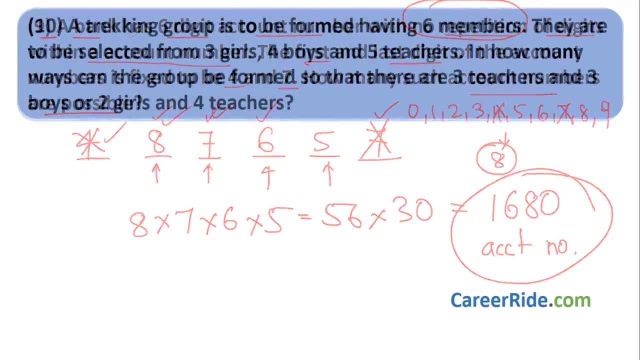 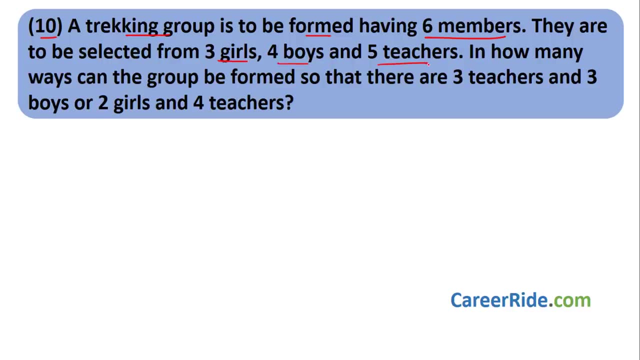 with the given conditions. moving to question number 10, a trekking group is to be formed having six members. they are to be selected from three girls, four boys and five teachers. in how many ways can the group be formed so that there are three teachers and three boys, or two girls and 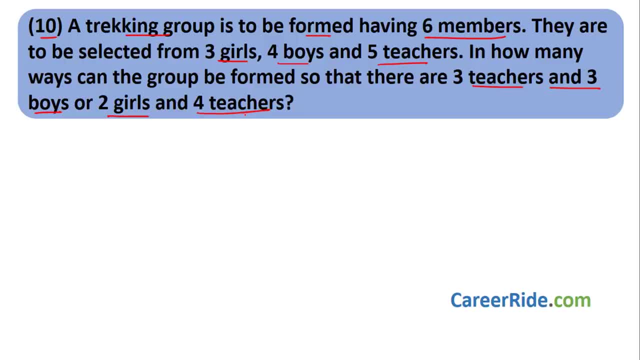 four teachers. so there are. they are giving us two options, like there are two kinds of groups that are to be formed. okay, what they are saying is that the group which is to be there, it can either have three teachers and three boys- okay, or you can have a group which has two girls and four teachers, right, see in. 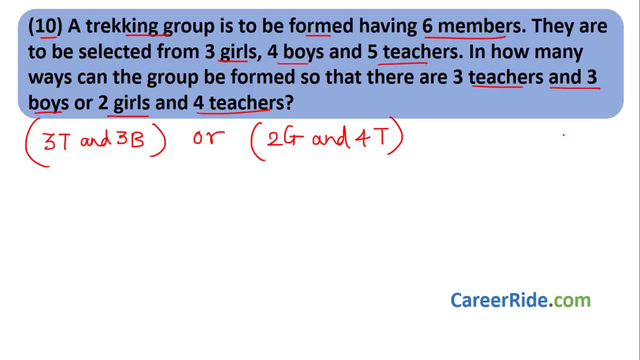 probability. we have in the probability video. if you have not seen, please take a look at that. over there we learned a very, very easy concept and very small concept. please remember it. it is useful and means multiply or means addition, that is, add. okay, if you remember this, you will. 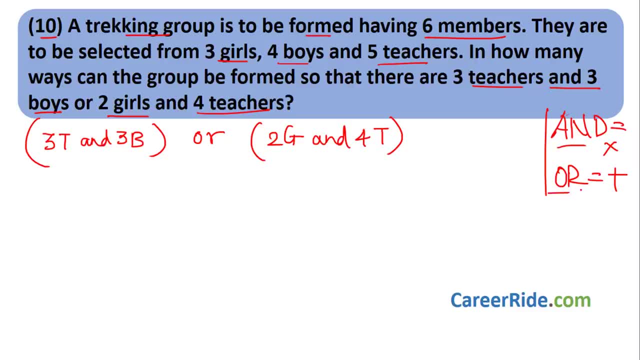 very easily be able to solve this sum using formula and this basic concept and means to multiply or means to add. okay, now over here, we want either three teachers and three boys, or we want two girls and four teachers. now, how to select three teachers? okay, we want. how many teachers are there? there are. 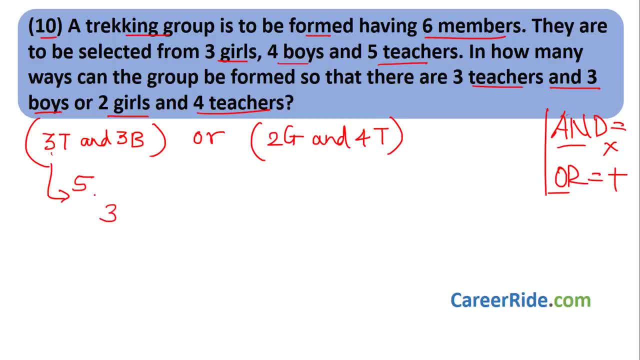 five teachers. out of that we have to select three teachers. select means combination five factorial upon 3 factorial into 5 minus 3 is 2 factorial. That would give us 10 ways to select 3 teachers. Then 3 boys are there. How to select 3 boys? How many boys are there in total? 4 boys out. 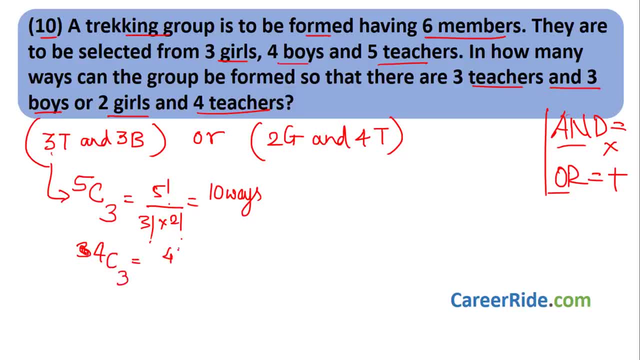 of that we have to select 3 boys. Select means combination, 4 factorial upon 3 factorial into 4 minus 1.. 4 minus 3 is 1 factorial. That would be equal to 4 ways And we know that we have 3 teachers and 4 boys, So 10 ways. and and means multiplication 4 ways would. 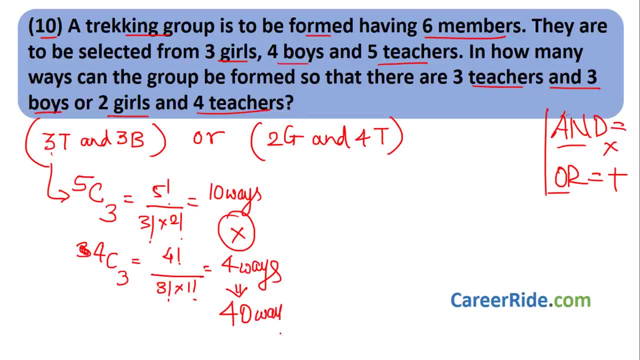 give us 40 ways. Now this is or Or means addition. We have 40 ways over here. Or means addition. We want to select 2 girls. How to select 2 girls? How many girls are there? 3 girls Out of that? we need to select 2 girls. Select means combination: 3: factorial upon. 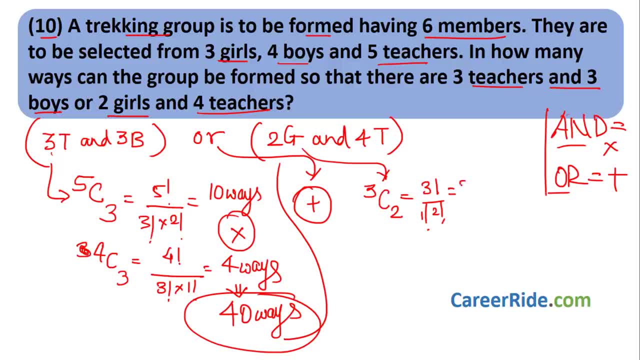 3 minus 2 factorial is 1 factorial into 2 factorial. We will get answer as 3.. Then these are 3 ways. We also want 4 teachers out of 5 teachers. So 5 teachers are there. Select 4 teachers. That would give us again the answer would. 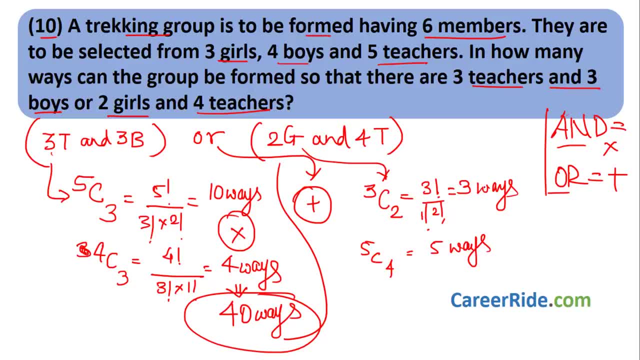 be 5 ways. So select 2 girls and select 4 teachers. So total number of ways would be 3 into 5 ways 15 ways. So in 40 ways we can select 3 teachers and 3 boys. Or we can go for 15 ways, which where we select 2 girls and 4 teachers And or means. 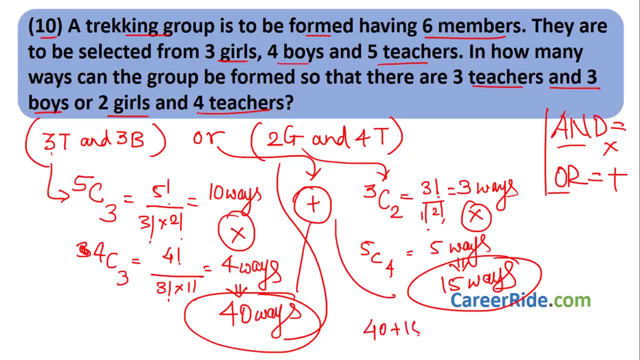 addition. So add these 2. What do we get? 40 plus 15, equal to 55 ways, is the answer. See how easy. it is Very, very easy, Just remember. and means multiply Or means addition. This would be useful in probability also. And means multiply Or means addition. Moving to question, 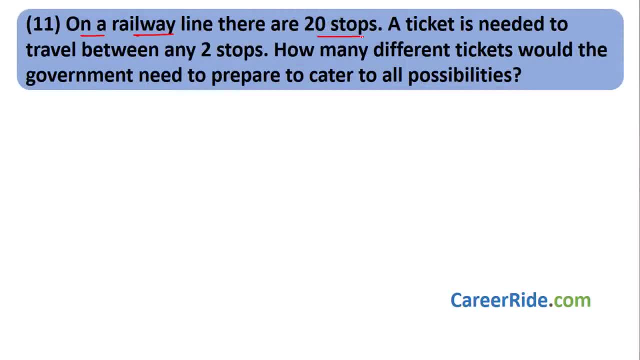 number 11.. On a railway line there are 20 stops. A ticket is needed to travel between any 2 stops. How many different tickets would the government need to prepare to cater to all possibilities? Very, very easy. Let us see, This is a railway line. This is the start. 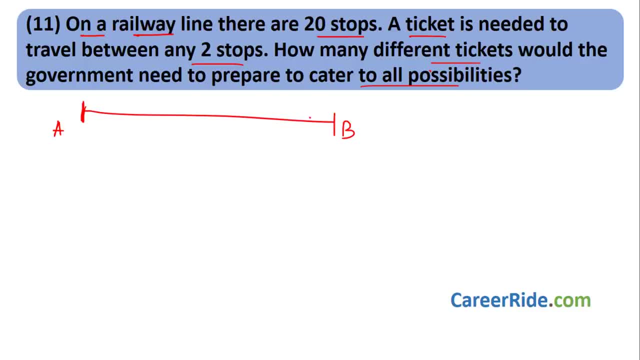 point A: This is the end. point B: This is the first stop. This is the 20th stop. So 2nd, 3rd, 4th, 5th, 6th, like this: There are 20 stops. If you want to go between any, 2. 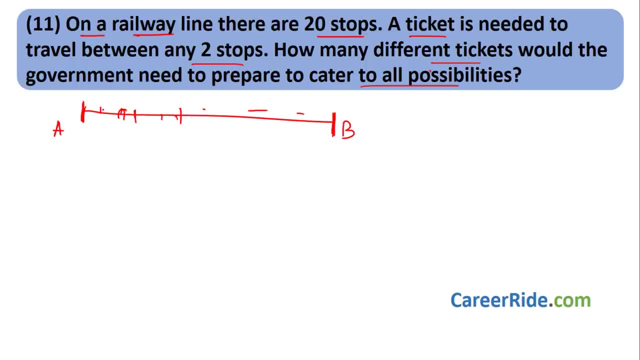 stops like this to this, Or say Year to year, Or even year to year, Then you need a ticket. So how many different type of tickets would the government need? Very easy to find out. How many stops are there? 20 stops are there. Now, if you want to travel between 2 stops, If you need a ticket, A ticket. 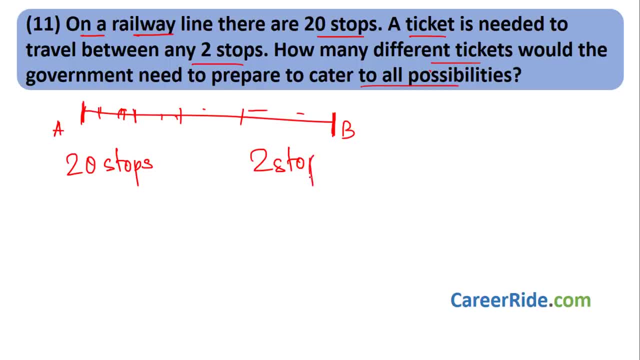 is between how many stops? 2 stops. If you want to travel from 1st stop to the 2nd stop, or 1 stop to other stop Or 1 stop to 2nd stop, Then you need, Then you need a ticket. So ticket is needed for between any 2 stops. So that means it. 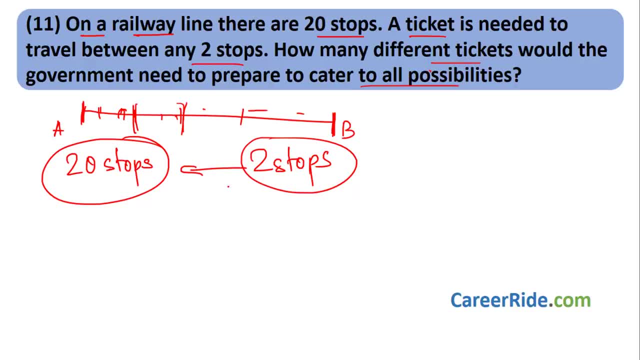 is simply: we have to select 2 stops out of 20 stops. This is R, This is N. Select means combination: Select 2 stops out of 20 stops. What is that? This is 20 factorial upon 2. factorial into 18. factorial. 20 into 19 into 18. factorial divided by 2 factorial into 18. 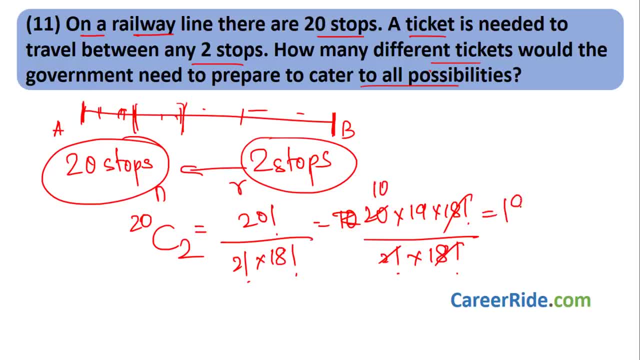 factorial. This gets cancelled. 10. 190 possible tickets. But this is not the answer. Now you will say why. Because this 190 is when we are starting from here, When we are going from here. Now, if say this and this, You want to travel from here to here, You will 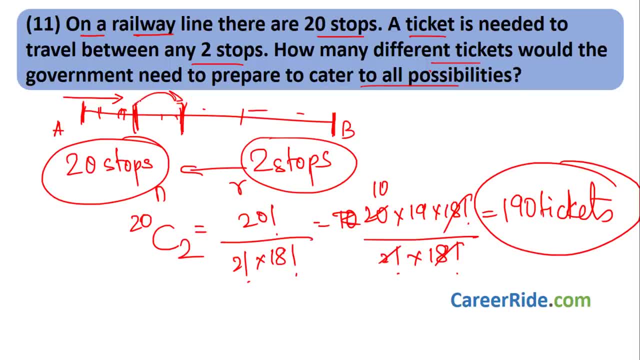 buy a ticket, Will you use the same ticket to travel from here to here? No, If you want to travel from this stop to this stop, there will be a separate ticket for this. So 190 tickets are from one side, while travelling from one side, Again, while travelling from. 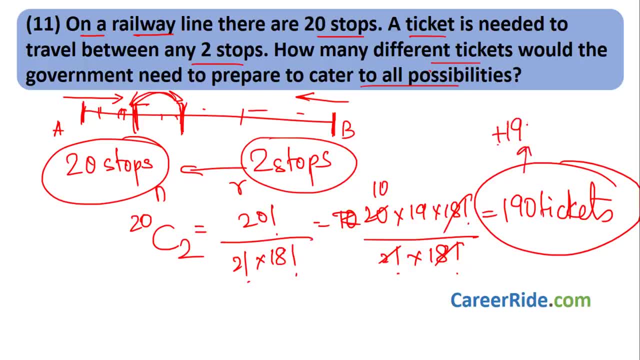 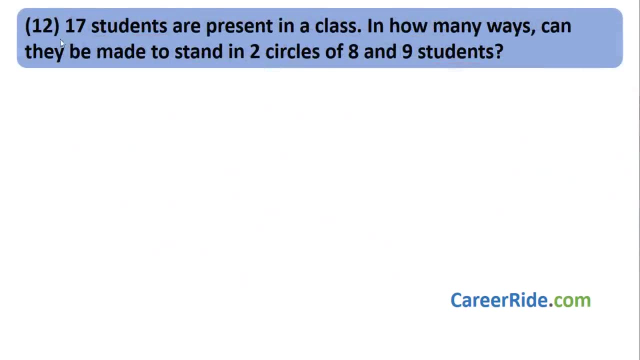 other side we will have same plus 190 tickets. That would be 380. is the answer 380 possibilities? are there 380 possible tickets are to be made by the government. Moving to the next question, 17 students are present in a class. In how many ways can they be made to stand? 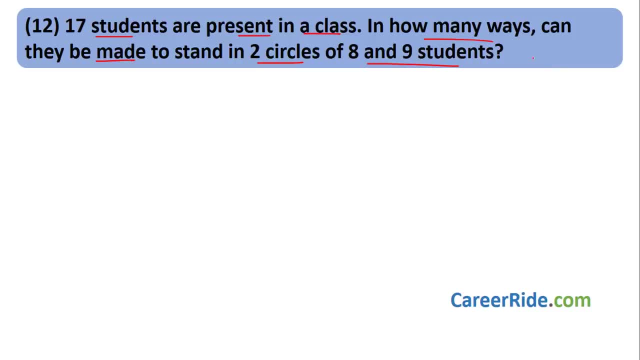 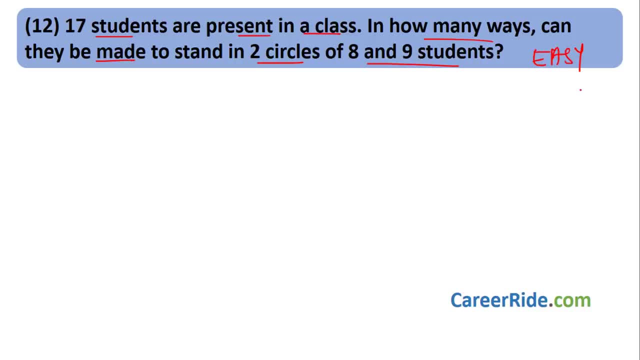 to explain over here. The first thing is that here the students are not made to stand in a straight line, They are made to stand in a circle. and the second thing is that we already know that if we have n things, if we want to arrange them in a circle, that can be done. 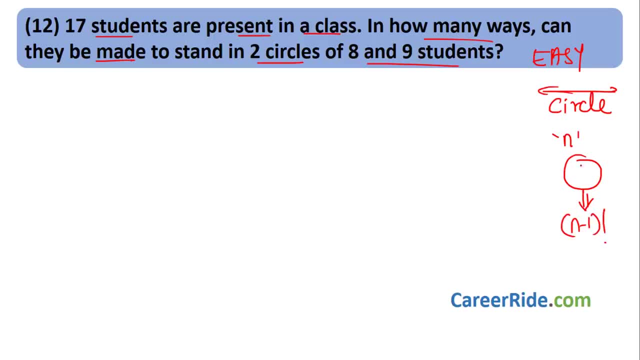 in factorial. If you want to arrange them in a straight line, we do it in factorial ways. If you want it in a circle, we can do it in bit. ooh, We can do it in bit, ooh, let, we can do it in n minus 1 factorial ways. okay, very easy, let us see how to solve this sum. 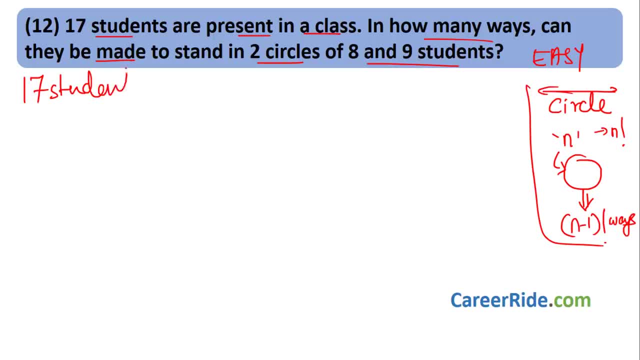 there are 17 students, okay, and we need two circles. okay, two circles, one of nine students, one of eight students, right, 9 plus 8 is 17. that means that what we'll do is: first we'll select nine students out of 17 and arrange them, and the remaining students will arrange over here. 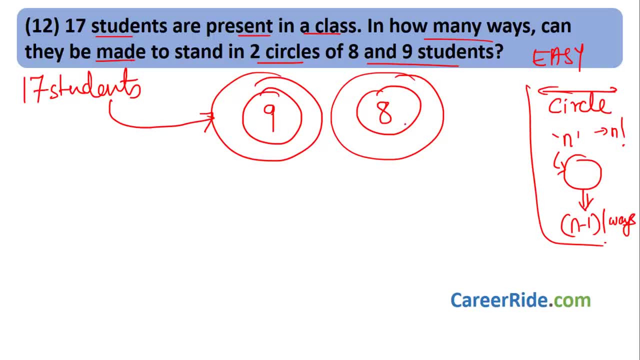 as remaining are eight students only. we can arrange it in this circle. so, first, what we need to do? select nine students. select means combination. we have to select nine students. out of how much? 17 students. what do we get? 17 c 9. okay, let's not solve it right now. okay, this is 17 c 9. that is we. 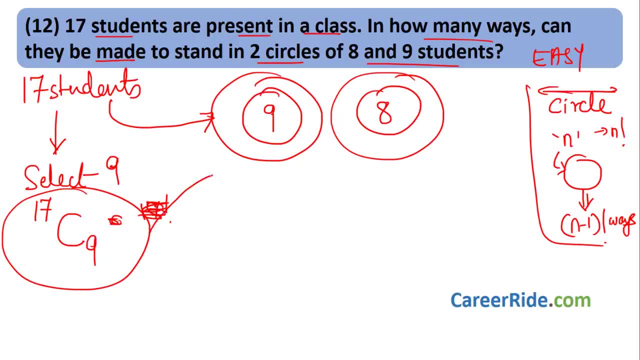 have selected these nine students. now these nine students will be arranged in a circle. in how many ways? very easy, n minus 1. so 9 minus 1 factorial would be 8 factorial ways, correct. so these students would be arranged in 8 factorial ways. right now, how much these students are remaining: 17 minus 9 is 8. 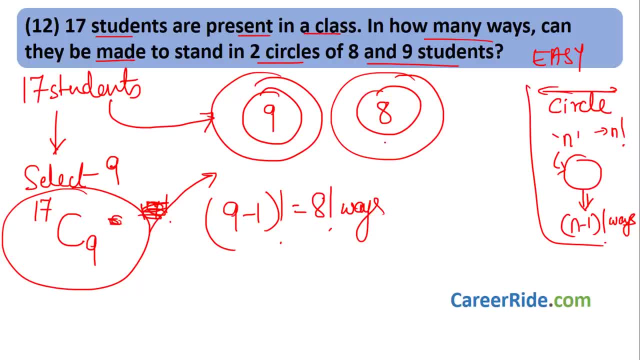 these 8 students will form a circle of 8- okay, which they have given. okay, the second circle. these 8 students would be arranged in how many ways in a circle? 8 minus 1 factorial ways, that would be 7 factorial ways. so what are the total number of ways? 17. 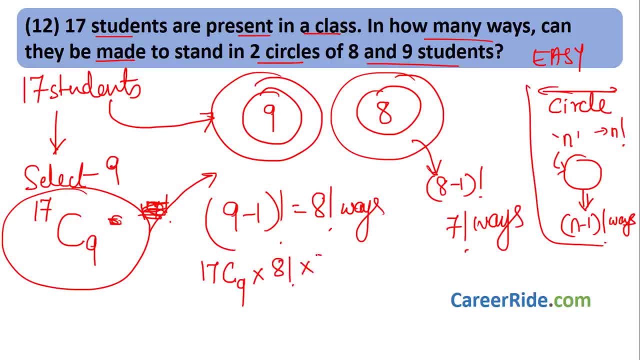 c: 9 multiplied by 8 factorial, multiplied by 7 factorial. you can keep this as answer or you can simplify it as 17 factorial divided by 9 factorial into 8 factorial, into 8 factorial, into 7 factorial. so you get this: you will have 17 factorial into 7 factorial, divided by 9 factorial. okay, now, when there are values like this. keep the answer like this. only don't try to calculate, because 17 into 16, into 15, into 14, into 14, into 15, into 7, and to the from bottom right corner, you will get K 9, and so it would be 15 factorialHHHH. 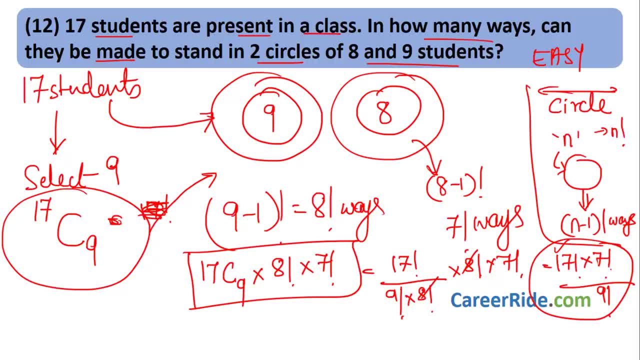 like this. only don't try to calculate, because 17 into 16, into 15, into 14 would be really huge. so in options you will get similar kind of answers. okay, similar kind of option. so tick the appropriate option now if the we can do it other way also, we can have 17 students and we can select. 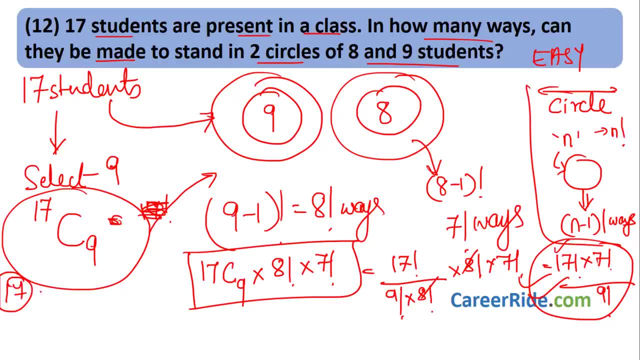 8 students. let us see we have 17 students and we'll select 8 students first and arrange them in a circle. selecting 8 students is 17, c 8. okay, arranging them in a circle is 8 minus 1 is 7, factorial. how many students remain? 17 minus 8 is 9. this is 17. 17 minus 8 is 9. these 9 students can. 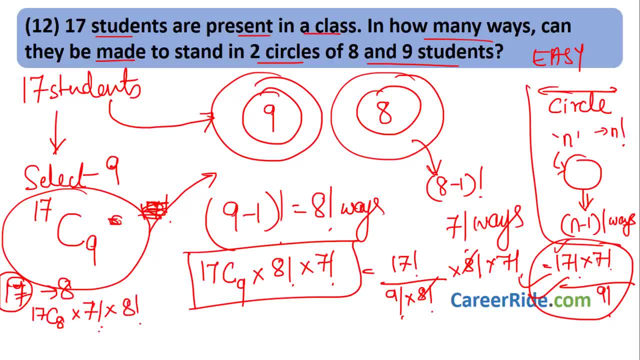 be arranged in a circle in 8 factorial ways. right, so what is the answer? we'll get 17 factorial divided by 8 factorial into 9 factorial into 7 factorial into 8 factorial. same as this. okay, so we'll get the same answer as this. now over here, what is happening is that the students are to be 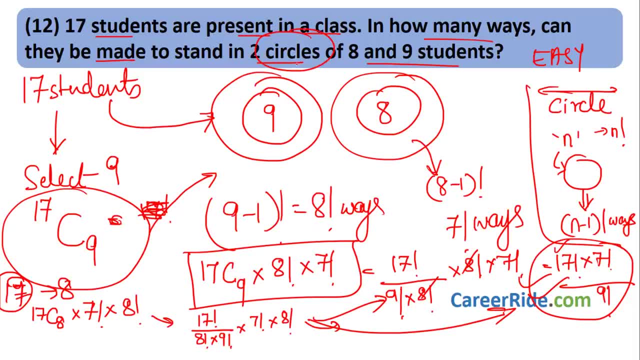 arranged have to be arranged in a circle. right, two circles had the students been to arrange. if they say that take 17 students and arrange them in a straight line, you can directly use the permutation formula. what is the permutation formula? npr is nothing but n factorial upon n minus r factorial. 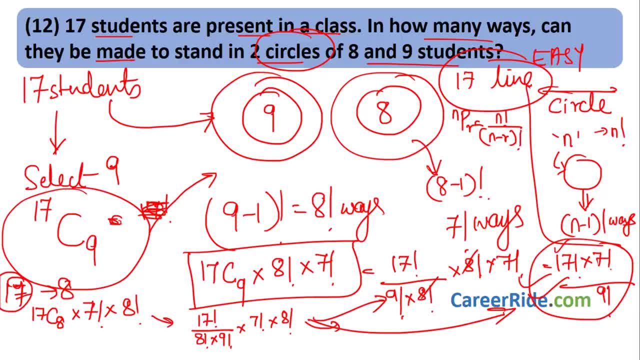 right. permutation formula is derived from combination formula. right, we have n factorial upon r factorial into n minus r factorial, and arranging is r factorial, so r factorial gets cancelled and we get this formula. so what we can do is we'll have npr equal to n factorial upon n minus r factorial. okay, so if we 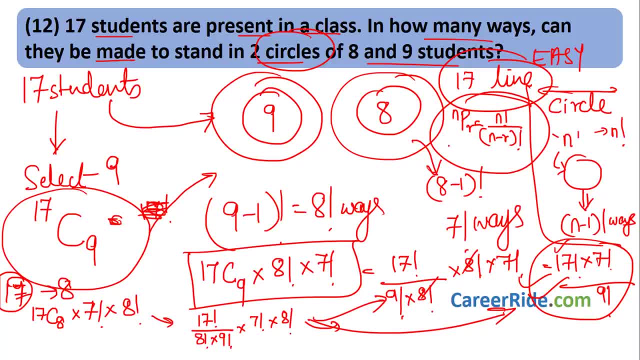 have to arrange two. if you want to arrange students- 17 students- in two lines of 8 and 9 students- then what we'll do? we'll simply take this permutation formula. okay, let's solve over here. so we'll have n factorial at the bottom. we'll take this formula: 17 students are there, we have to arrange it into. 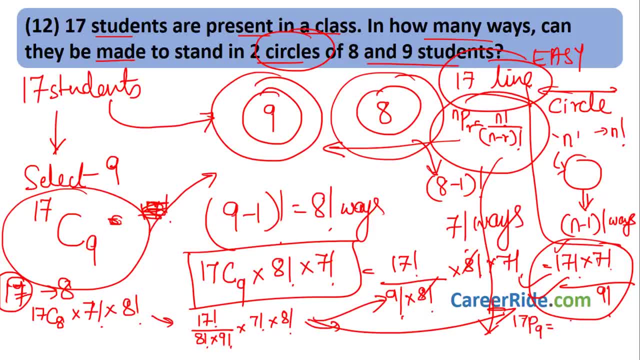 two, two lines. so let us assume we select nine students first. okay, so we'll have 17 factorial divided by 17 minus 9 is 8 factorial. okay, this is the arrangement of nine students in single line. now, arrangement of eight students in single line is 8 factorial. this gets cancelled. answer comes. 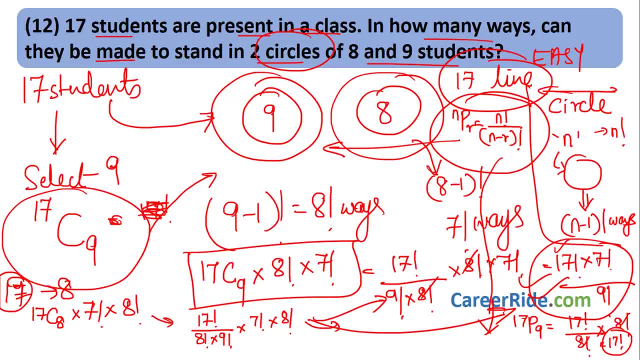 out to be 17, factorial. okay, so we can use permutation formula also if we have to arrange it in a single line. but here we want a circle. so what we did, we just selected and then arranged in circle. selected, arranged in circle. okay, very easy, most of the 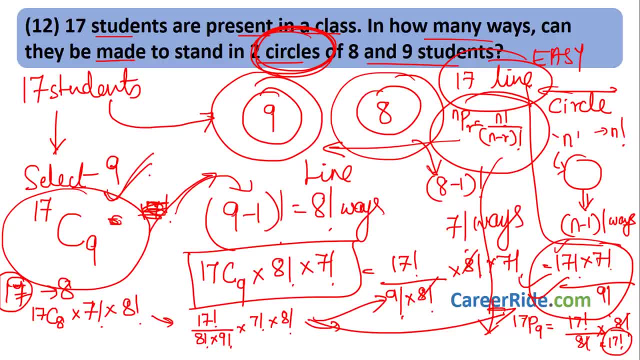 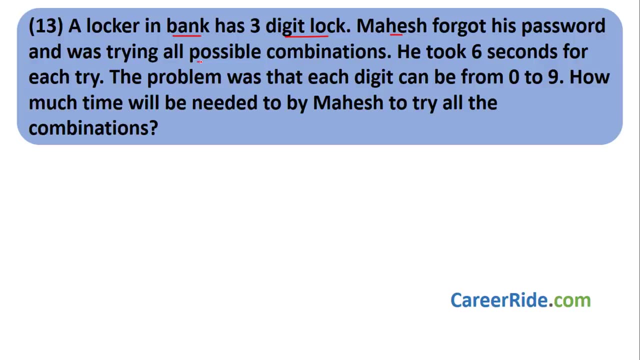 permutation sums. you can solve by selection and then arranging. okay, that would become easier and logical if you are not able to remember the permutation formula. moving to next question, a locker in bank has three digit lock. mahesh forgot his password and was trying all possible combinations. he took six seconds for each track. the problem was that 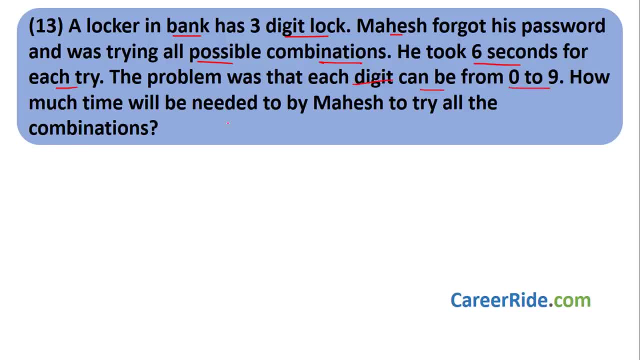 each digit can be from 0 to 9. how much time will be needed by mahesh to try all the combinations? okay, now here they have given each digit can be 0 to 9. that means repetition is allowed. okay, repetition is allowed. it has a three digit lock, okay, and each of the digit can be from 0 to 9. 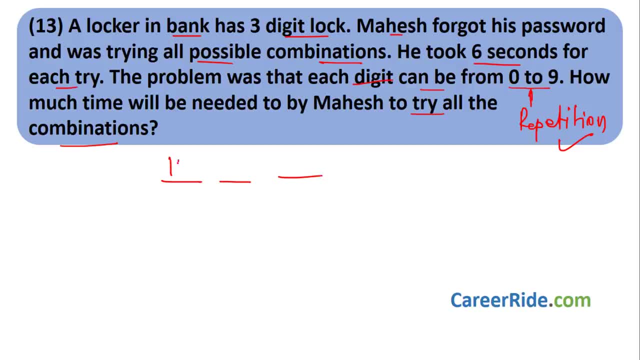 that means there are 10 possibilities. 0 to 9 are 10 digits, so 0 to 9 can come over here anything. 10 possibilities, again 10 possibilities, again 10 possibilities. how many are the total possible combinations? just multiply 1,000 combinations are possible for. 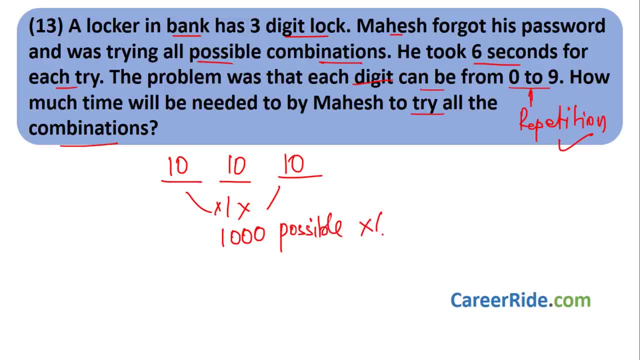 each combination, mahesh takes 6 seconds. so total seconds taken: is each possible combination: 6 second? okay, thousand are possible, so he'll take 6,000 seconds. that is nothing but divided by 60 what you will get 100 minutes, right? so mahesh will take 100 minutes to try all, to try all the combinations. moving to next question, 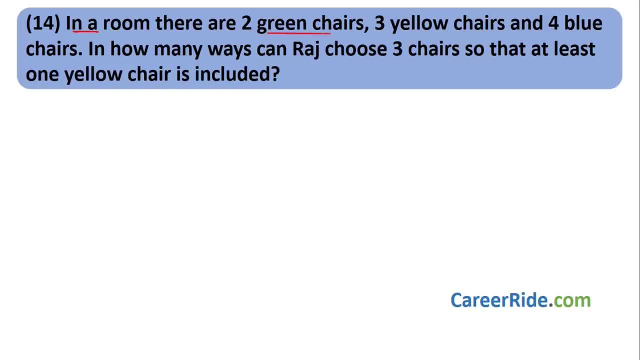 in a room there are two green chairs, three yellow chairs and four blue chairs. in how many ways can Raj choose three chairs so at least one yellow chair is included- again very similar to some, to what we had seen in probability as well as earlier here on. here they have given what Raj needs to. 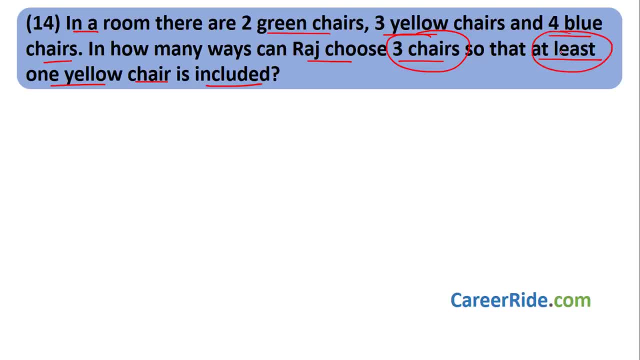 choose three chairs. so he will take 100 minutes to try all the combinations. moving to next question: chairs. and at least one yellow chair should be there. at least one yellow chair means what. at least means there can be one yellow chair or two yellow chair or three yellow chairs, so you can find out. 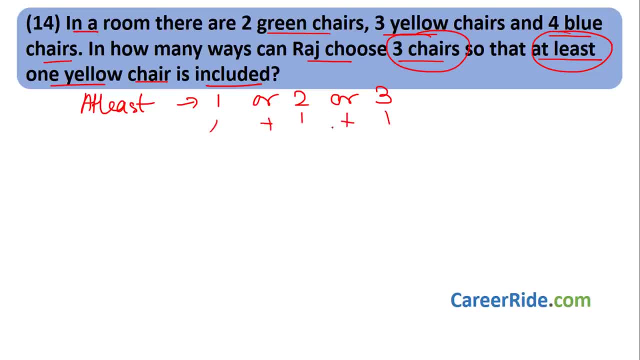 the combination for all these, and then we can add, or you can do another method. what is it? total ways are nothing but choosing yellow chair, okay, choosing at least one yellow chair plus choosing no yet to choosing no yellow chair. okay, choosing one yellow chair, okay, and choosing plus choosing no yellow chair. so what is at least? what are the number of ways for choosing at least one yellow chair? that would be total ways, minus choosing no yellow chair. what are the total ways? what are the total chairs over here? there are two green, three yellow and two green plus three yellow plus four blue chairs. that will four plus seven. total nine chairs are there. so what is the number of ways for choosing at least one yellow chair? that would be total ways, minus choosing no yellow chair. what are the total ways? what are the total chairs over here? there are two green, three yellow and two green plus three yellow plus four blue chairs. that will four plus seven. total nine chairs are there. so what is the number of ways for choosing at least one yellow chair? that would be total ways, minus choosing no yellow chair. what are the total ways? what are the total chairs over here? there are two green, three yellow and two green plus three yellow plus four blue chairs, that would four plus seven. total nine chairs are there, so what is the number of ways for choosing at least one yellow chair? 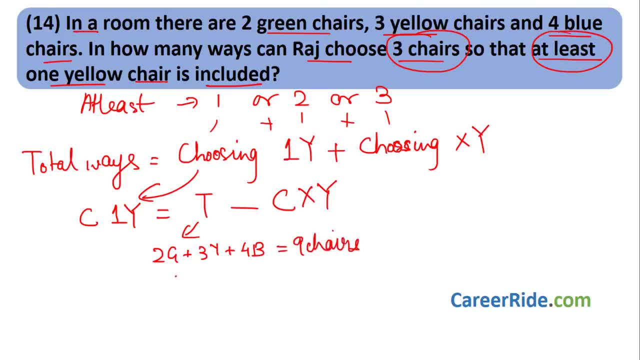 how to choose three chairs from nine chairs? very easy. select means combination: select three chairs from nine chairs. that would be 9, factorial upon 3. factorial into 6. factorial that is, 9 into 8 into 7. divided by 3 into 2, this comes out to be 4, 3, 84 ways. okay, these are the total number of ways. 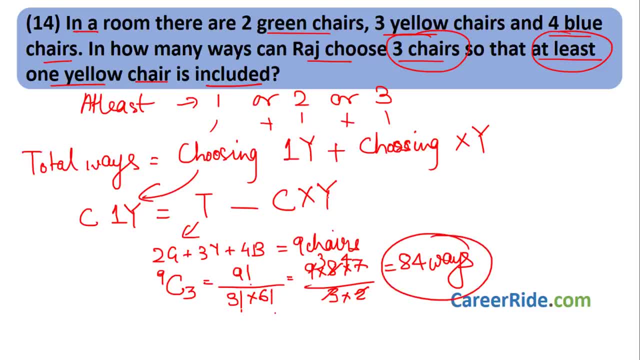 84 are total number of ways, now, how many ways in which we can choose not a yellow chair, or we should not choose even a single yellow chair. how many non yellow chairs are there? two green and four blue, that is six non yellow chairs. are there? non yellow chairs are there? out of these six, we 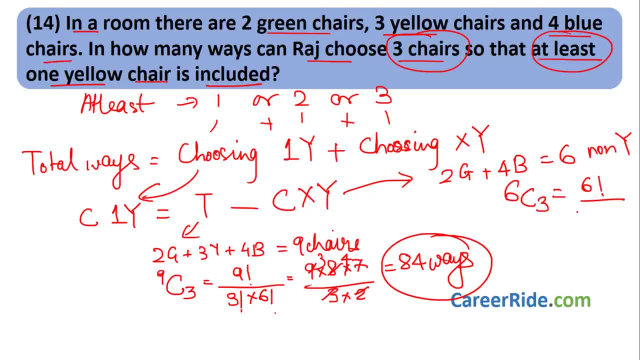 have to choose three chairs: six, factorial upon three, factorial into three. factorial that would be six into five, into four upon three, into two. two, twos are three, twos are 20 ways. okay, so in 20 ways we can choose a non yellow chair. so total number of ways in which we can choose at least one yellow chair: 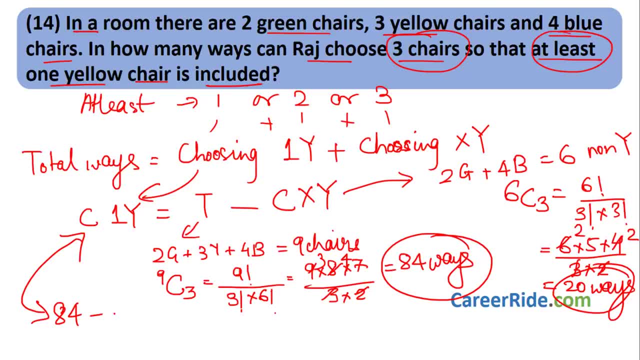 is nothing but total ways, minus ways for choosing no yellow chair, 64 ways is the answer. see how easily, by using this method- which we have seen in probability also and right now, in few sums before few sums also, we have used this technique- we can solve the sum moving on to. 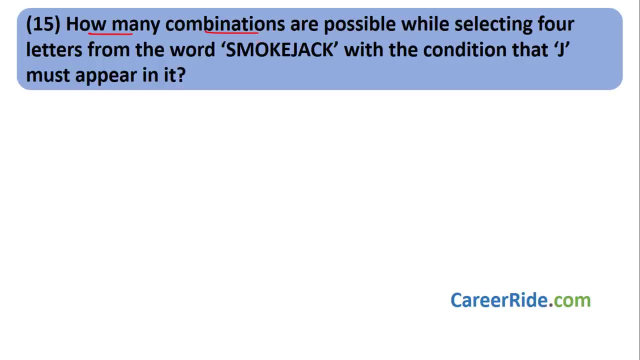 question number 15: how many combinations are possible while selecting four letters from the word smoke jack, with the condition that j must appear in it again? very easy sum. let us take a look how to solve this. what are they saying? we want a four letter word or we have to select four? 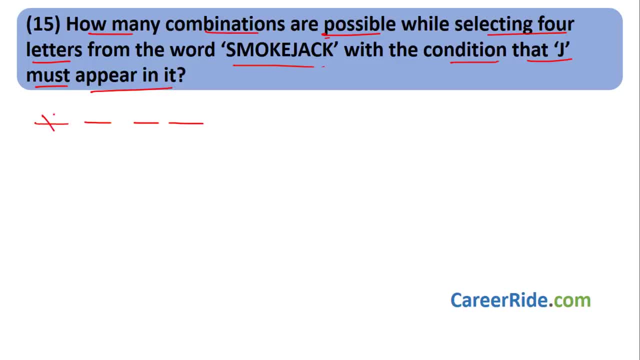 letters. out of that, j has to appear. that means one place is already occupied by j. okay now, so we have to select only three letters also out of smoke jack. j already has occupa has been occupied, so we cannot select j again. so what are we left with smoke ack- okay. 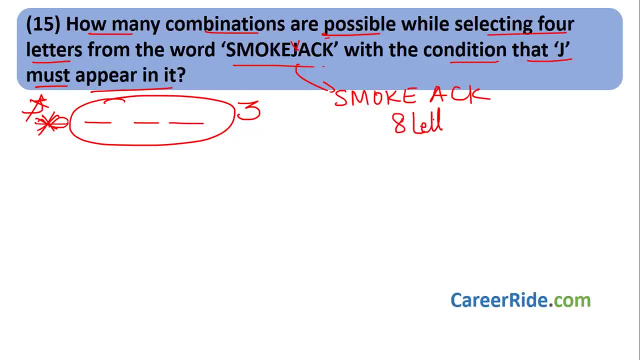 so we are left with five, eight, eight letters. we are left with eight letters. out of that, k is repeated twice. okay, k comes two times right now. what to be first? okay to be. after that, j three, j two, j okay to be there. so we need to silicon, we need to silicon, okay, و. 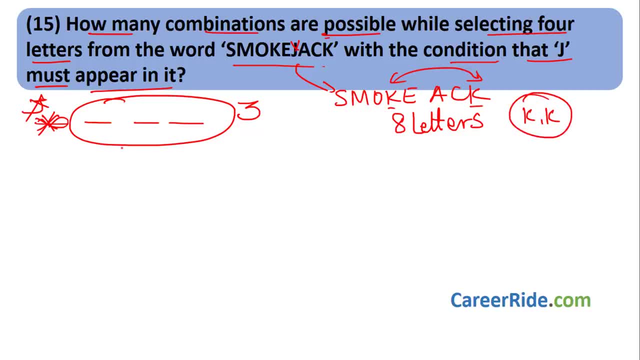 Now we have got the three letter letters out of that j. j has to occupy two letters out of that j has to occupy in. so we are left with five, eight, eight letters out of j to do. now we have to select three letters. there are three possibilities that can happen. what can? 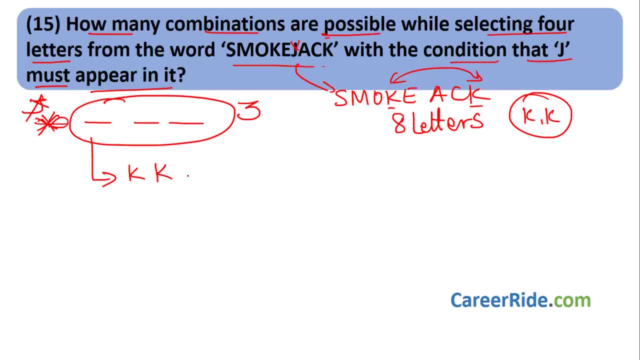 happen is that you can have both the case and you just need one letter over here. you can select two case and you just need one letter over here once you select two case. so these two case will go out of commission. we cannot select them. how many are left? one, two, three. one two three, four, five and 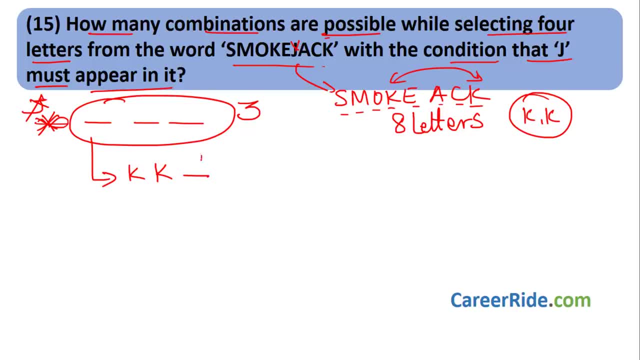 six. out of these six, one will come over here. that means there are six choices, or we can write this: six has nothing but select one letter from six possible combinations. correct, right. what is the second possibility? that you include only one? k. okay, at any of these places, you include only one. 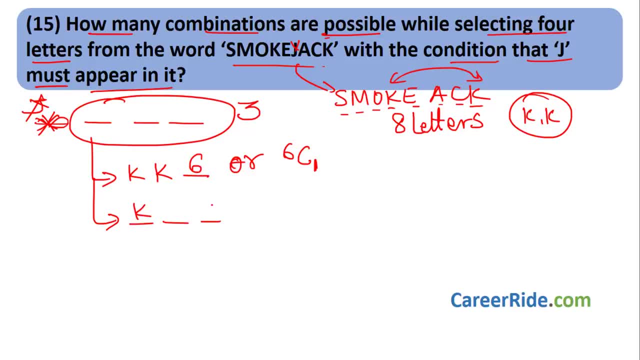 k. now you need not include k over here or over here, because it is not selection and arrangement. it is only selection of four letters. so you can select k for any of the place. it doesn't matter, okay, only select means combination. right, we select one k and these two places can be filled in. how we have to fill. 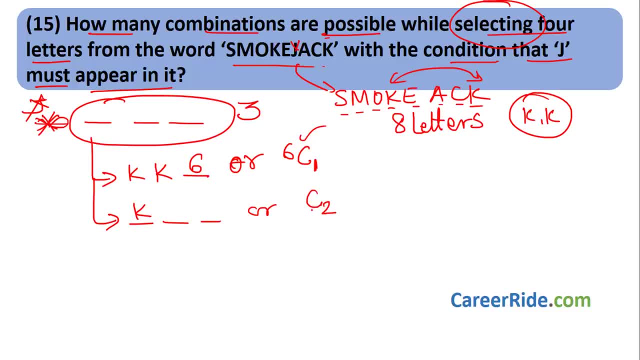 two places and we have to select these characters from where? from the remaining six, because we are here considering only one k. we are not going to select the other k, so we will not consider the other k over here in the six. okay, these six will only include s, m, o, k, a, e, a and c, these two k's. 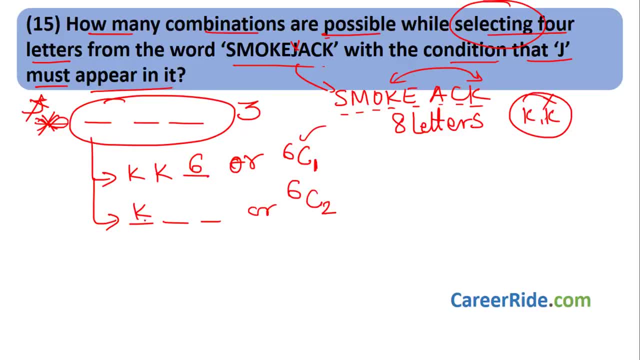 will not be included out of that. out of the two case we have already included, one other one will not include. that possibility has already been covered over here. okay, so these two can be filled in six c two ways. okay, what is the third possibility? this is the first possibility. 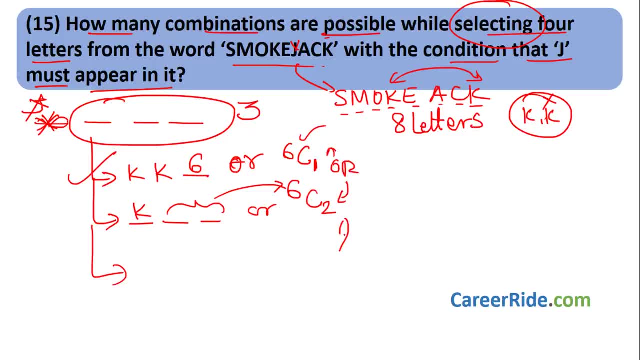 or this is the second possibility, or okay, or the third possibility is what? do not consider k at all. okay, how to fill these three places using six characters, three places selected from six characters. why should we not include these k, two k, because we have tried to include these. 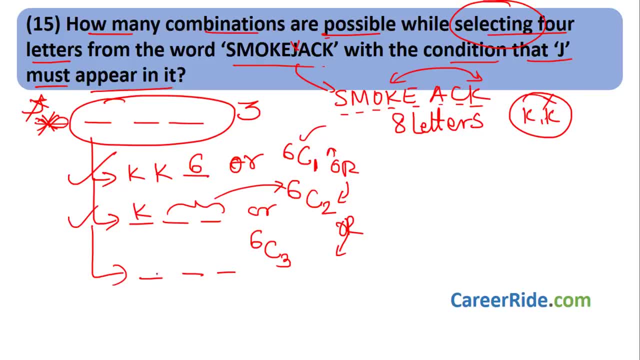 possibilities over here. so over here we are considering a possibility where k is not included at all. okay, so without including k, how many letters are there? six out of six. you have to select three. so what are the total possible ways or total possible combinations: six c, one or we can have. 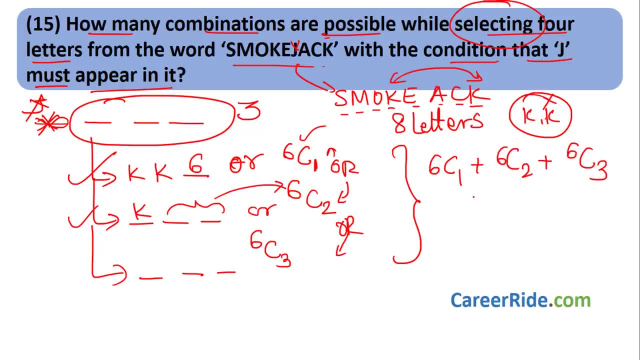 six e two, or we can have six c three. this is nothing but six factorial upon one, 4c3 characters factorial multiplied by 5 factorial plus 6 factorial upon 2 factorial into 4 factorial plus 6 factorial upon 3 factorial into 3 factorial, This would be 6 plus 15 plus 20.. 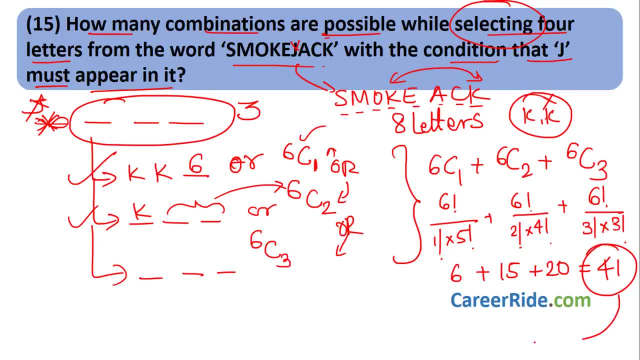 That would be 41 ways. it is possible to have j while selecting 4 letters from the word smoke jack. See, we do not need any more formula, just know the combination formula, just use simple common sense and we can solve the sum. You need to remember that permutation and 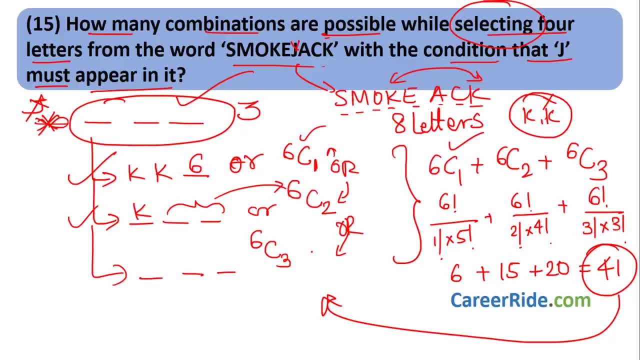 combination is not a tough topic. You just need to remember the formula and little bit of logic. you will be able to solve the sums. also, if there are n things we need to, we can arrange them in a single line in n factorial ways If we want to arrange them in a circle. 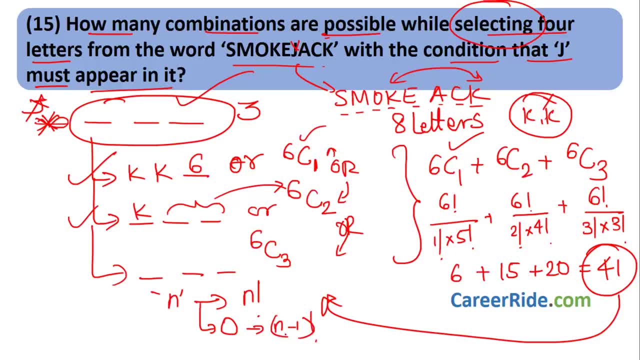 we can do it in n minus 1 factorial ways. very easy formula for combination is what n, c, r is, since we have n, so n factorial. here. we have r bottom, so we have r factorial and n is greater than r, so n minus r factorial. Combination also means to select. Now, permutation means if: 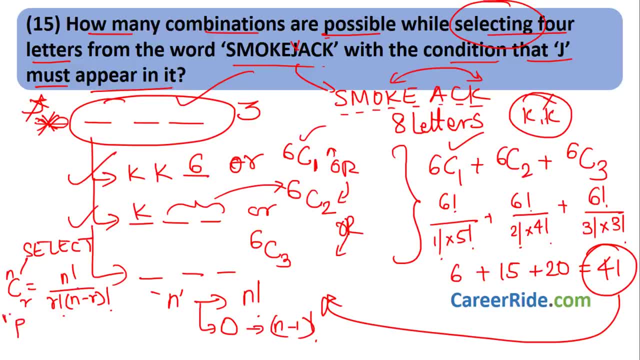 combination is select. permutation means permutation is nothing but select and arrange. So formula for selection is nothing but same as combination. What is it? r factorial into n minus r factorial multiplied by selection is done. now arrangement r. things can be arranged in r factorial ways. So this gets cancelled. So what is the formula? 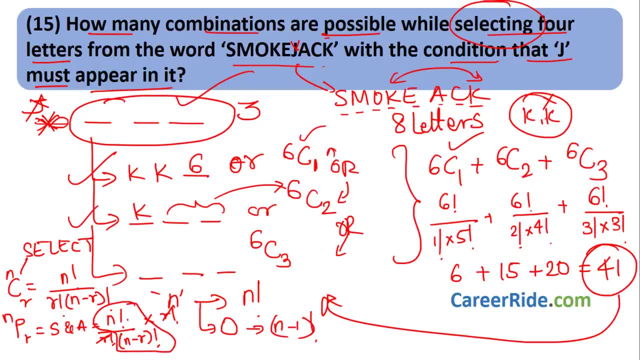 for permutation. This is the formula n factorial upon n minus r factorial. Even if you do not remember formula for permutation, it is fine. If you remember the formula for combination you can derive permutation formula, because combination is select, permutation is select And arrange very easy. just remember these things and another important thing and means. 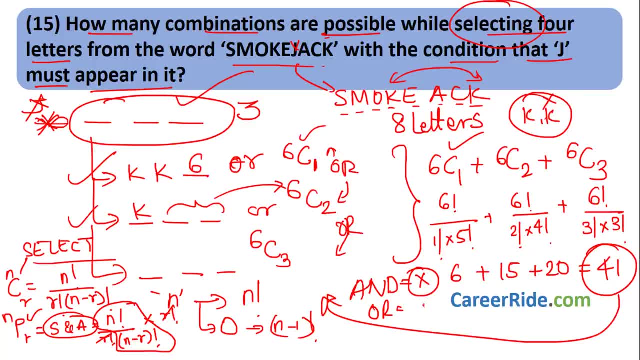 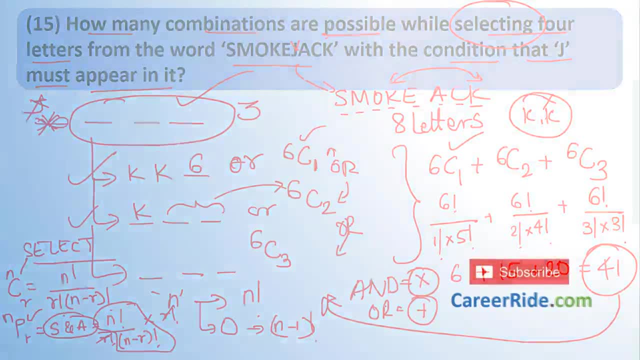 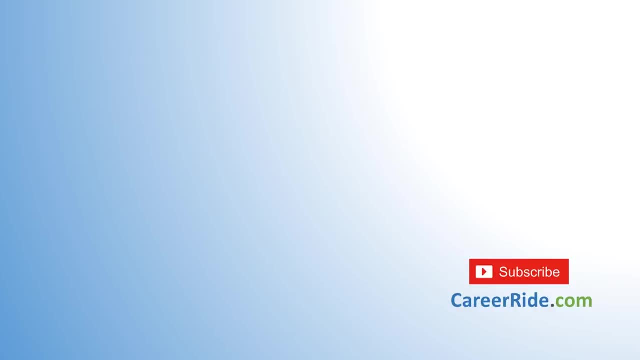 to multiply, or means to add or addition- Very easy, just remember the formulas. This is it for video on permutation and combination. I hope this helped you. If you liked it, please give it a like and do share the video with friends. Leave your comments and suggestions. 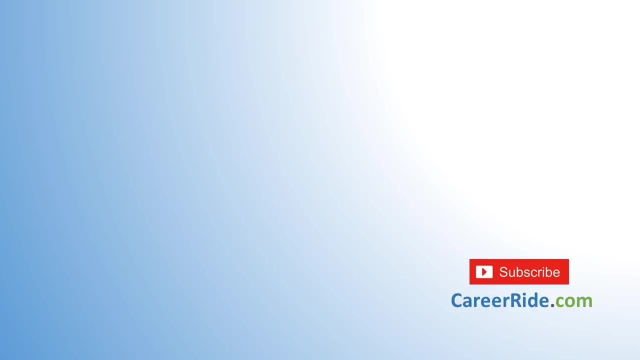 for us. You can even leave a request for video on topic of your choice. Also, do not forget to subscribe to our channel to stay updated.